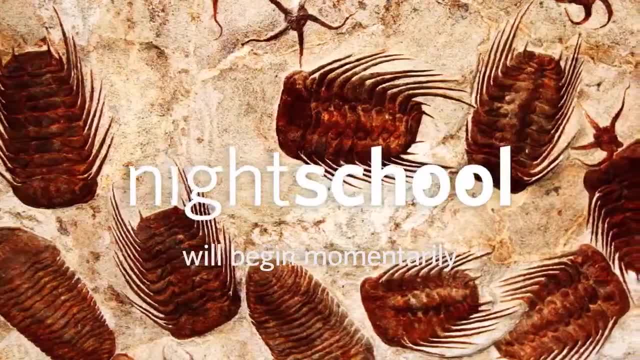 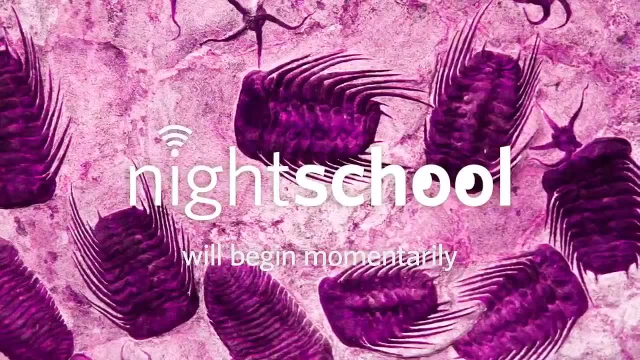 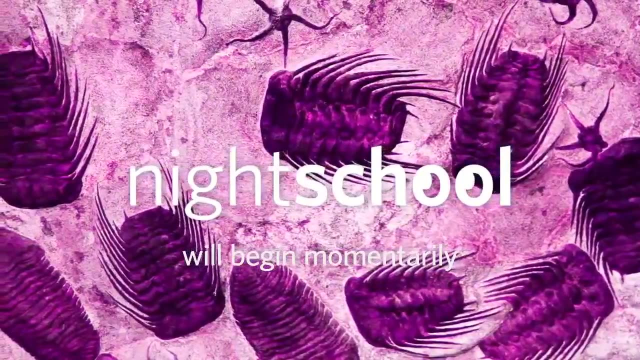 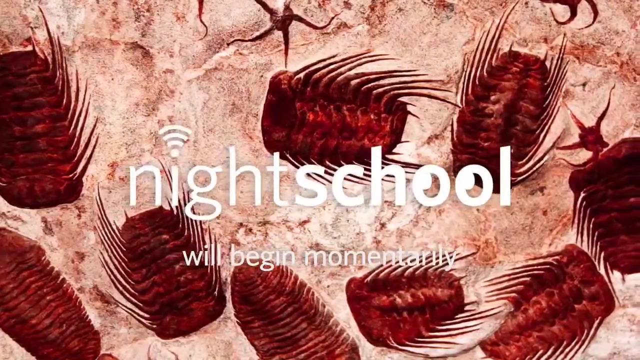 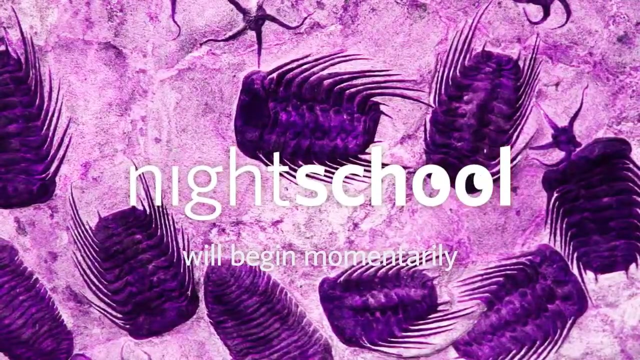 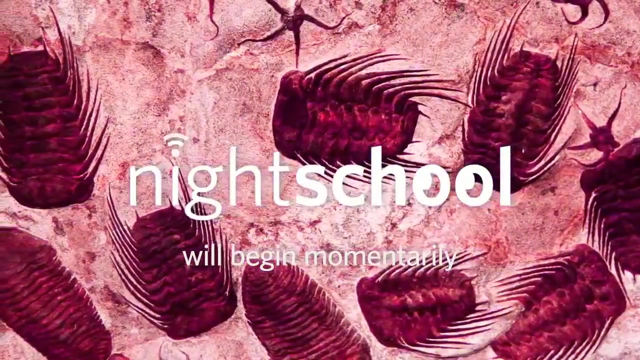 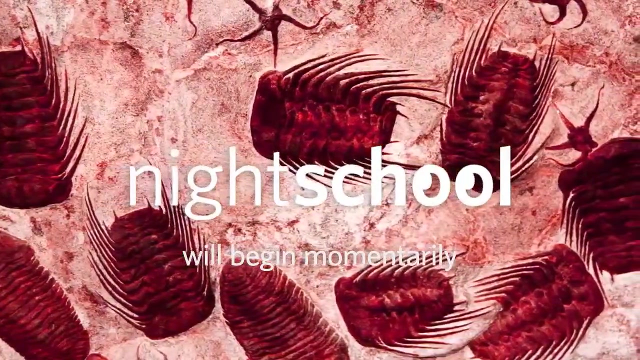 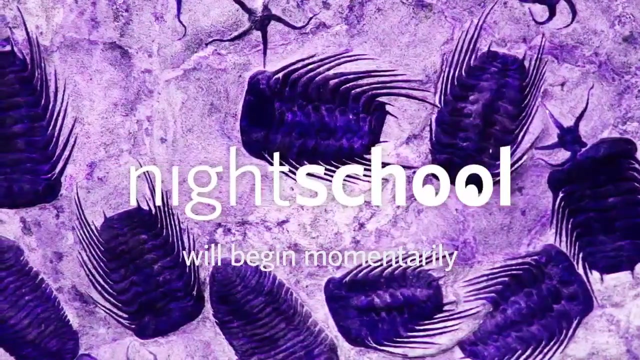 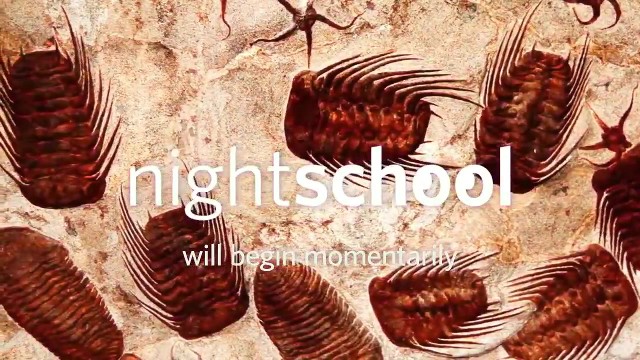 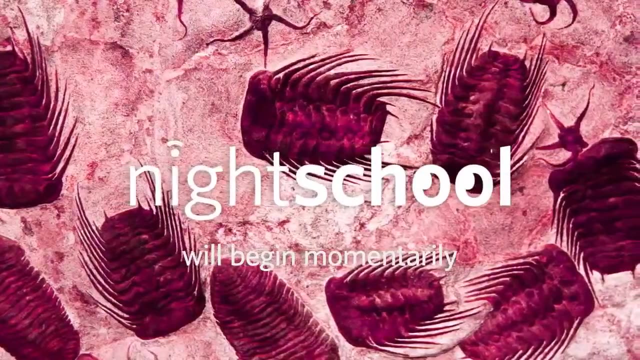 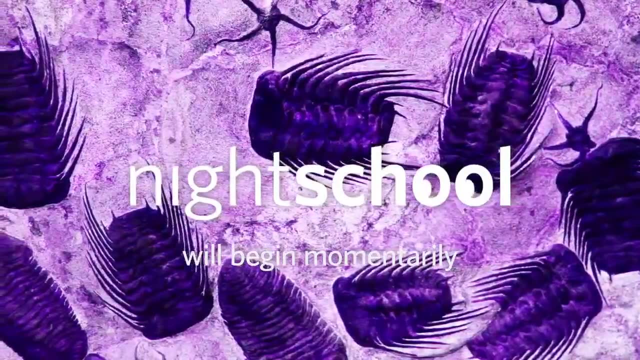 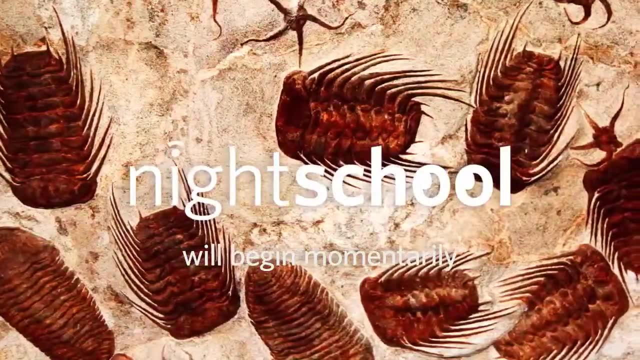 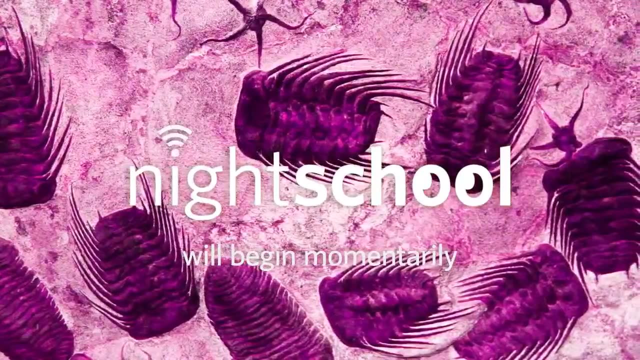 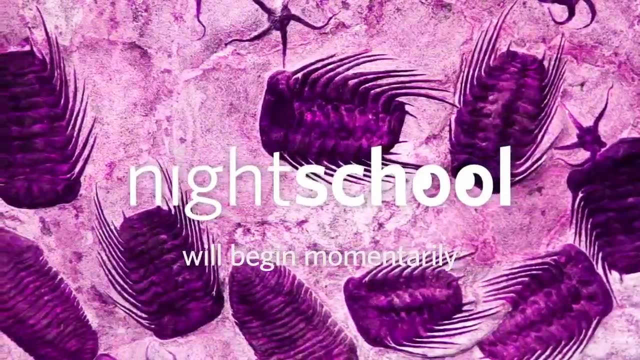 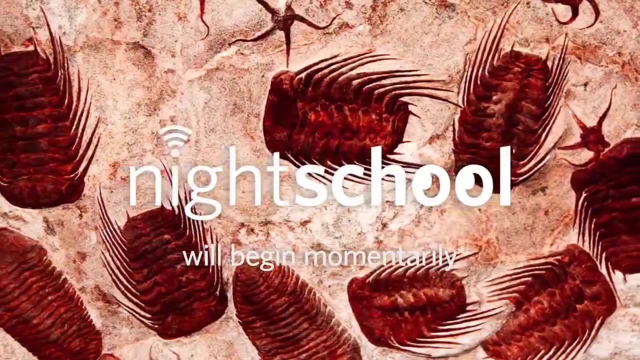 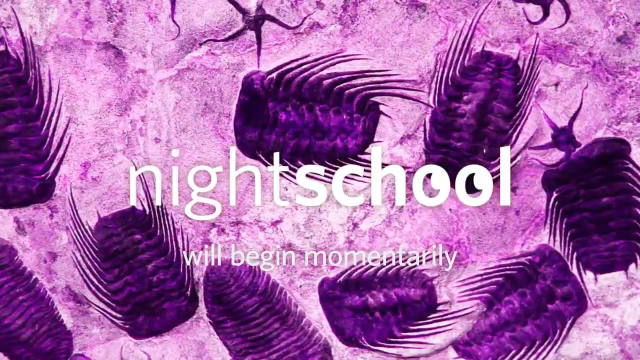 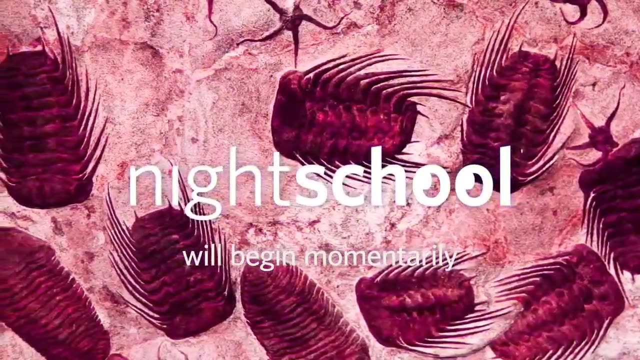 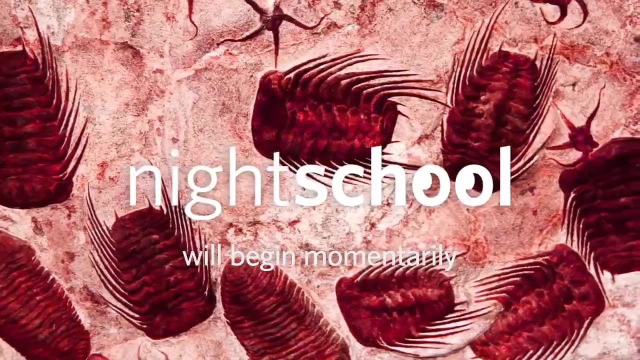 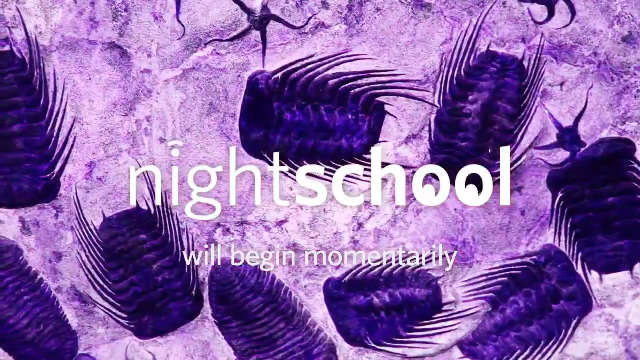 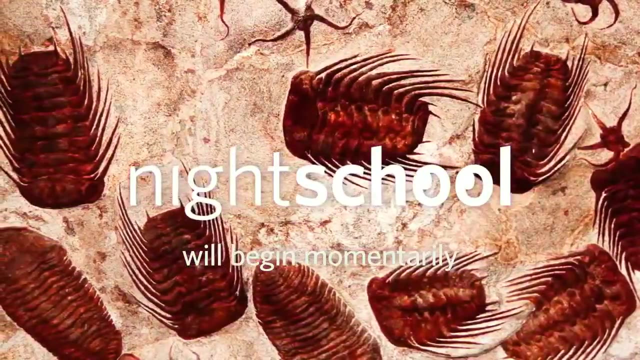 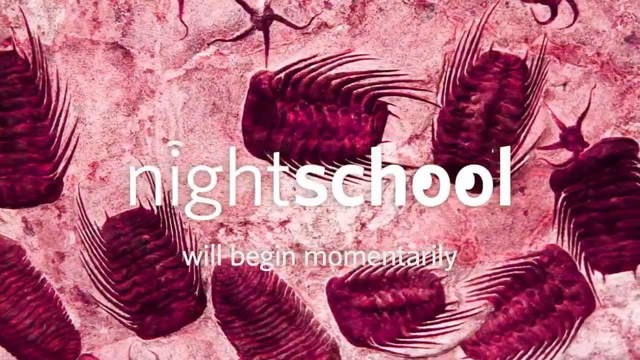 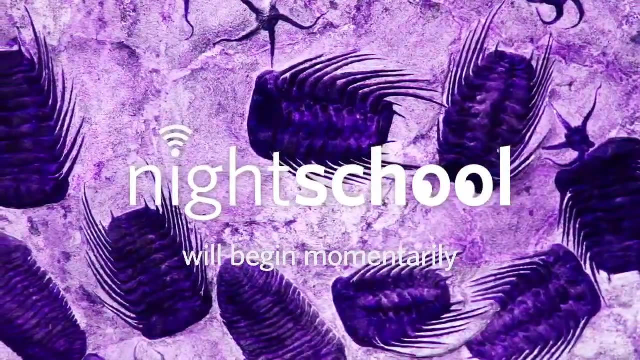 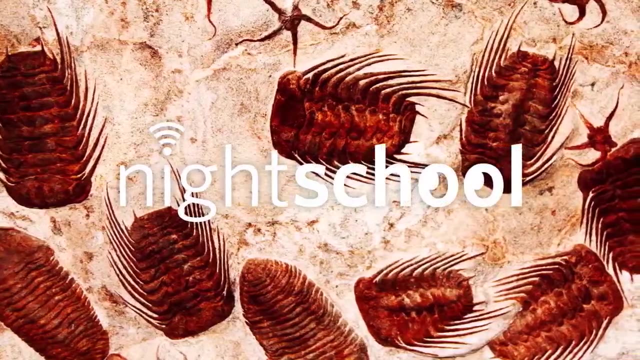 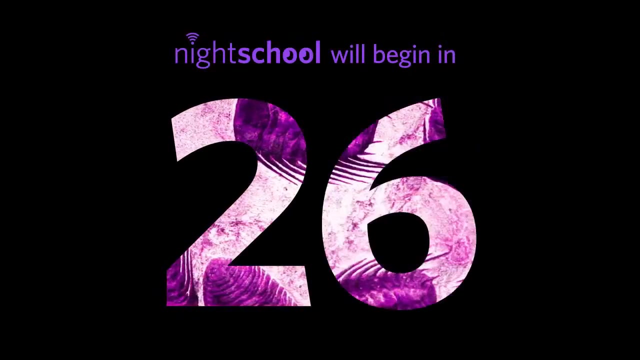 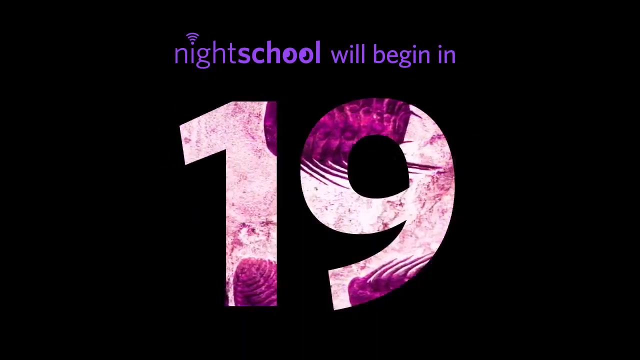 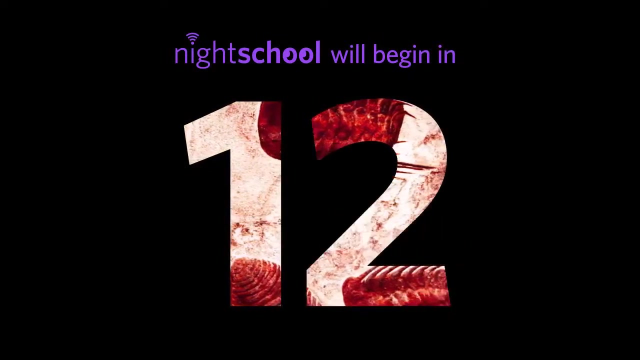 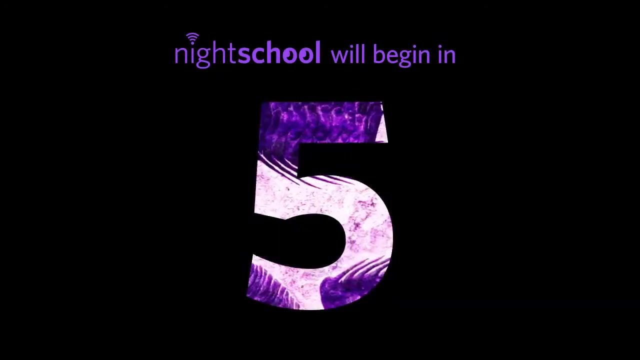 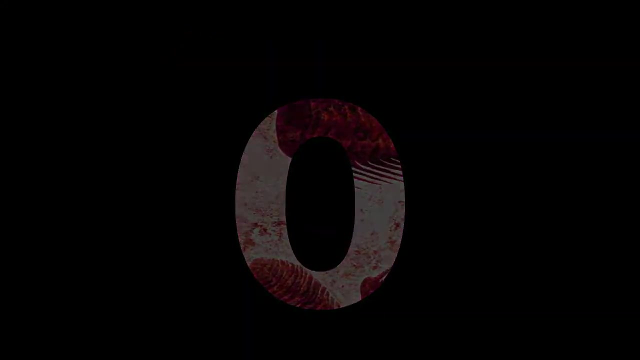 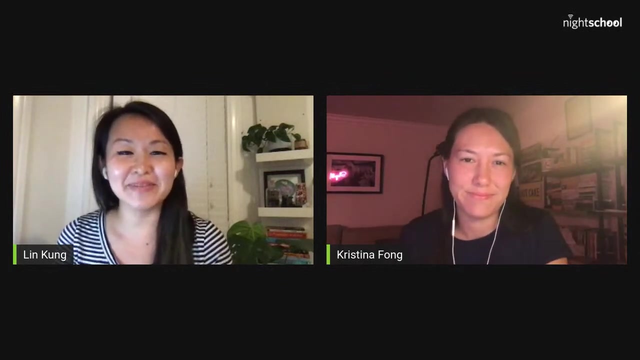 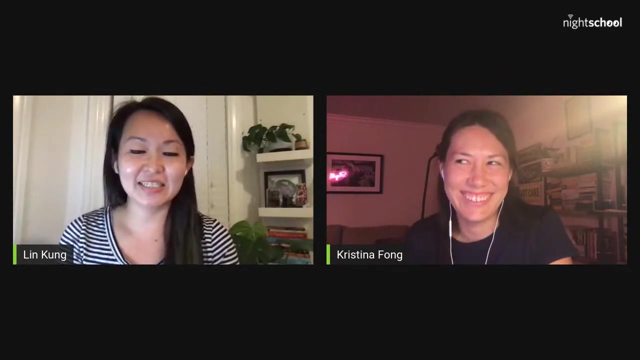 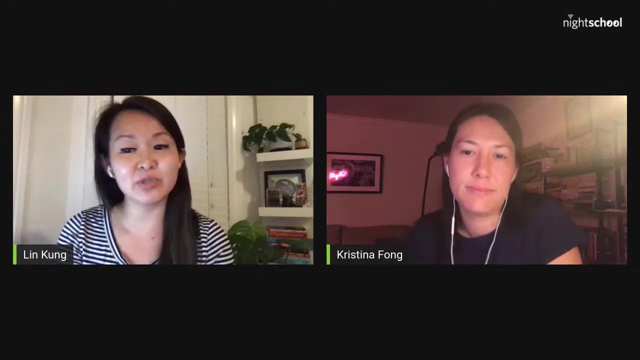 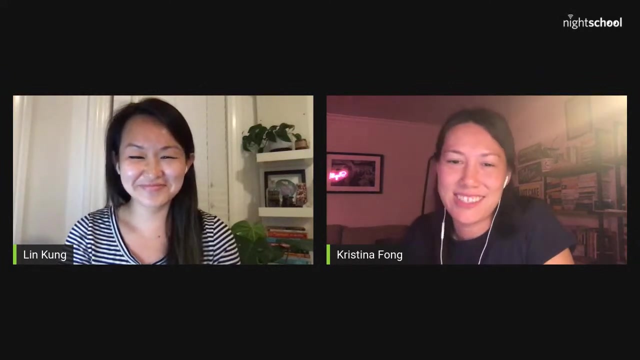 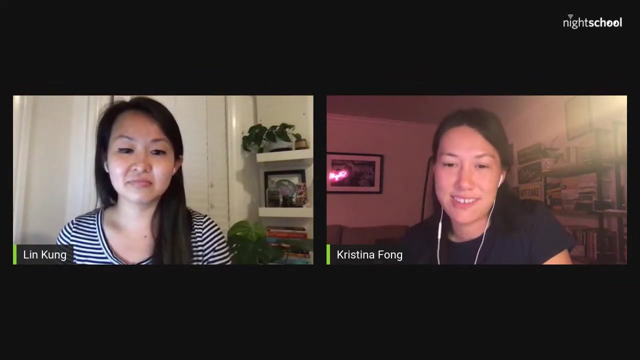 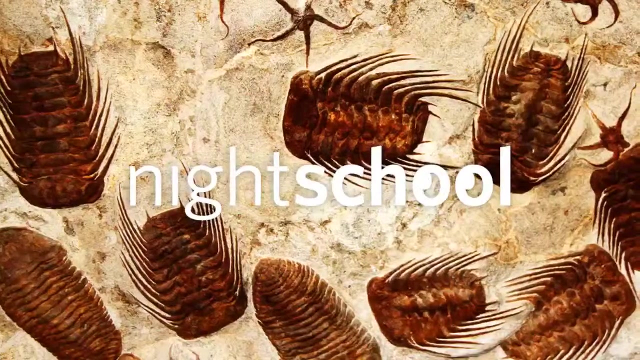 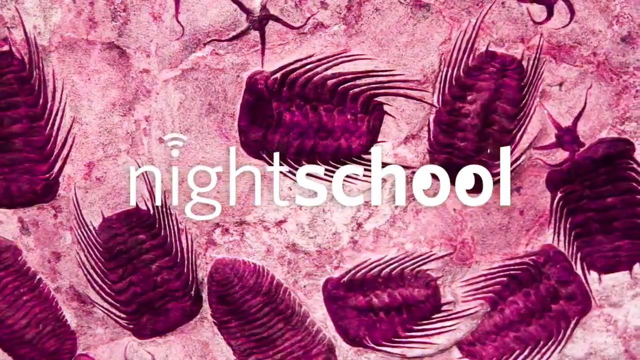 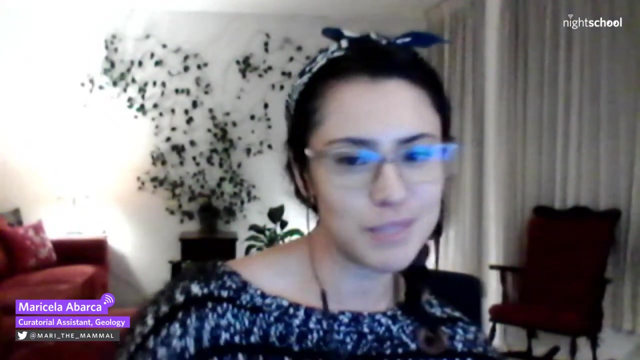 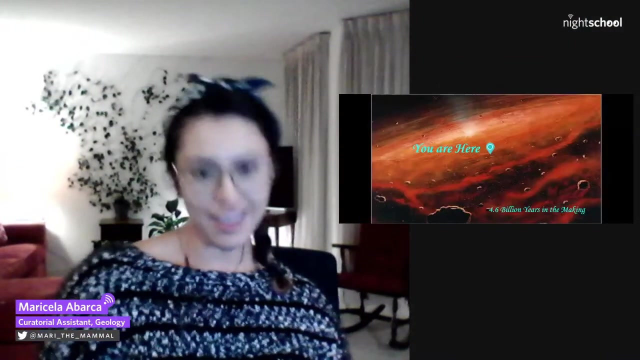 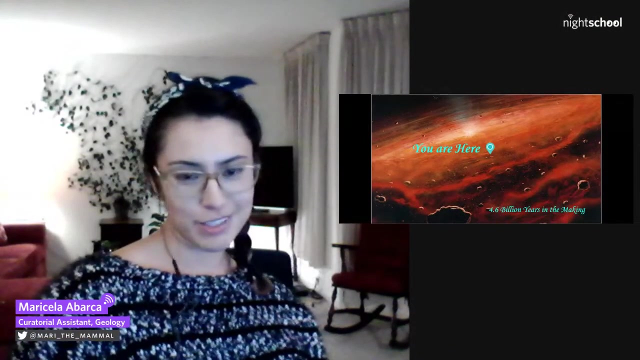 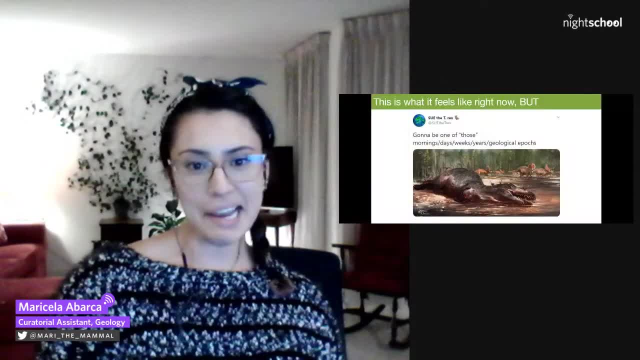 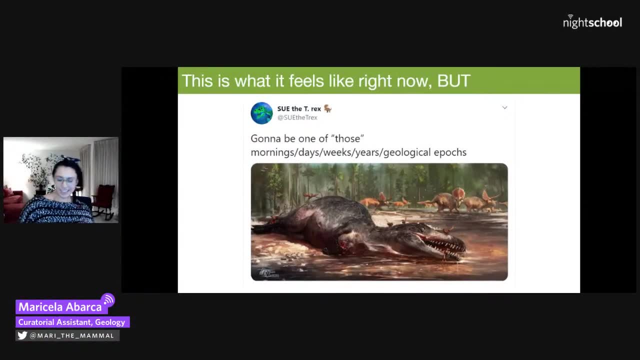 nebula to what it is now and this is kind of what it feels like right now, right, but hopefully by the end i'll convince you- maybe with a side of existentialism or, um, yeah, just general questioning of life- that still life is beautiful and it's unique that we're all here right now in this. 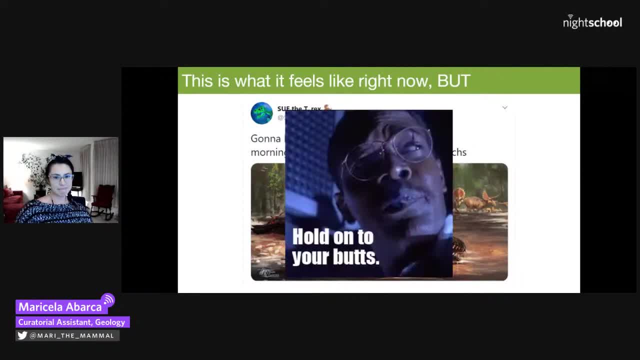 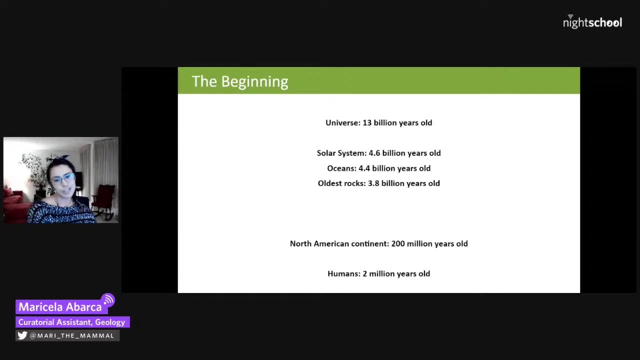 pandemic in 2020, um, but that's okay. so hold on to your butts. uh, the great words of samuel jackson jurassic park, because we're gonna do 4.6 billion years in 25 minutes. this is just like a greatest hits compilation of, uh things through my perspective that are important. 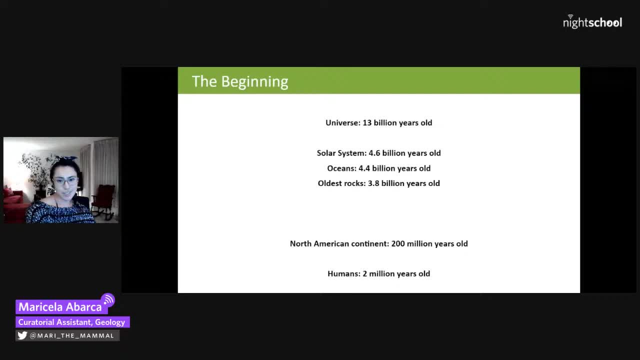 in the geologic record. so the universe at 13 billion years old. humans on the other end, 2 million years old, basically babies, and two things that are missing from this greatest hits list are sexual reproduction and the appearance of animals. so probably take a second and just think about. 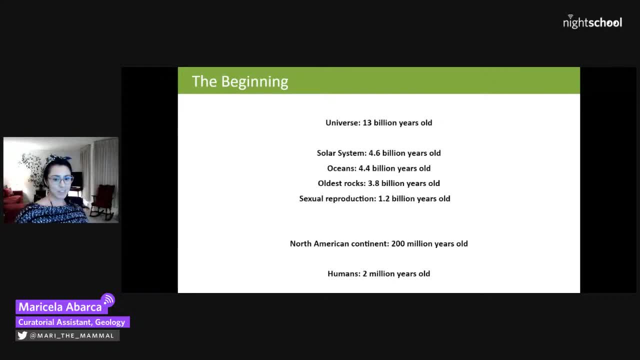 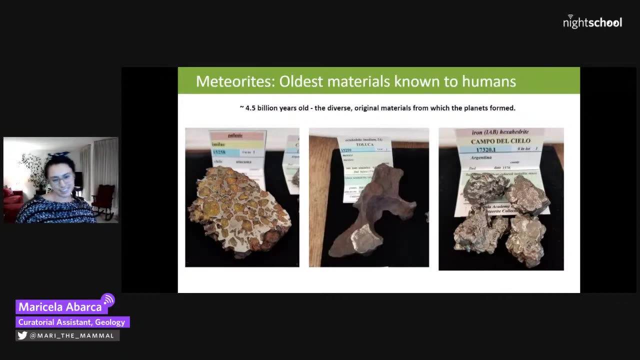 what came first? um, and if you guessed that sexual reproduction was 1.2 billion years old, good job. if you didn't, that's okay, because i'm gonna come back to this a couple more times throughout the presentation. i like to start out with meteorites, just because 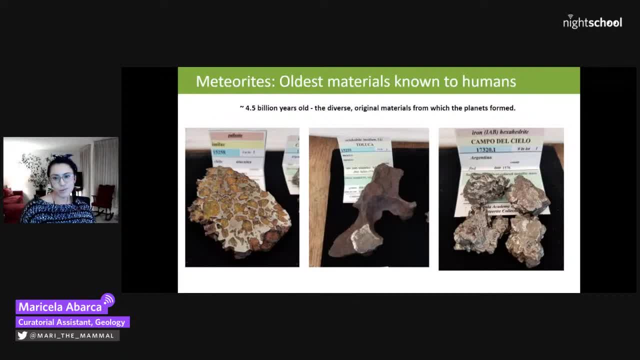 they're like these concrete, tangible things that people can interact with and see, and they're really old. um, they may not give you like a scale as to how old 4.5 billion years is or what the net worth of jeff bezos is, but these are like tangible things and these specimens are from the 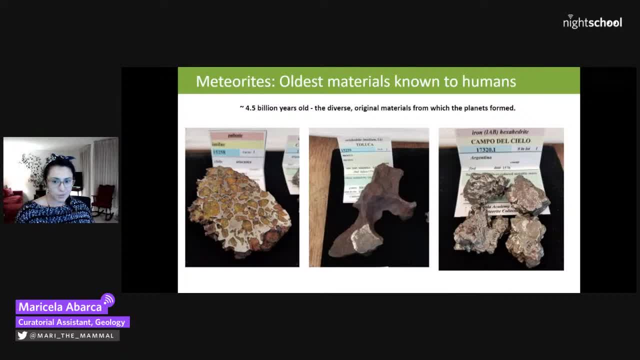 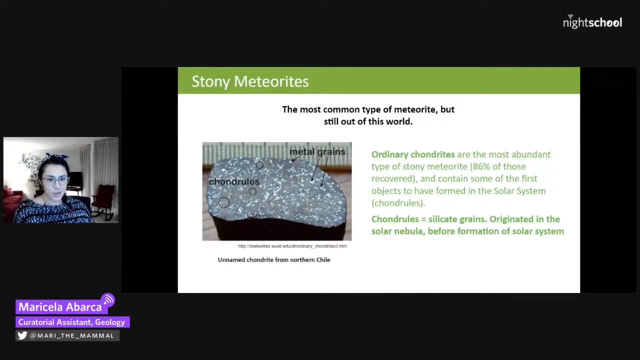 collections at the academy to the left is one of my favorite specimens. it's a palisade and it has these really beautiful olivine crystals and they're really rare and they're really sought after. and on the next slide we have these ordinary chondrites, a kind of stone meteorite. that's really. 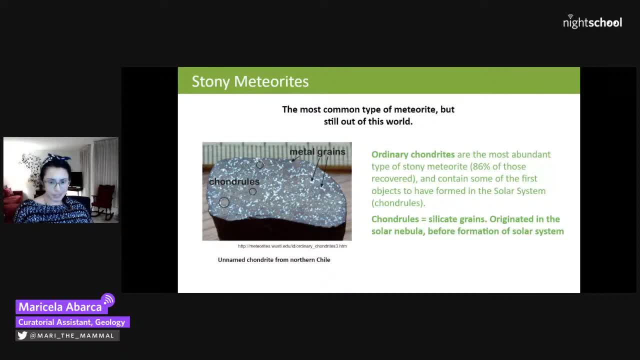 common and they may not be as beautiful as a palisade, but they're definitely really cool in that they have these little silicate grains in them called chondrules, and you can see them outlined in the image. and these little grains were present in the solar nebula, so they just remained unchanged in the specimen flew. 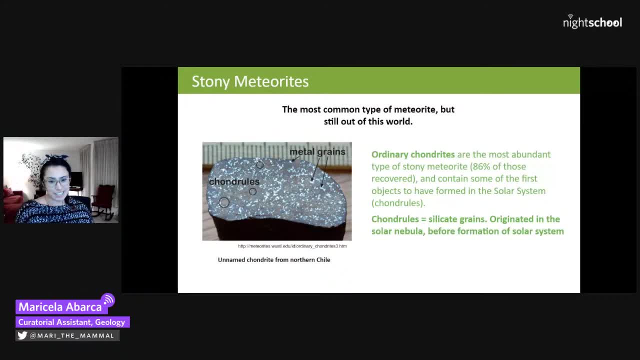 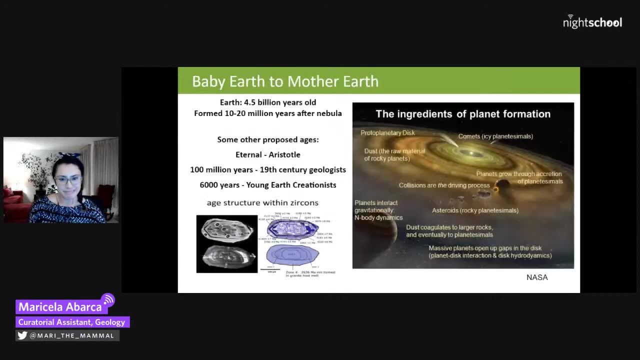 through space and ended up on earth. and now it's here in some collection, um, i'm i don't remember from where it's- um, just like a, like a really unique glimpse into that time in geologic history. piggybacking off of that, this is a representation of um, the protoplanetary disk, which is basically a. 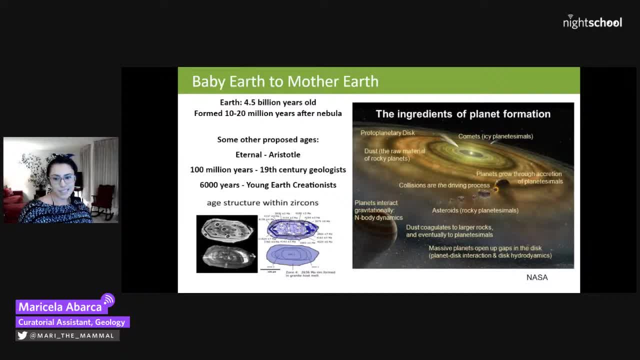 pancake of swirling cosmic dust, and somewhere in this dust was the baby earth. it had a really violent event. um, coming up, there was lots of collisions, lots of getting thrown around. um, if you can imagine rolling a ball of play-doh on the carpet, you're gonna pick up a lot of really random things. 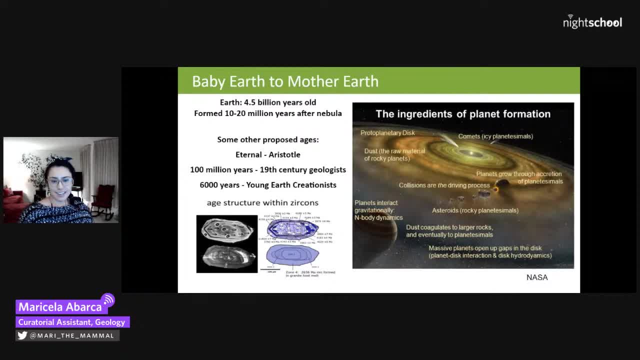 in this case, the random things are cosmic dust and we know that the earth is 4.5 billion years old because of a really um rad technique called radiometric dating, and you can use it on zircon. so part of the crystal structure of these zircon minerals is uranium and you can use the half-life of uranium to get the age of the earth. 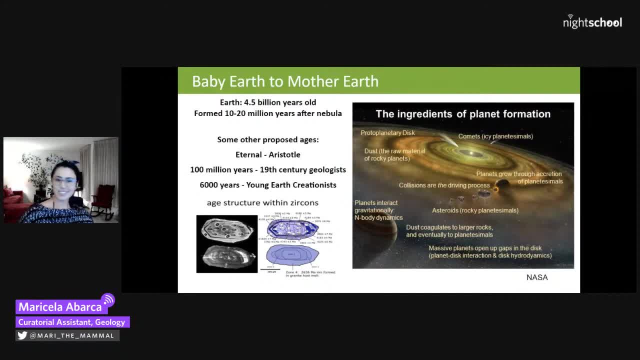 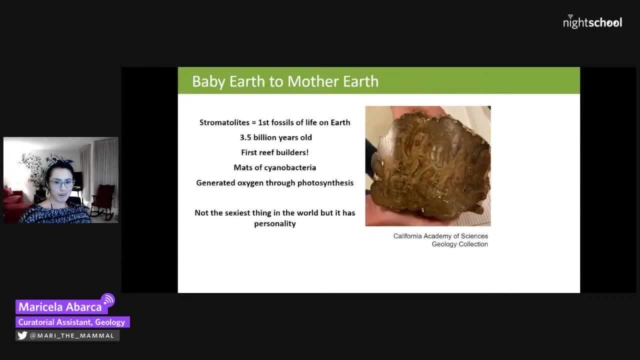 and i'm sure it's a technique that aristotle and geologists in the 19th century would have drooled over. right, so um, earth became a mother sometime around 3.5 billion years ago, and its first poster child were the stromatolites. there was earth before. 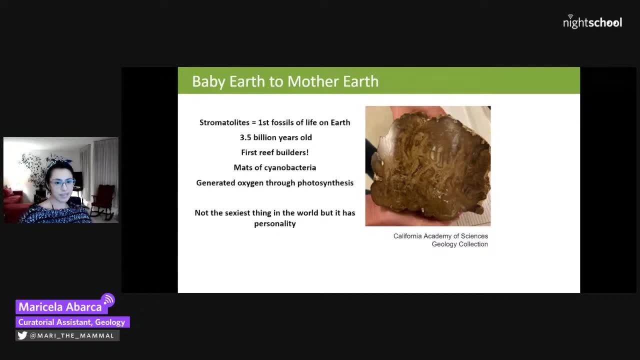 there was life on earth before the stromatolites- probably bacteria, but um, these stromatolites are the first like undisputed fossil evidence of life on earth, and if you don't know what that is, it's okay. they're just photos photosynthesizing bacteria. they're pulling carbon dioxide. 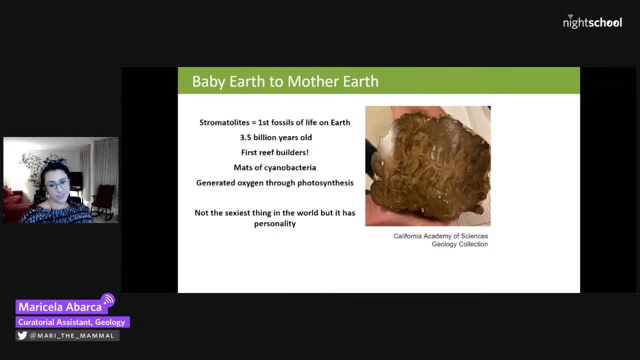 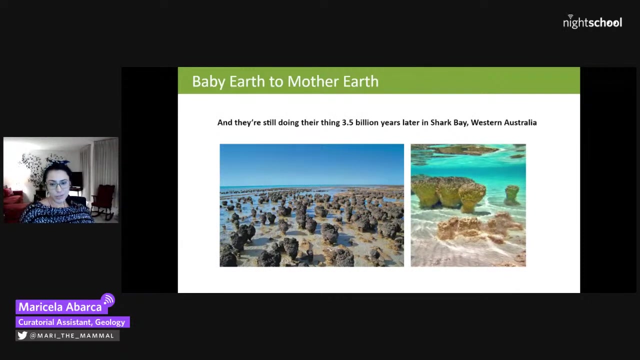 of the water out of the atmosphere and generating oxygen. so this specimen from the collection might not look like much, but don't judge a book by its cover, because without it we wouldn't be the oxygen consuming life forms that we are today without them. and they're still around today in western australia. they're really rare now, though. um, they're only found in 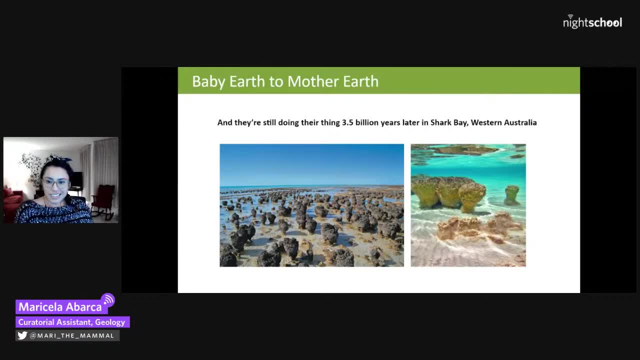 shallow waters, so poor went out for stromatolites. and also shout out to australia, um, because, aside from having tons of animals that will kill you and are really terrifying, um, it's also home to a lot of really cool geologic formations, like stromatolites and. 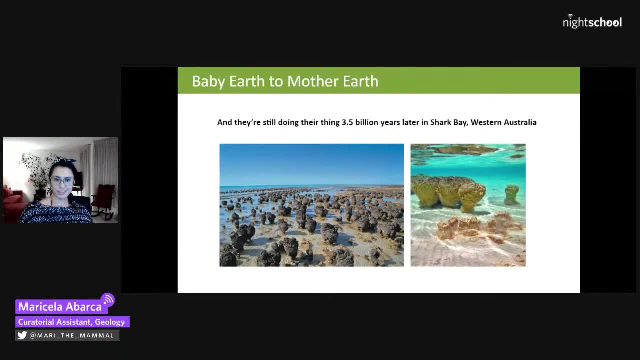 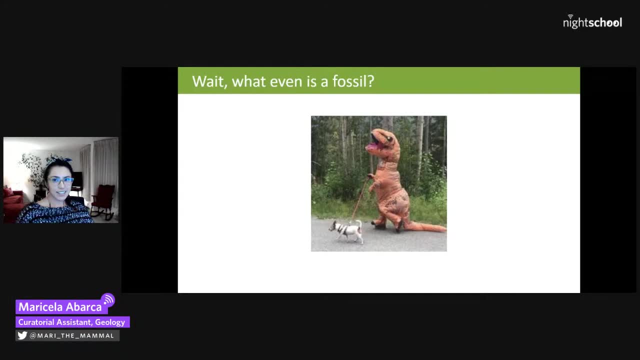 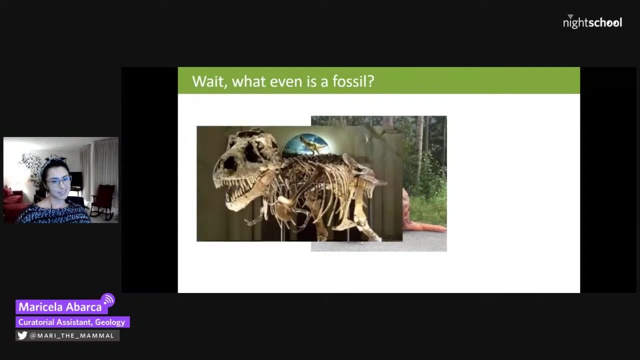 like the zircon. that dated the earth back to 4.5 billion years, right? so stromatolite is a fossil, and usually at nightlife. it's kind of fun to talk to people about what a fossil is, and it's not just dinosaurs, they're really familiar. i'm not going to spend a lot of time on it. 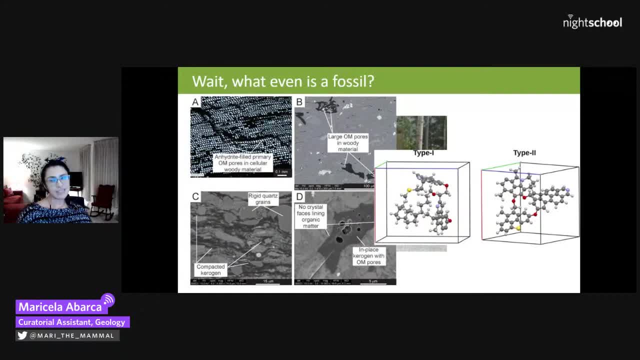 there are definitely other kinds of fossils and basically what it boils down to is a fossil is anything of evidence of past life on earth, and what you're looking at now is what we call chemical fossil, and the specific unfortunate thing is um that those fossils are really calm and they're not going to die long, no matter when we look at it, um, or if we do see them being put in a place where they could be aand they're really stable in the ocean, and then they would be better than生 others by falling. and there are lots of fossils that are still found in the years, of course, um木 margins that are 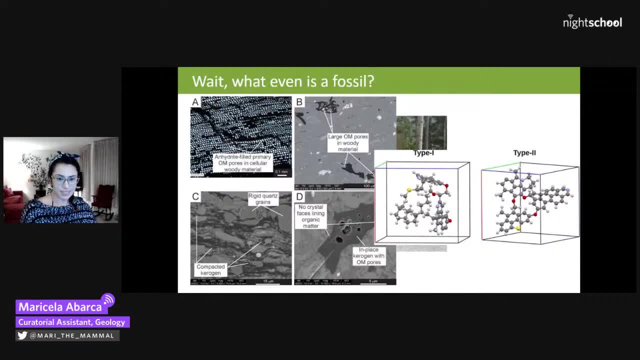 type is a kerogen, which is just a fancy word for a bunch of carbon and hydrogen that's linked together. And carbon and hydrogen linked together is like a really telltale signature of previous life, And it's usually plants- In this case it's a piece of wood- And these were taken with a. 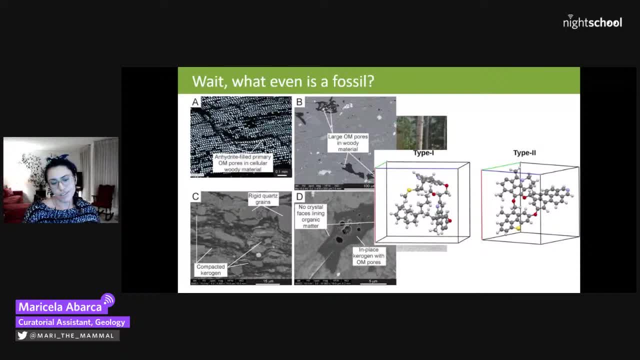 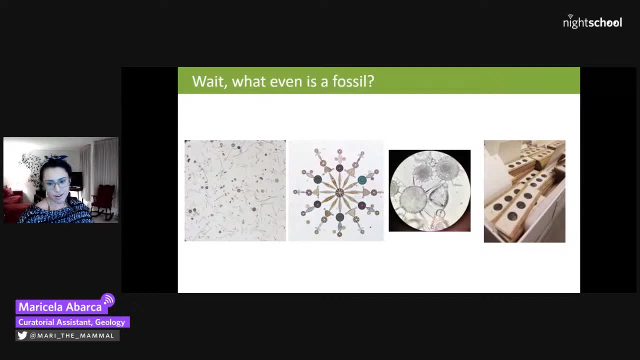 scanning electron microscope And oil. geologists really fawn over kerogen because it's a precursor to fossil fuel deposits. So other really tiny fossils that you need a microscope to look at are the microfossils To the far left is a strew of diatoms, So somebody just spread them. 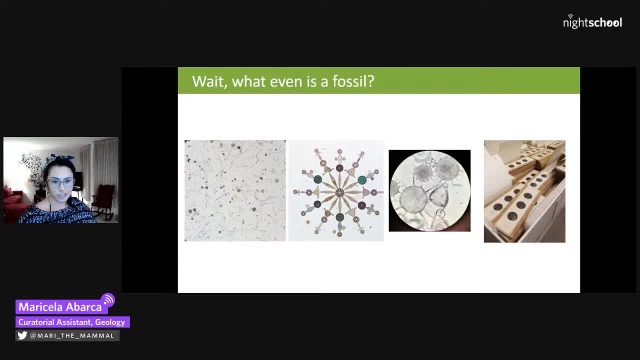 out on a microscope slide In the 1900s- And I took this photo of them a couple years ago- And if you're really bored, in the Victorian era a really popular thing to do was arrange them on slides and make these little. 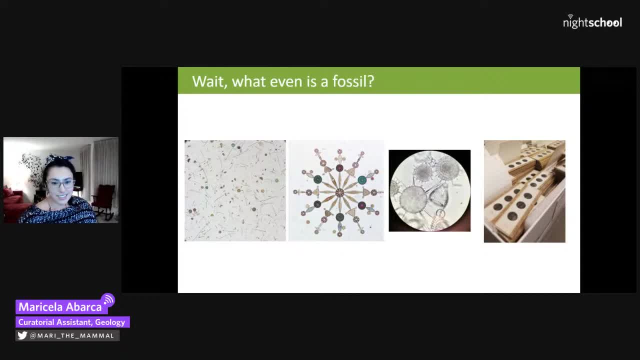 artistic patterns, And this collection is also- there's like a little collection of artistically arranged diatoms in our collections at the Academy as well, And if you don't know what a diatom is, it's basically the modern analog of what a stromatolite was. They're the primary producers in marine environments now. 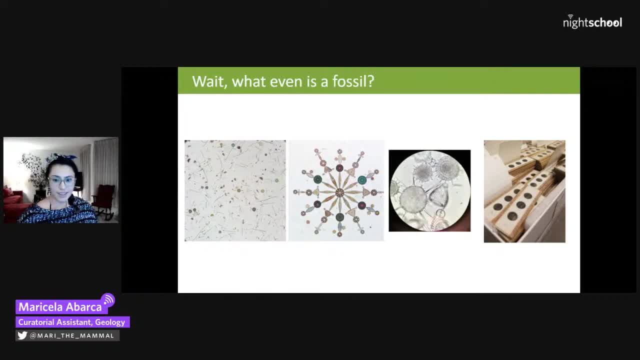 They generate a lot of oxygen. So to the right of the arranged diatom slide is a microscope photo that I took of radiolarians, Also another kind of little microfossil with really cool structures, And then to the right of that are well slides And you might be able to make out like these really. 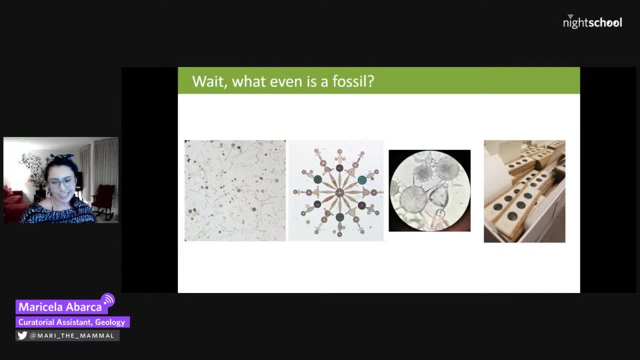 tiny grain of sand looking things in the middle of the wells and in there are these other moon microfossils called 4AMS, And we actually have a grant from the National Science Foundation right now to like digitize this collection of 4AMS In order to reconstruct this collection of layers. 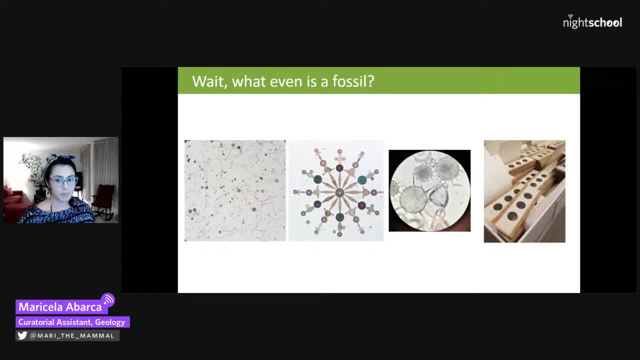 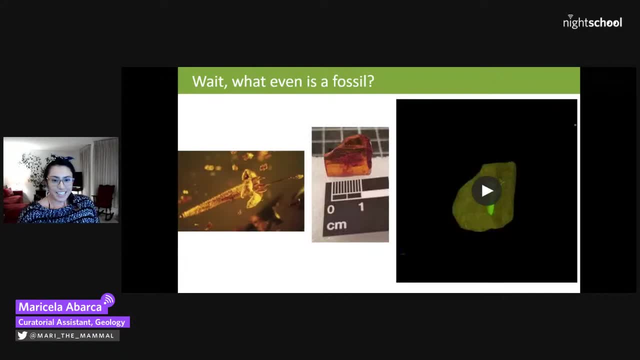 So that's another thing that you can find further down the line towards us, In the inнаяwater'sorymf, outside of the tipos, you'll find various Congress times or major construct like paleoclimates. So next up on what is a fossil, we have amber of Jurassic Park fame. 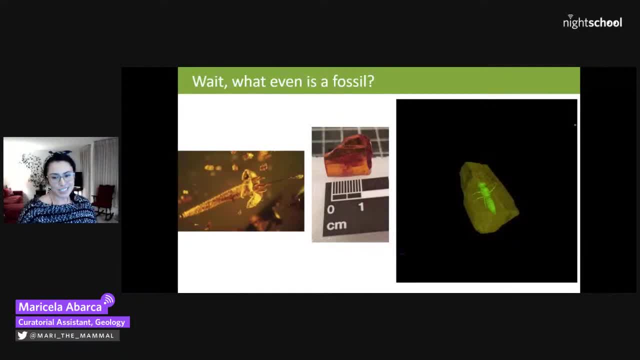 Amber is really cool. It's really pretty, Everybody loves it. It's really sexy, But it's also they can tell really cool stories. So the amber specimen on the left is of an asteroid flower, And if you don't know what an asteroid flower is, you can think it, for 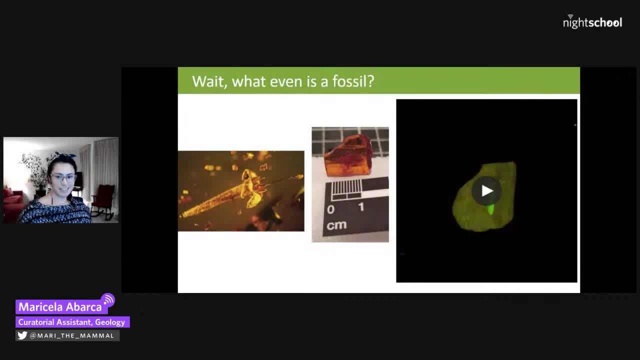 things like coffee potatoes, tomatoes, sunflowers- It's this really big family of flowering plants And this specimen was trapped in amber 20 million years ago And it's the first asteroid flower fossil that's been found And it's in our collections at the Academy And it was described. 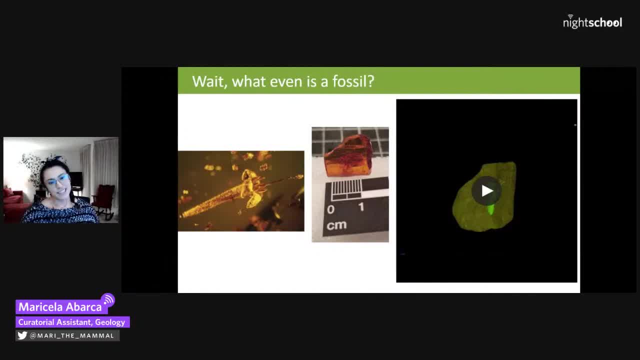 by a man named George George Pointer, who is like the Elvis of studying stuff trapped in amber, And it was through him that Michael Crichton got the idea that you could extract dinosaur DNA out of the stuff trapped in amber, Since then disproved, but like that's where we got the 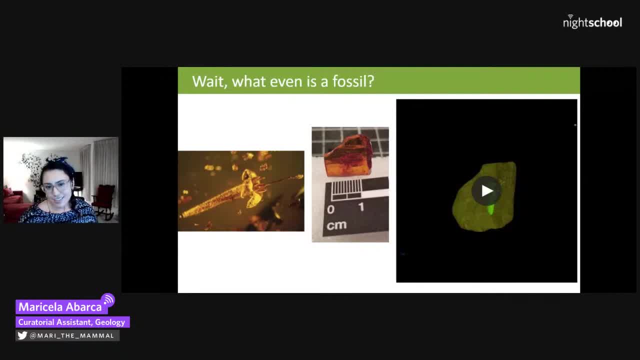 idea. And next to that is a little piece of amber, also in our collection, And there's a wasp In the middle And from the photo you can't really tell. you can't really make out a lot of the detail, But this is a CT scan that I did of this piece of amber a couple of years. 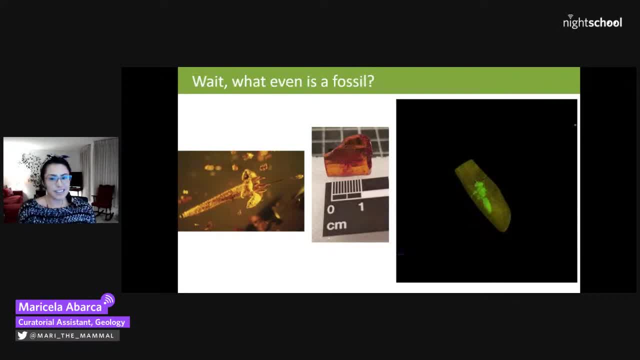 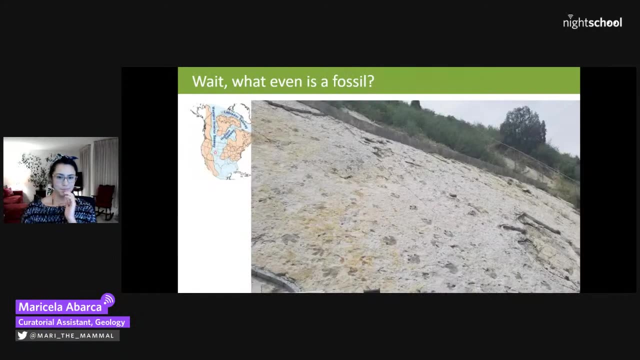 ago And it's really cool piece of technology that we have now and it allows you to do measurements on what's trapped inside the amber and like study its anatomy without destroying the specimen Right. so other kinds of fossils We went over like body fossils. This is more characteristic. 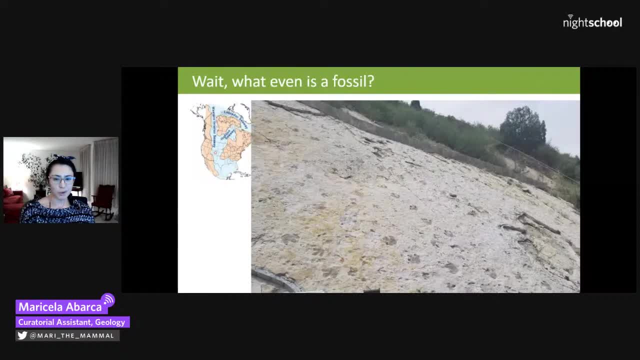 of trace fossils. So things like footprints, things like worm burrows, just signs of life, And these are from a place called Dino Ridge, just out of Denver, back in the Cretaceous, when Denver, Okay, Had a coastline because of the Western Interior Seaway. 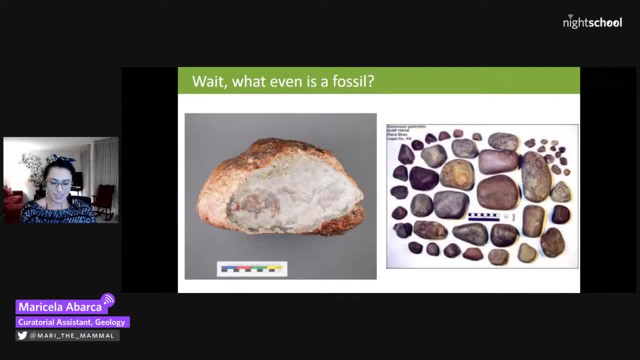 And these are more fossils, believe it or not. and you can probably say, Maricela, I don't believe you, They just look like rocks And I wouldn't blame you because they do just look like rocks. But the one on the left is a coprolite, which is a fancy word for fossilized. 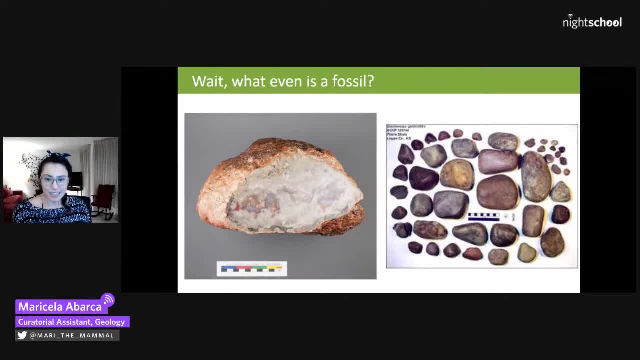 poop, And the ones on the right are examples of gastroliths, Gastro from stomach. And if you still don't believe me and you're like, no, those are just rocks- like I'm sure that you're a crazy person, I would show you this really special fossil where the gastroliths were actually. 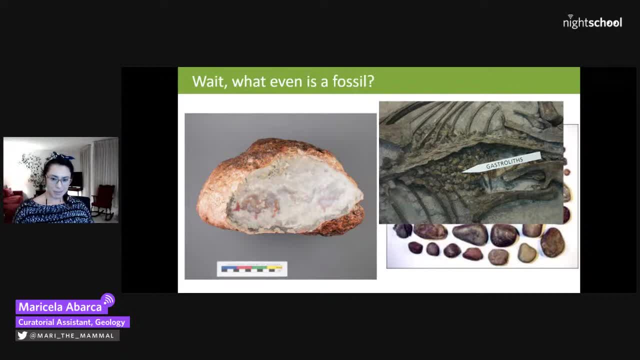 found inside the body cavity, And they're found there because birds and reptiles would swallow these rocks to eat. And they're found there because birds and reptiles would swallow these rocks to eat. And they're found there because birds and reptiles would swallow these rocks to eat. 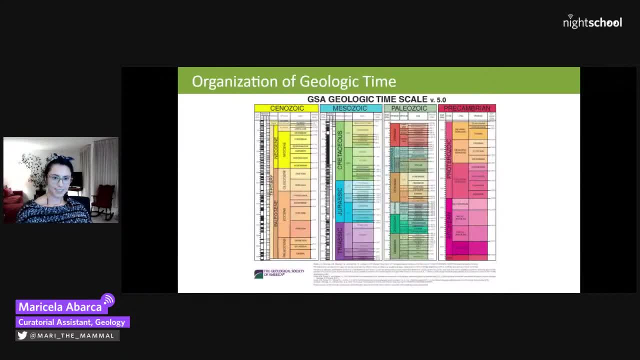 digestion Right. so that was in no means like an exhausted list of kinds of fossils. I could probably do like a whole hour on just kinds of fossils by themselves. but we're going to change gears a little bit and kind of explore how humans have broken up geologic time And we're going to 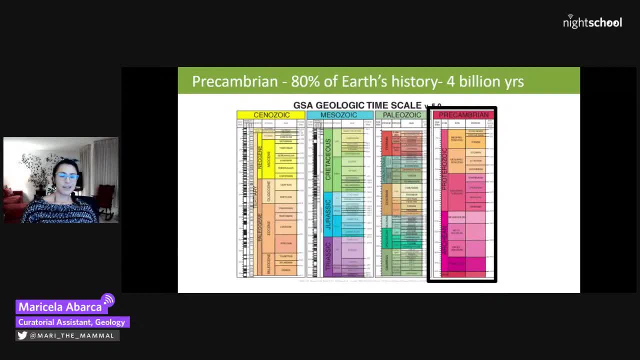 start from the beginning. In the Precambrian. this skinny yellow column represents 80% of Earth's history: 4 billion years. There wasn't a lot going on in terms of life on Earth at this time, but there was a lot of important stage setting processes that occurred. 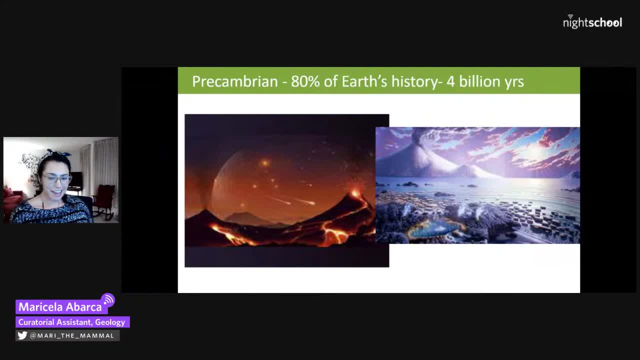 And it began looking like on the left really scary, terrifying molten lava situation. Some scientists estimate that there were 22,000 meteorite impacts during this time when the Earth was spinning around in that protoplanetary disk after the nebula. 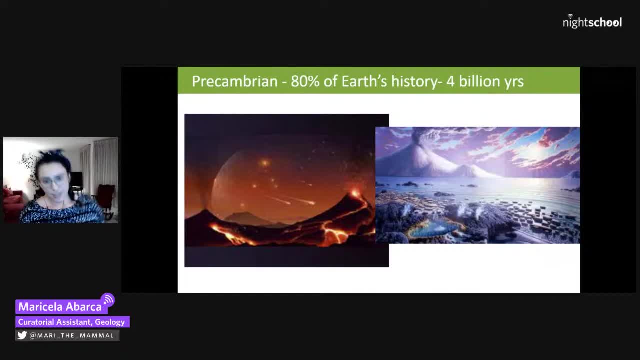 And it was probably one of those impacts that gave us the moon. But by the end of the Precambrian everything kind of chilled out. The Earth cooled off. You got the formation of oceans, the beginning of plate tectonics and the stromatolites You can. 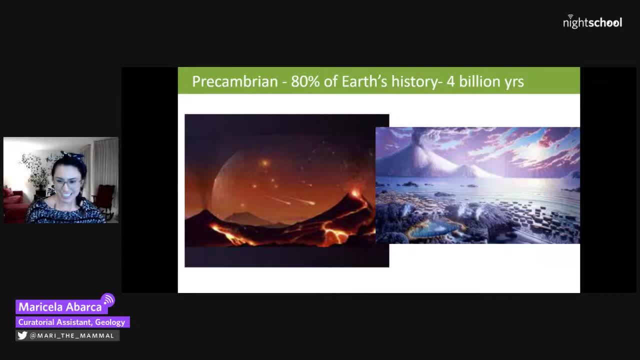 kind of like make out little stromatolite reefs on the right And I promised we would come back to sexual reproduction. Somewhere in these waters is red algae, And red algae we know um reproduces sexually, So 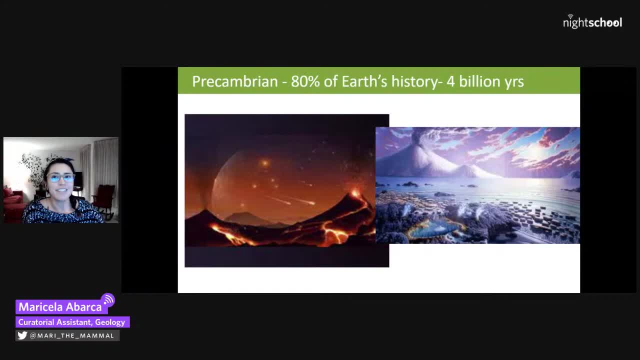 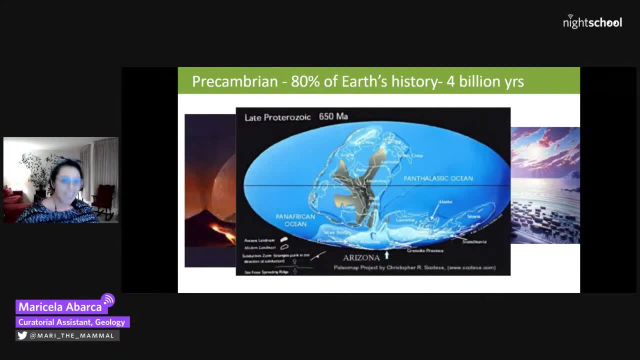 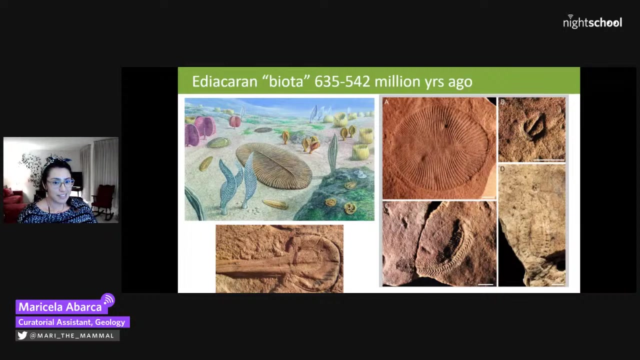 um, this is a depiction of like of sexual reproduction 1.2 billion years ago And at the end of the Precambrian. this is kind of what life forms were working with in terms of land mass, And it was the home for the Ediacaran biota. Biota in quotes: 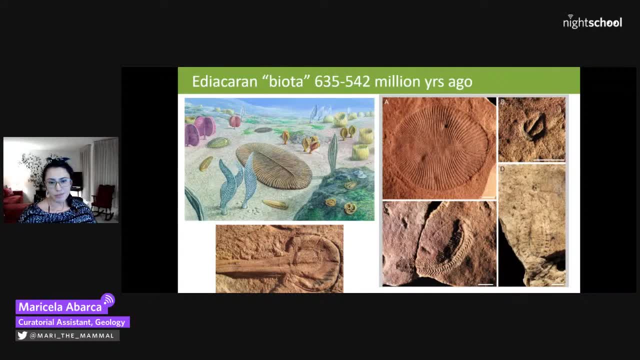 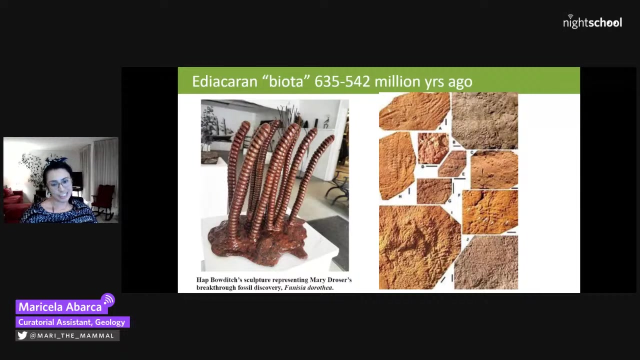 was something that was extremely important to human formation. So this is just the fine detail And this is a picture of the re-اطation of a human being, And the idea is that if one is living in a place that has an event and there is a process of doing something to the earth, the earth will come back to us and 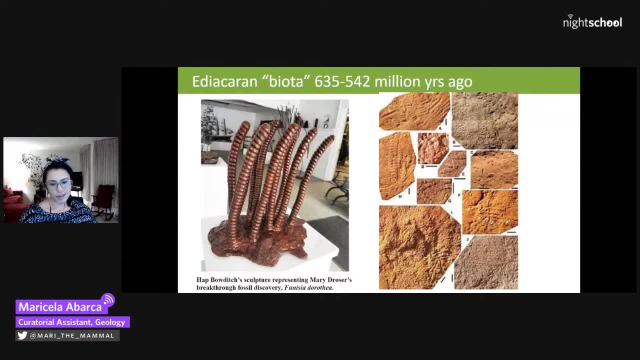 take us back to our present age, And that is what we're really trying to do, which is to make sure that to the Right, which were published by Mary Drozer at UC Riverside, And, just like staying on the sexual reproduction train, she successfully argued in that paper that they also underwent. 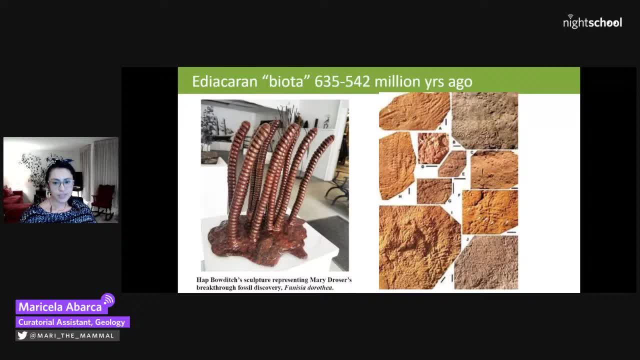 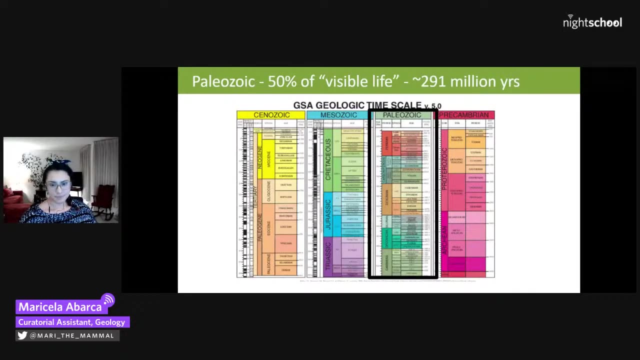 sexual reproduction. So it's like the first accepted evidence of sexual reproduction in animals about 600 million years ago. So now we're going into the Paleozoic, And the Paleozoic is kind of like a very romantic geologic era to me because it's bookended by two really. 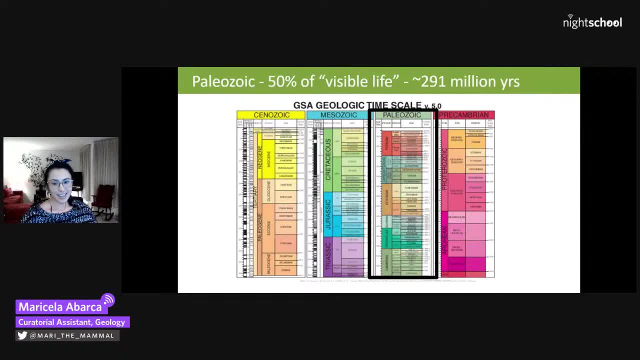 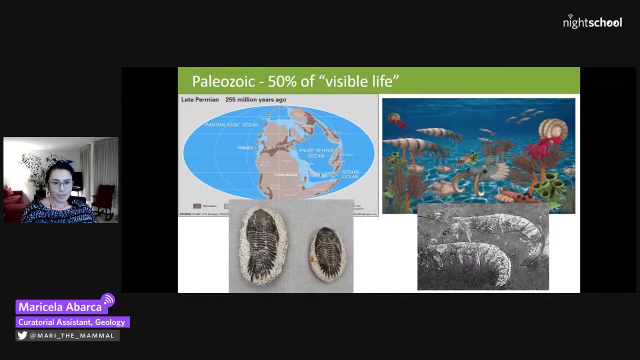 major, totally opposite phenomenon, And it kicked off with the Cambrian explosion, this really vast explosion of life On Earth, different life forms, And it ended with the biggest mass extinction in Earth's history, where over 90% of species just said goodnight forever. So, yeah, towards the end. 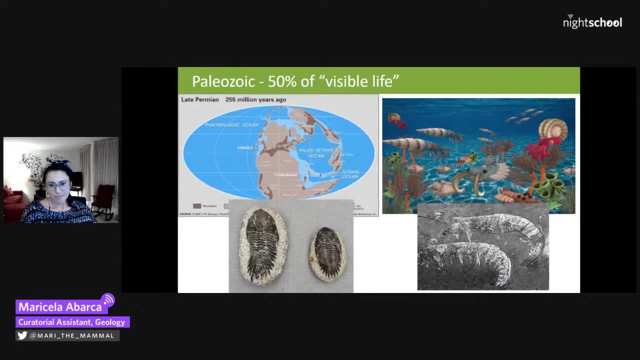 of the Paleozoic we have our friend Pangea. To the right is an artistic depiction of a little animal named the Anomalocaris. I don't know if you can see the pointer, but this is a fossil of Anomalocaris, a little shrimp-looking thing, And this is the drawing of Anomalocaris. 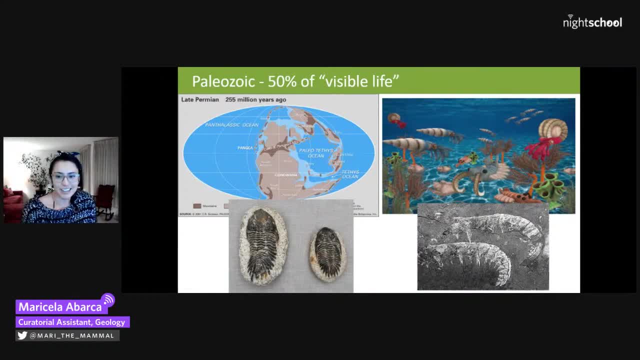 And if you were Anomalocaris in the Paleozoic ocean? like you were the apex predator. You got to like mob around in this like pink tutu thing, but you were it. Everybody was scared of you and you were like the first kind of predator on the scene. And if you were a trilobite? 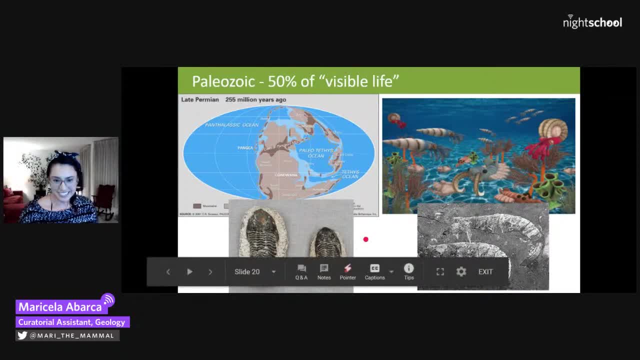 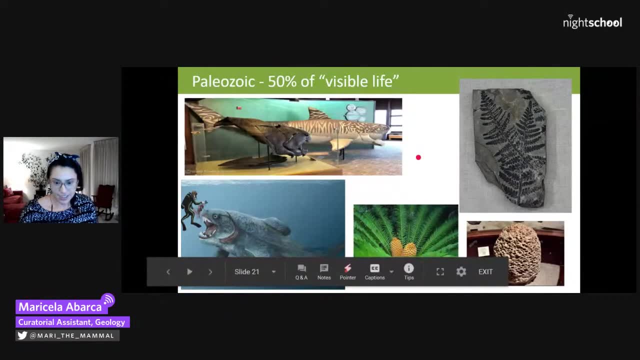 you were just a bottom toe feeder. They're basically the cockroaches of the ocean. So other things that were kicking around in the Paleozoic to the right are plant fossils. So I didn't even mention plant fossils in those other slides. but we have a fern and then a large cycad seed on the bottom right And cycads are. 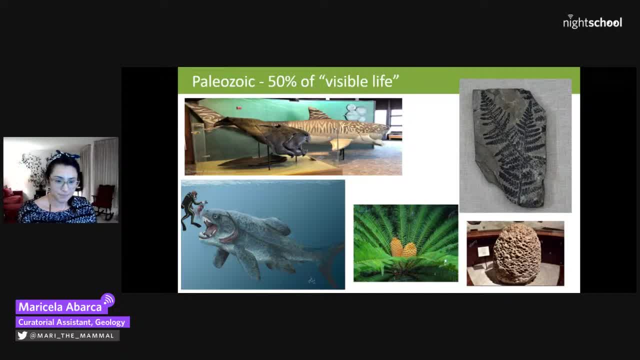 still around today as well, but they're endangered. And the really horrifying thing on the left is Dunkleosteus, which was a really crazy looking armored fish, And there's actually fossils of Dunkleosteus ancestors that have embryos in them, So that was actually evidence for internal 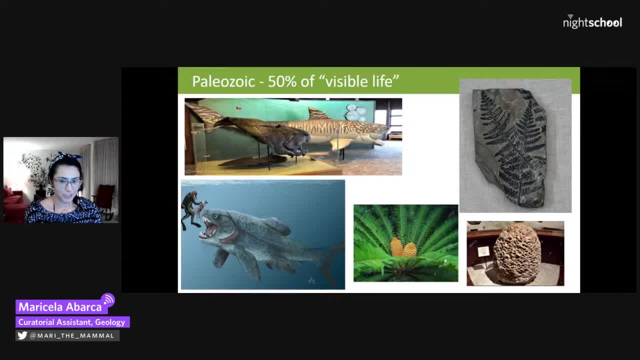 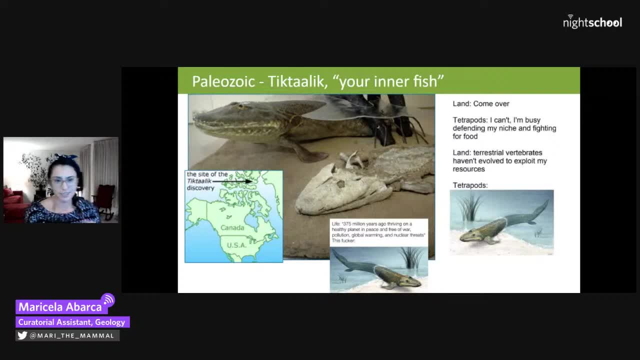 insemination in vertebrates. So that's like the first evidence of that. And also towards the end of the Paleozoic we have Tiktaalik, made famous by Neil Shubin who discovered it in Arctic Canada. He did a PBS series. 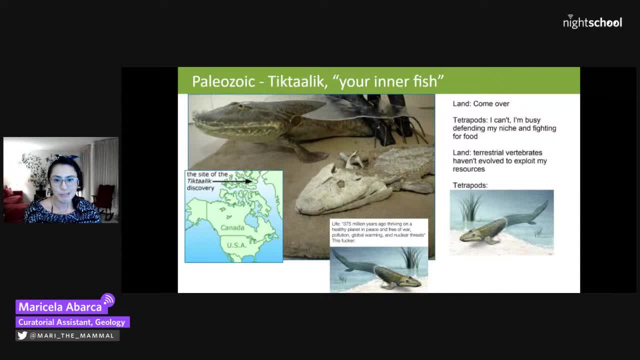 called Your Inner Fish, which is way more thorough and informed history of life on Earth And I would highly recommend it. And if you know me In real life, I like live for memes, so especially science memes. So these are just some I found of Tiktaalik. 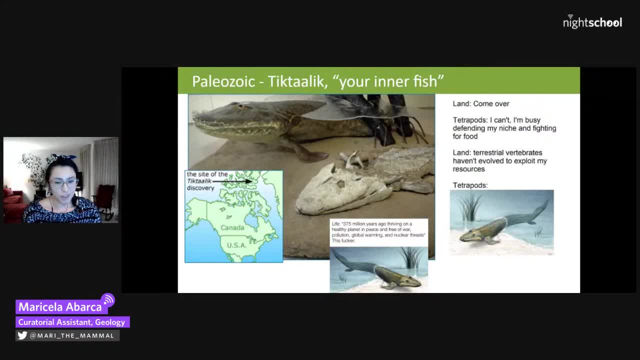 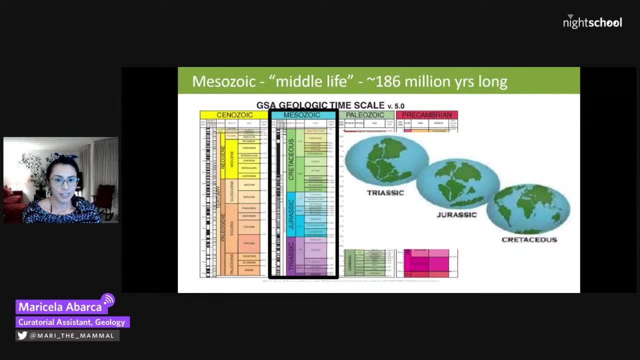 And it's basically like a transitional fossil between fish and tetrapods. So things like amphibians, like kind of paved the way for reptiles, mammals and then later us. Okay, so, leaving behind the Permo-Triassic mass extinction, you start to move into the Mesozoic. 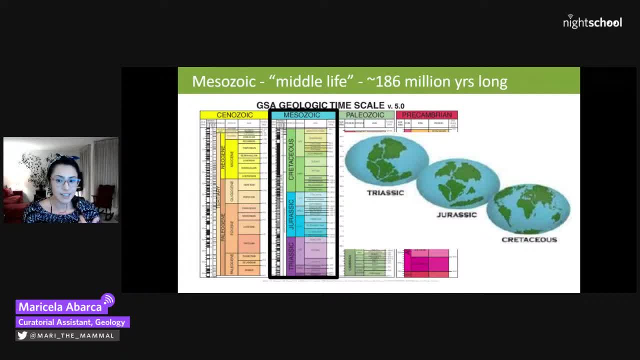 Yeah, Pangea broke up in the Mesozoic. The continents are kind of taking on a formation that's more familiar to us. The climate is really different And we all know that dinosaurs are around in the Mesozoic And, like I said earlier, I'm not going to go into that. 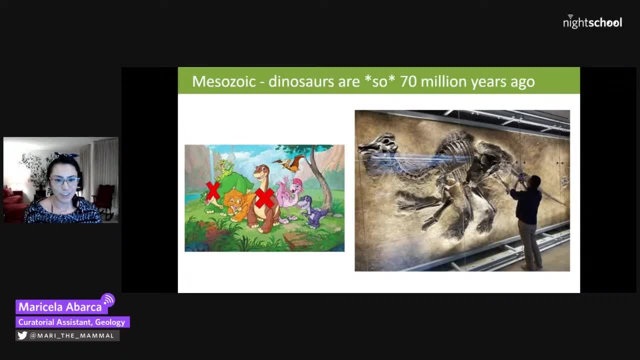 I'm not going to spend a lot of time on dinosaurs because they get all the attention, But I will say- and it'll just be like a total wet blanket stick in the mud and say that Littlefoot and Spike weren't even alive when everybody else was. 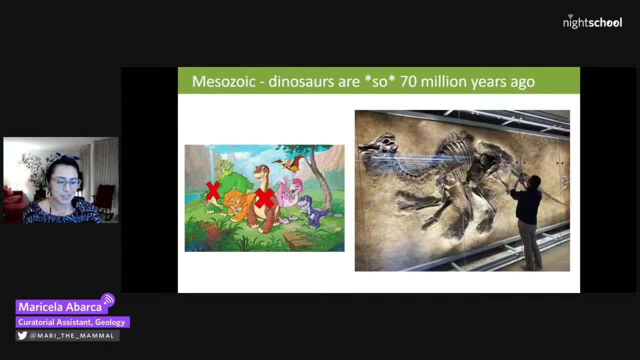 And they actually went extinct before the rest of the dinosaurs and land before time. So sorry to like crush childhood dreams, But aside from that I don't know Like we're. on a brighter note, To the right is a specimen of California's state dinosaur which is a hadrosaur: the duckbills that have these really awesome crests. 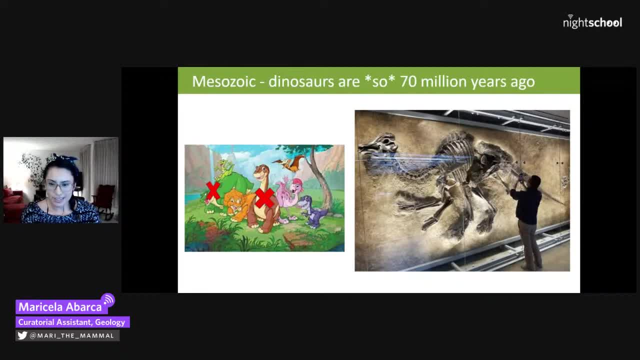 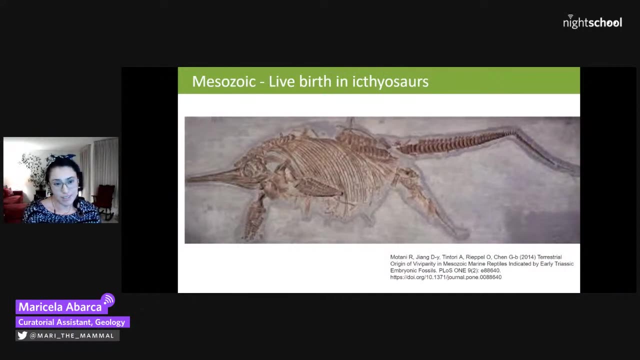 And this specimen has skin preserved with it as well. Yeah, so those are pretty cool. I'll give props to that dinosaur. So in the Mesozoic, aside from dinosaurs, there were lots of other cool things going on, And including marine reptiles. 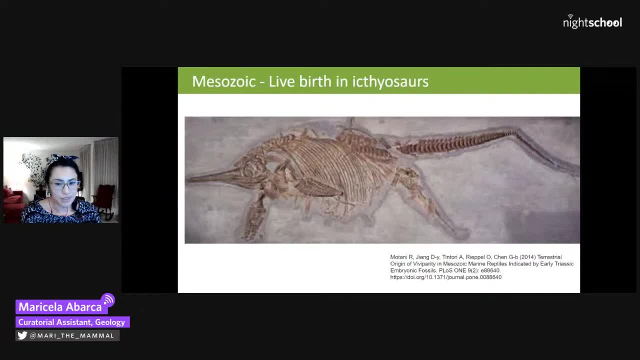 This fossil is of an ichthyosaur. It was found in Germany And you can see it giving birth. So this mother ichthyosaur was giving birth while it died And you can see the little baby coming out. And this image is from a publication. 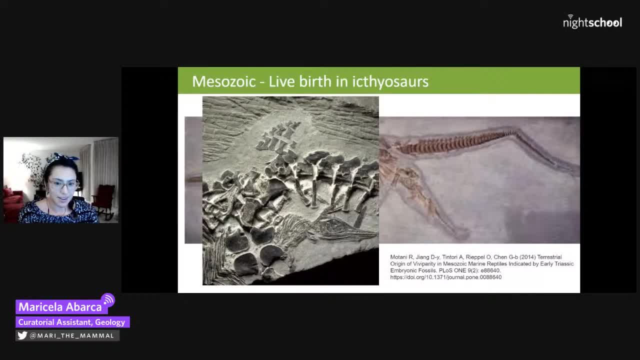 that i got. it's down there on the right. um, yeah, it was just another live birth, so there's actually there's one coming out and then there's other ones that are trapped in the pelvis that you can see in different parts of the image. so ichthyosaurs are marine reptiles that lived in. 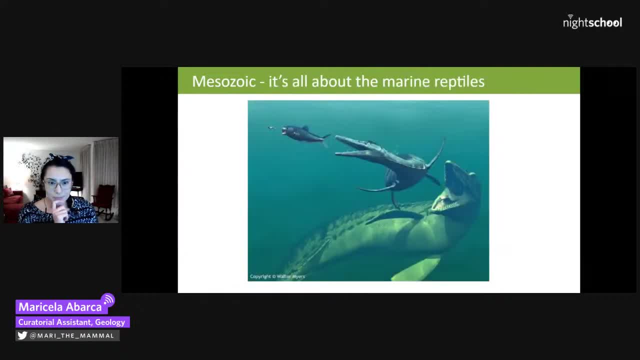 the mesozoic, um, and i'd like i like to think about mesozoic being all about the marine reptiles. there are really scary things going on in the mesozoic ocean: uh, really terrifying predators, very large, lots of teeth, really scary, and it's- uh, it kind of it sparked this thing called escalation. 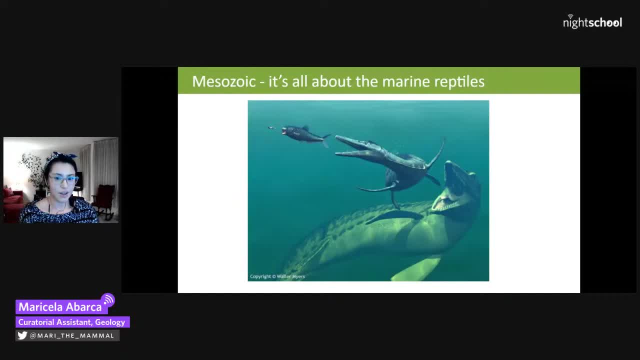 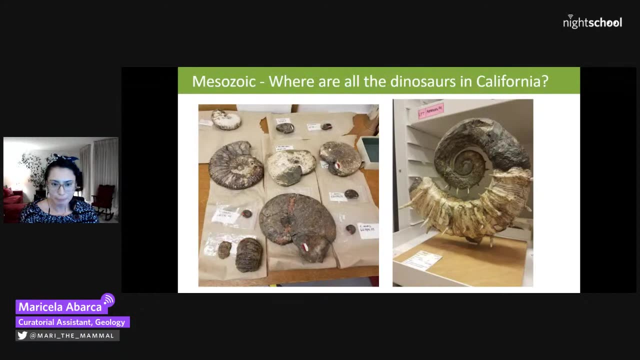 where these predators are getting really big and scary, so prey have to develop these new ways and structures for protecting themselves from being eaten. so you can see this in um ammonites, so ammonites which i think franz might talk about later. um, we're basically shelled octopuses, if you can imagine that, and everybody always. 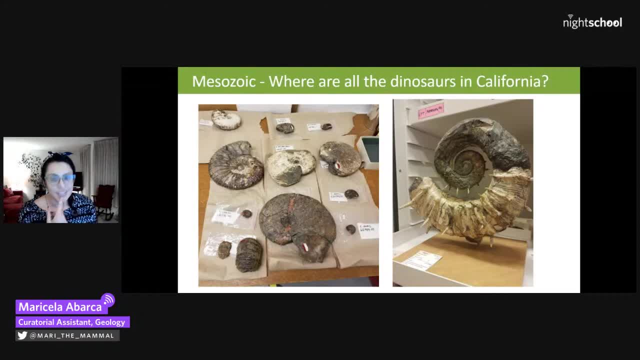 like where all the dinosaurs from california? and the answer is that california was actually mostly underwater in the mesozoic slash, undergoing really violent mountain building in the mesozoic. so a lot of fossils from california are marine and you can see that um example of like escalation and the specimen on the right because for towards 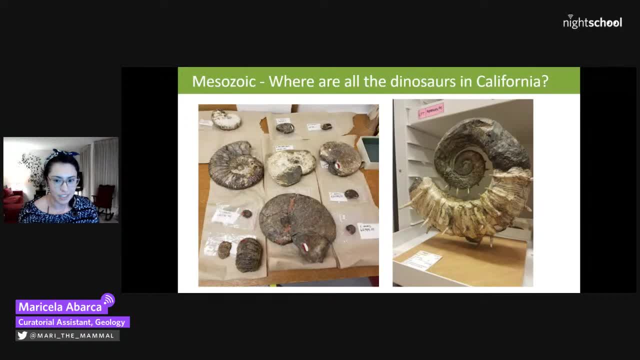 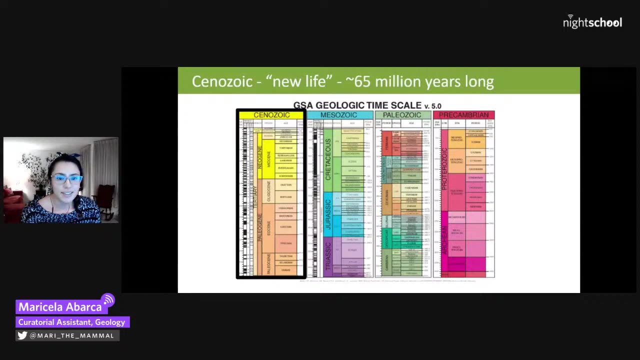 the end of um ammonite lineages, they started like getting these crazy spikes on their shells and opening up their coils, which is supposed to be like an anti-predatory mechanism. okay, so at the end of the mesozoic, the dinosaurs all went extinct and we get the cenozoic and that's where we are now and it's really short, it's only 65 million. 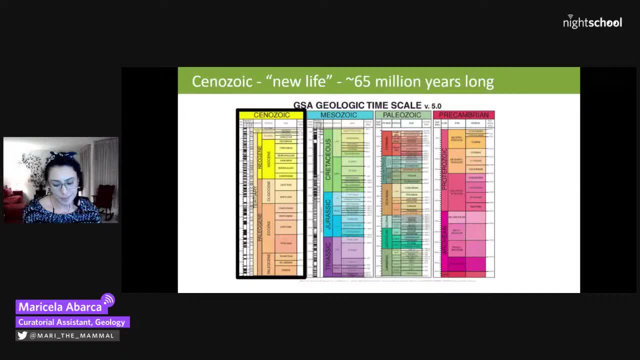 years long so far, um. and there's a really cool exhibit at the hayden planetarium in new york city where you like walk 100 yards and every step is 70 million years. so if you take one step in that exhibit, like you'll miss the cenozoic entirely. if you blink an eye like that's it um. 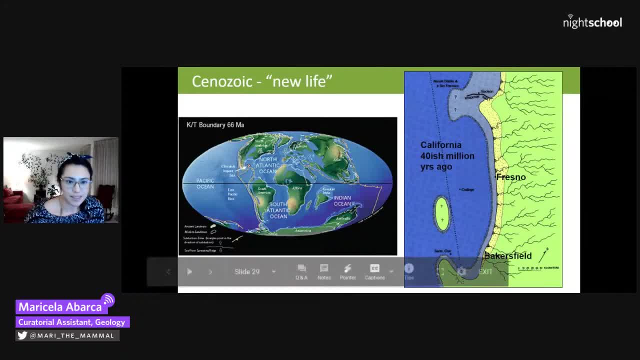 uh, yeah. so here, um in this you can kind of see this is what it looked like- um, after the extinction wiped out the dinosaurs and this is where the impact struck that wiped them out and, like i said, california was mostly underwater in the mesozoic and it was still becoming 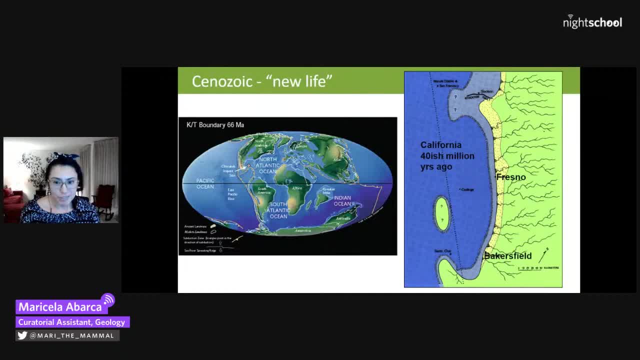 california as we know it today, in the cenozoic, up until like 40-ish million years ago, bakersfield was a beach, if you can believe that. i probably still wouldn't believe that if we didn't have fossils in the collection of like oysters from fresno, because it was all underwater. 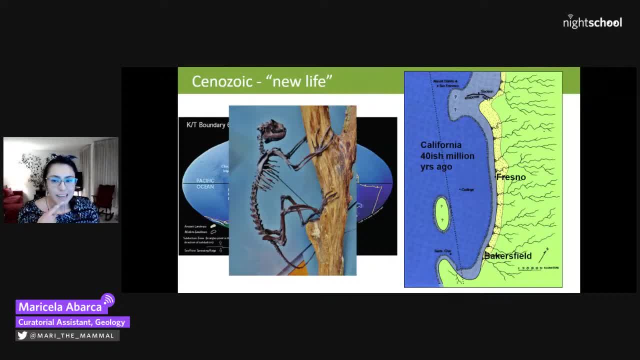 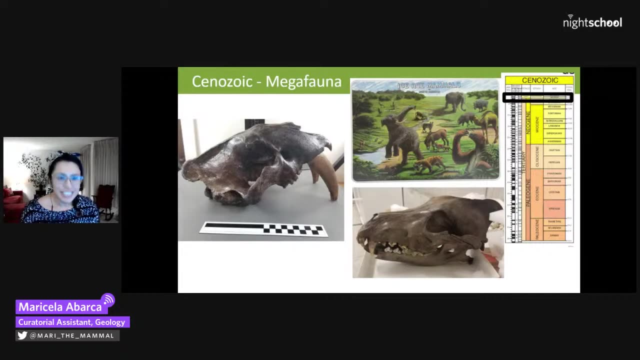 and also during this time, wyoming was like a subtropical forest, so we had a north american primate that went extinct and there were palm trees in alaska. it was very different, but we also have, like, the darlings of the cenozoic, which are the ice age megafauna everybody loves. 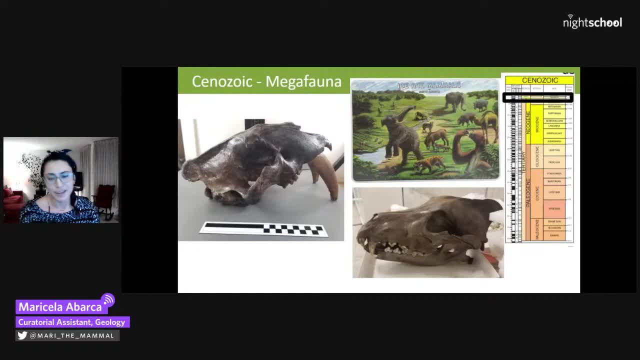 them. i love them. i have a personal bias towards them, but i'm not going to steal nick's thunder because they he's going to talk about them, but i just want to point out like how short their lifespan was on earth. it's just like this outline of the black box in the timeline. 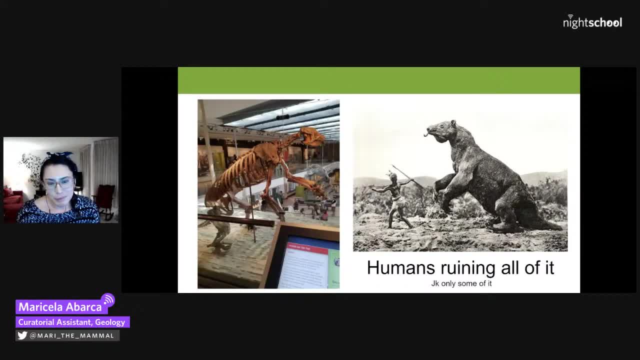 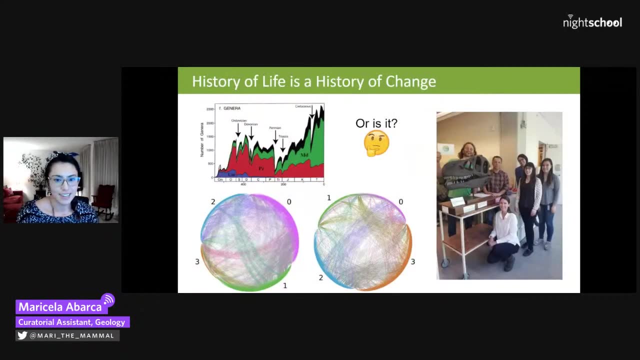 um- and yeah, nick's going to talk about this too- but their extinction, um was largely due to hunting for humans, but also climate change, so humans didn't ruin everything this time, just some of it, okay. so hopefully i've convinced you so far that the history of life is history of change. 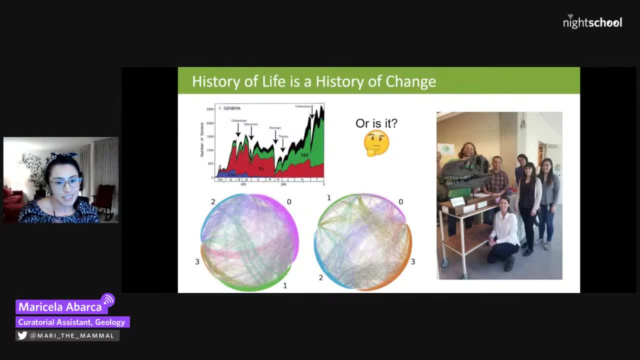 there's a lot of, we've seen a lot of extinction. we've seen a lot of turnover in species, which you can see in this graph to the left. it just shows the five mountains mass extinction, five mass extinctions and these turnover of genera. but what we do at the academy, 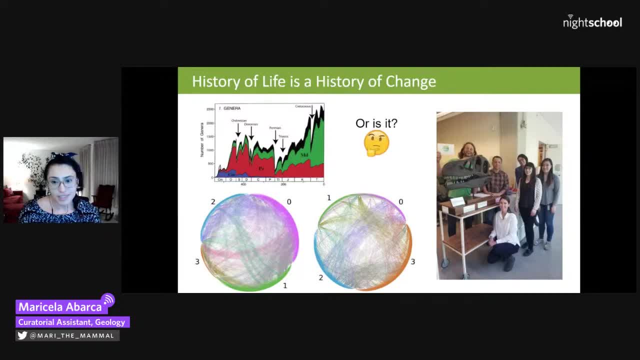 is use um these fossils in the collection that we have and collections from all over the world to kind of like see what the connections were in ecosystems in the past. and it actually turns out that, depending on the scale that you look at these things, communities can be really stable. 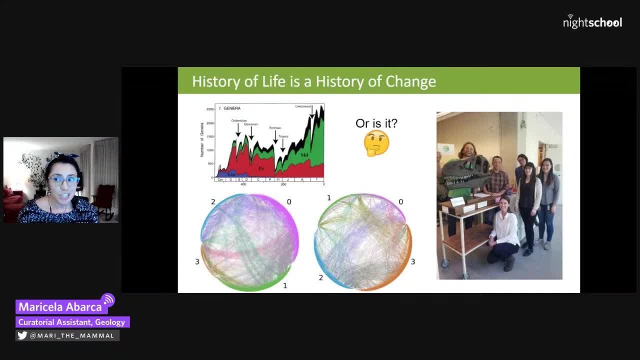 through time and really rapid changes and ecosystem destabilizes communities and it can be kind of important to look at these communities in the past and maybe like forecast or come up with strategic ways to save ecosystems in the future, because yeah thing, like communities in the past have been subject to climate change and really 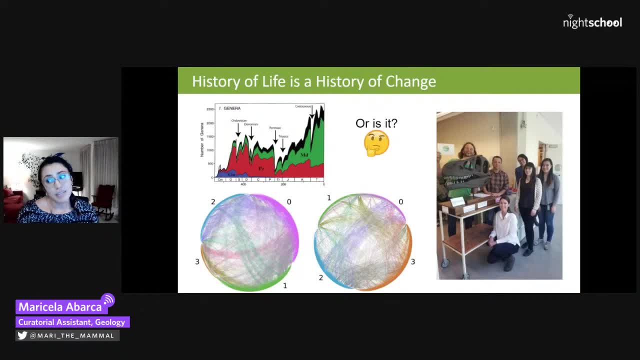 extreme events and thanks to humans, kind of like. what's happening now just at a really fast, on a really fast time scale, and to the right is just a photo of the people in my department who are curating your fossils, and this was like the last time we were all allowed to be together. 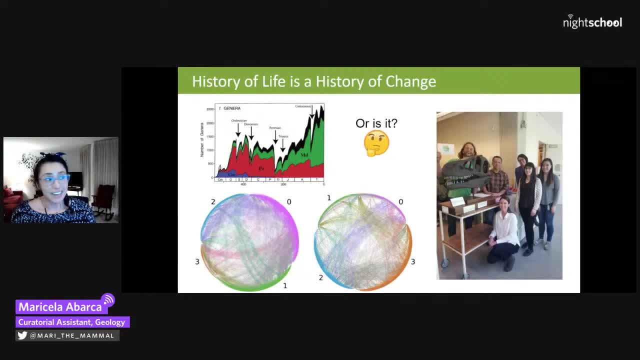 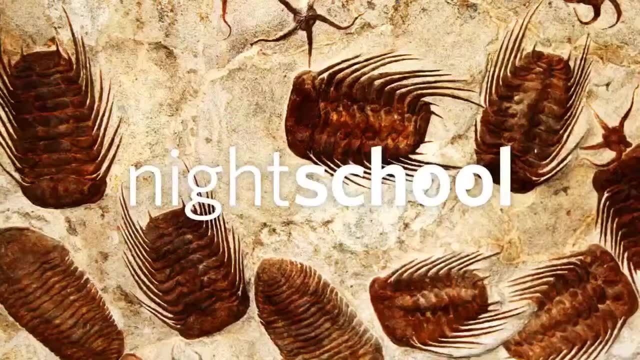 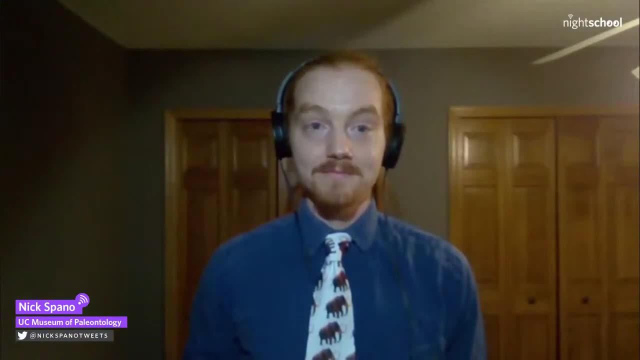 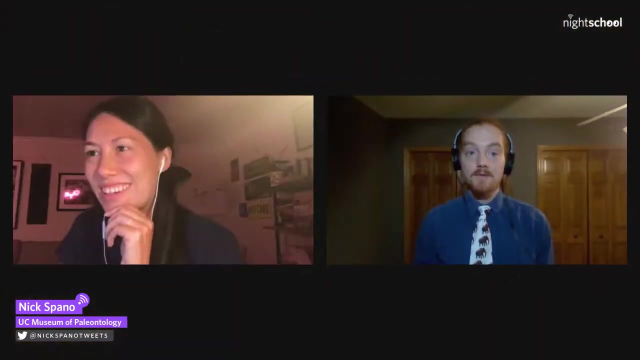 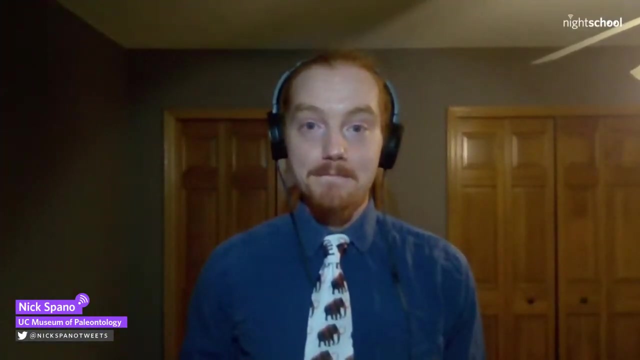 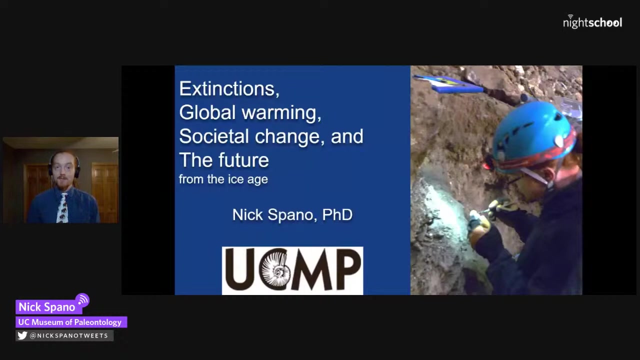 and take a photo. yeah, and I'll be around after Nick's talk if anybody has any questions about any of this stuff. you, you're live, okay. sorry about that, everyone. hello, okay, all right, thank you all for tuning in tonight. thank you to Maricela for that presentation. I don't know Jeff Bezos's network either. 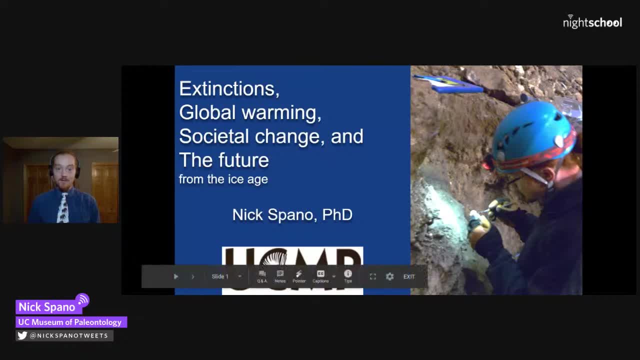 but I did really enjoy your talk, so let's get started. I am Nick. I'm a recent grad from the UC Museum of Paleontology, focus on Ice Age paleontology and its connections to life today, and I really like Ice Age paleontology because, one, it is cool, but, two, it is relatively recent in Earth's history, which 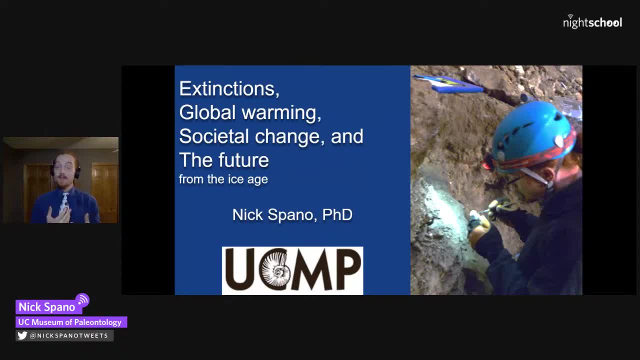 means a lot of stuff is still around, and three that's around. the same time, we see a lot of human activities really picking up. I've volunteered at nightlife events showing Ice Age fossils in the past, so I'm excited to digitally be here for tonight and I'm happy to share these slides. 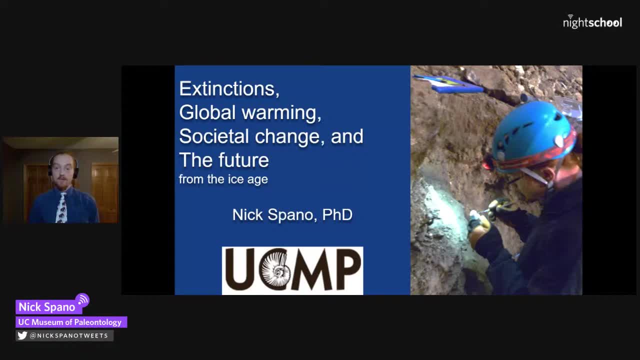 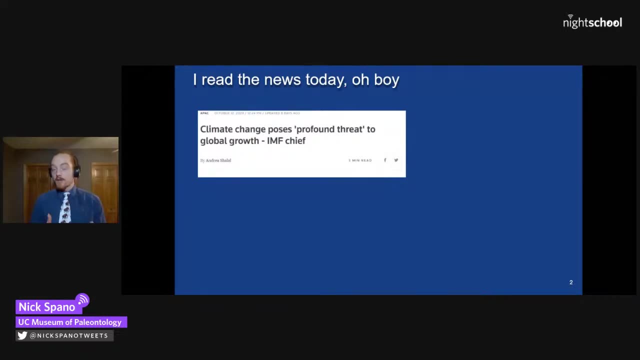 with references if anyone's interested after the talk. So let's see. Okay, All right. If you were to read the news today, this is from October 12th. a little bit ago, There was a story in Reuters about climate change and its profound threat to global growth. Here's a map showing. 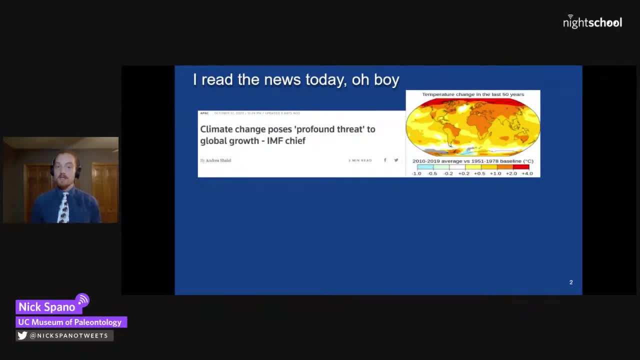 temperature change over the past 50 years and almost everywhere is getting warmer. The World Wildlife Fund back in September came out with their living planet report showing that animal populations worldwide have declined nearly 70% in the past half century. To show that in. 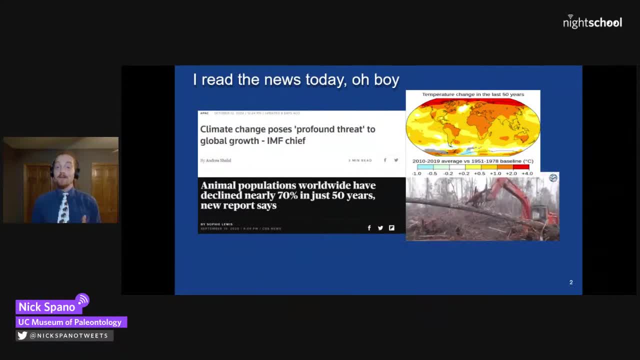 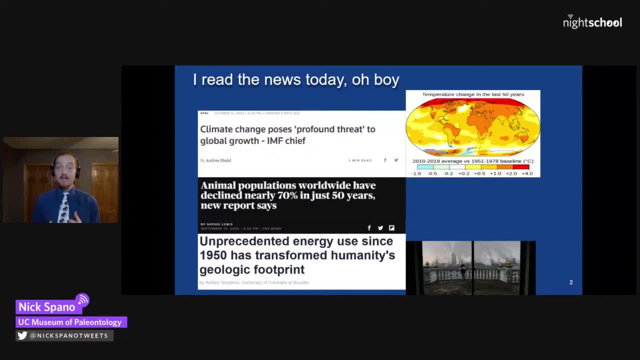 exceeded the energy consumption of the entire preceding 11,700 years, largely through combustion of fossil fuels. This huge increase in energy consumption has, then, allowed for a dramatic increase in human population, industrial activity, but also pollution, environmental degradation and climate change. So a lot is happening to Earth, And to tie this in with tonight's theme, 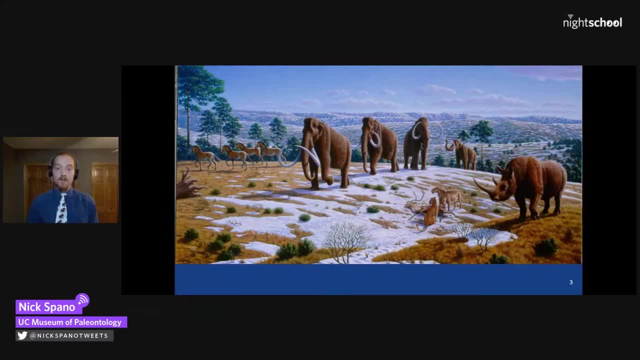 let's go back to the Ice Age and check what the news looked like then. So if you were just hanging out in this field with some woolly mammoths, some horses, maybe some lions, a rhino, and just plop down and start reading the paper, you might find. 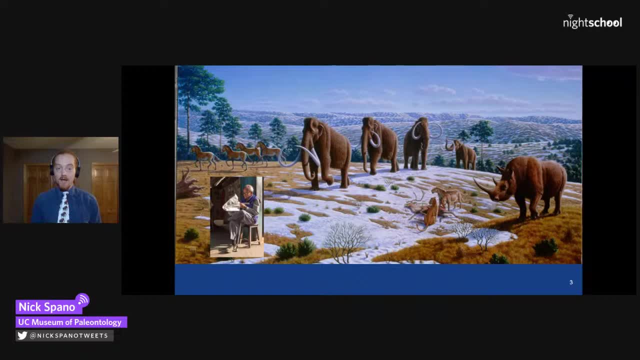 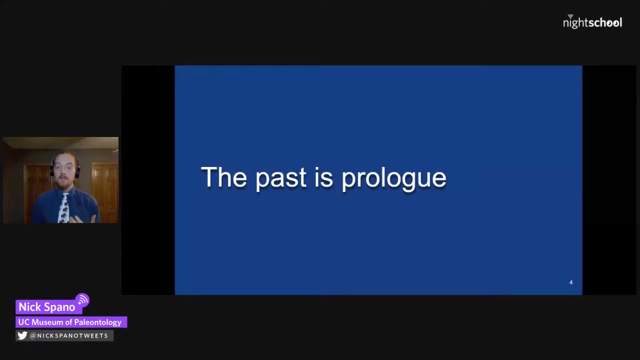 that those stories I was just telling you about were happening in a very similar form during the Ice Age as well. So the theme that I want to get across tonight is this idea that the past is prologue, and for those of you who listen to electronic music, you may be familiar with this as a taiko album. but 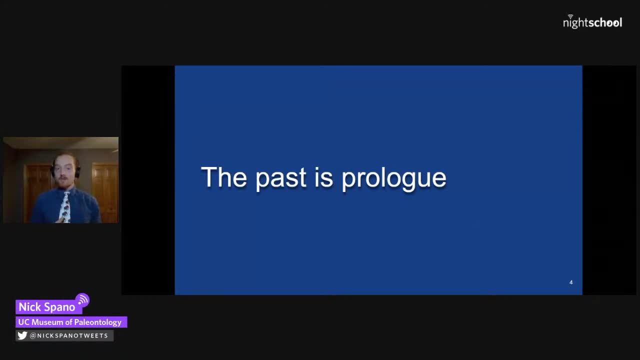 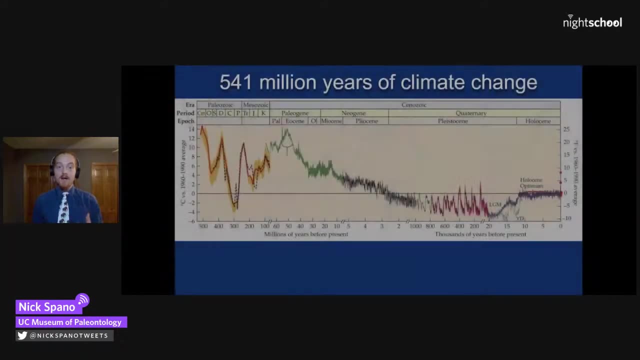 what I mean by that is, what has happened in Earth's history has set the foundations for what's happening now, with very important implications for the future. Tying in with Maricela's talk, here's a figure showing Earth's history. Earth's temperature over the past 541 million years is color-coded by age. 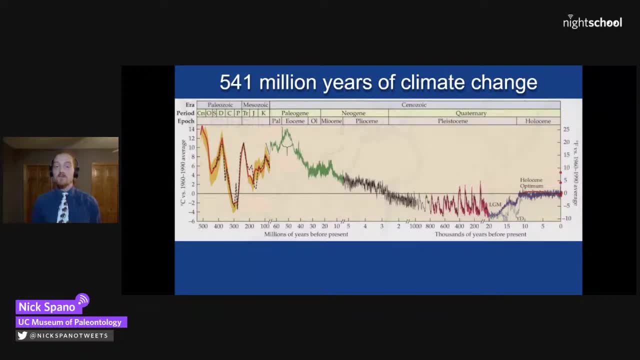 compared to the 1960 to 1990 global average temperature. That's a black horizontal line running a little below the middle. On the y-axis we have degrees Celsius on the left, same thing in Fahrenheit on the right. Note the shift. 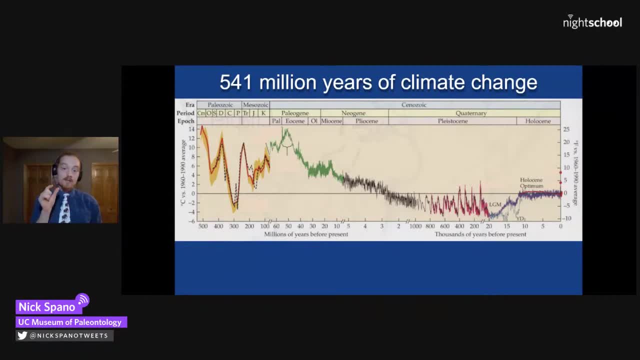 though. in time scales on the x-axis We have 100 million year tick marks, on the most left, 10 million year tick marks below the green wiggle, 1 million year tick marks below the green wiggle and 10 million year tick marks below the. 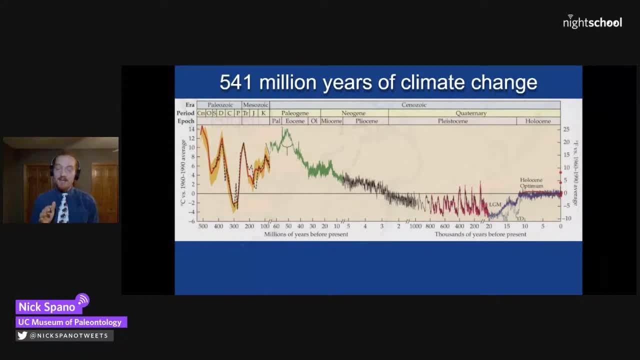 black wiggle, 200,000 year tick marks for the pinkish red wiggle and then 5,000 year tick marks on the right end. Things have been getting generally cooler, as we can see, throughout the Cenozoic over the past 65 million years of Earth's history. 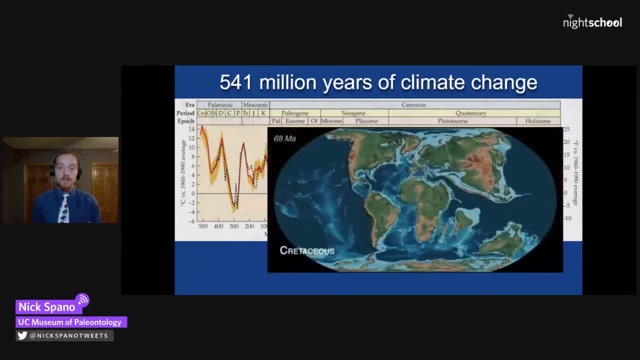 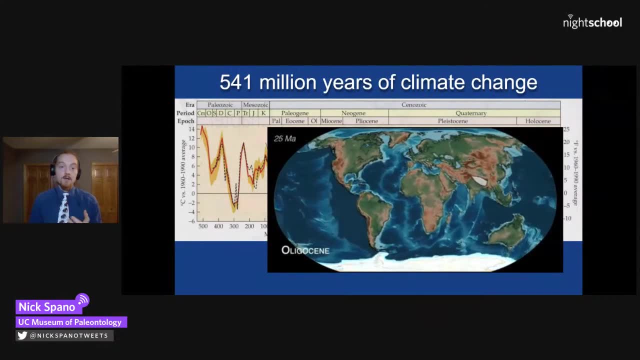 To get at causes of that, here is a map showing tectonic change throughout the Cenozoic. MA means millions of years ago and starting in the Oligocene. and once this gift loops back again, you'll see it a little bit better. 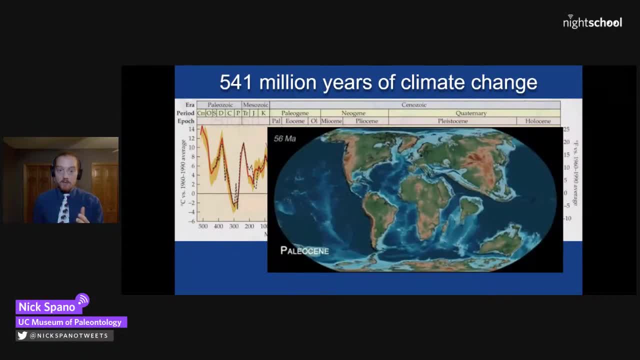 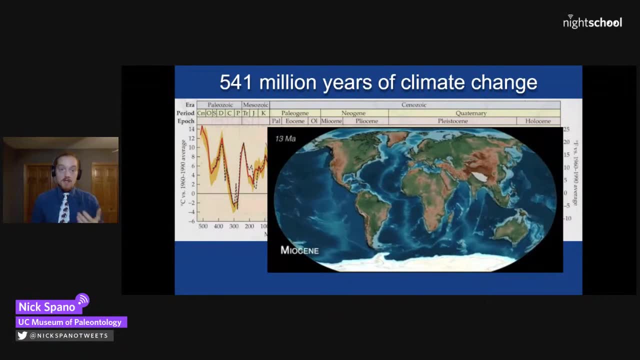 you'll see India slamming into Asia, as it's doing right now, and that caused the uplift of the Himalayas, which cools the rest of the planet by reflecting more sunlight, with ice and into the Pliocene here. that's when Panama forms this isthmus. 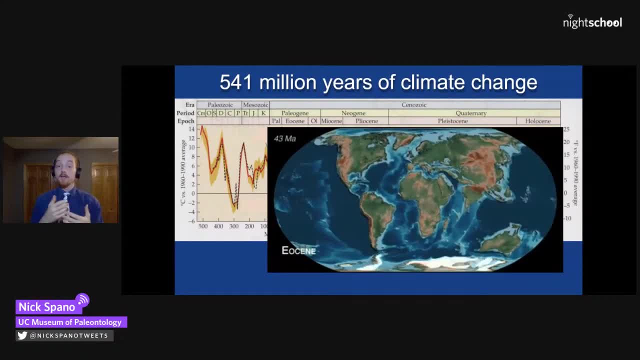 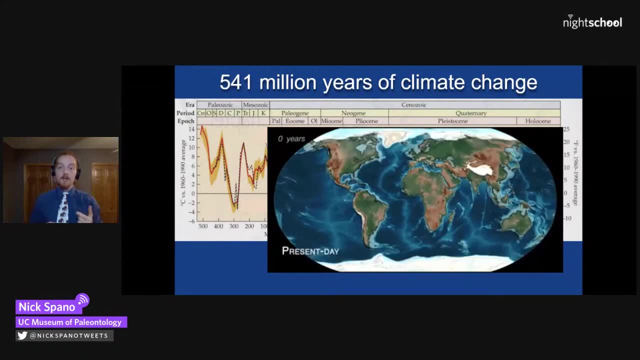 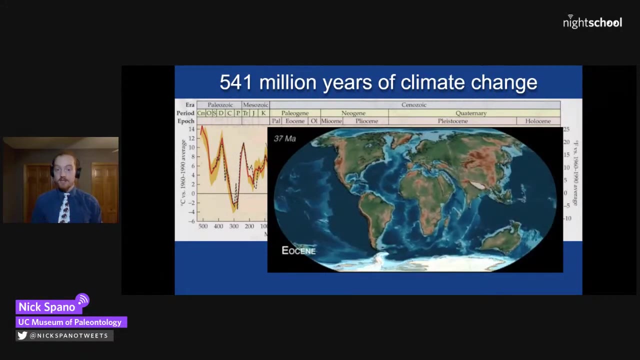 connecting North and South America. that's going to block oceanic currents. that would bring warm equatorial water between North and South America northward and that's going to start Arctic Glacier formation and progressive cooling to the Arctic ice sheet and more cooling from the Pliocene into the 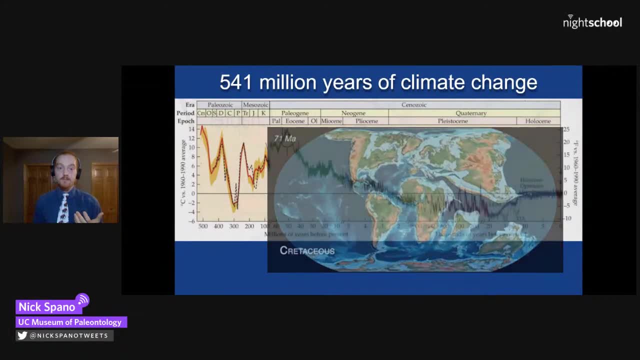 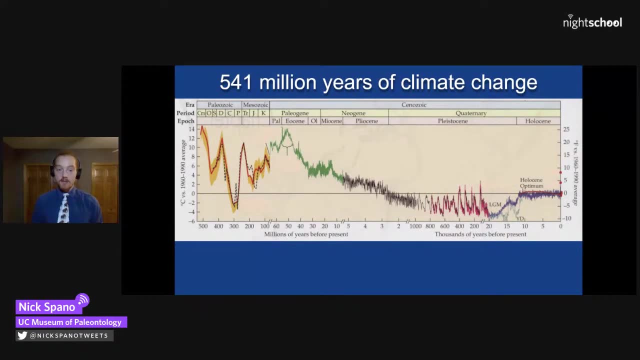 Pleistocene is going to lead to the Ice Age as we know it. So you can also see on this graph a lot of wiggles going up and down, up and down, up and down throughout the Cenozoic. What's causing those wiggles, for the most part, is variations. 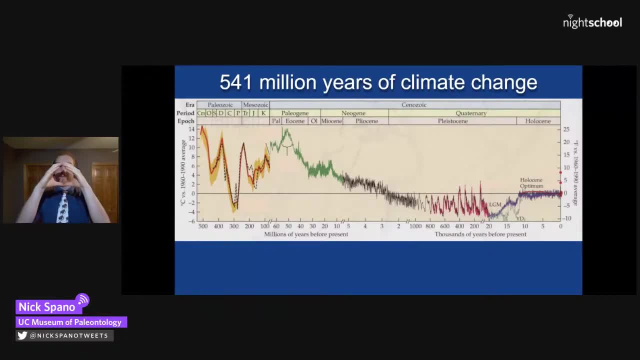 in Earth's orbit, that is, changes from a more circular orbit to more elliptical orbit, changes in how Earth's axis is tilted relative to the Sun. so let's say my fist is the Sun. here's Earth's axis sometimes a little closer, sometimes a little further away. if you're in the 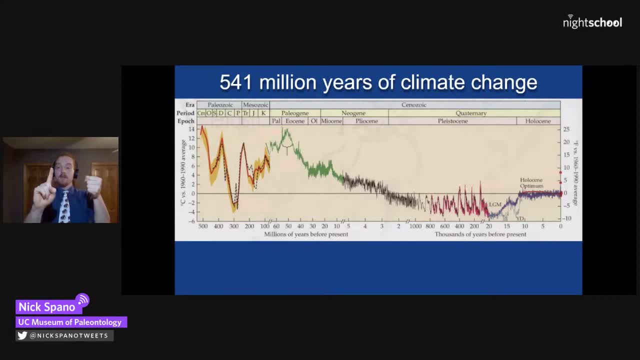 Northern Hemisphere that is, and just like a spinning top Earth rotates through time, and so if you match the frequencies of those variations with these wiggles in temperature through time, they line up pretty well. It's been happening all throughout the Cenozoic, but it wasn't until the Pleistocene that. 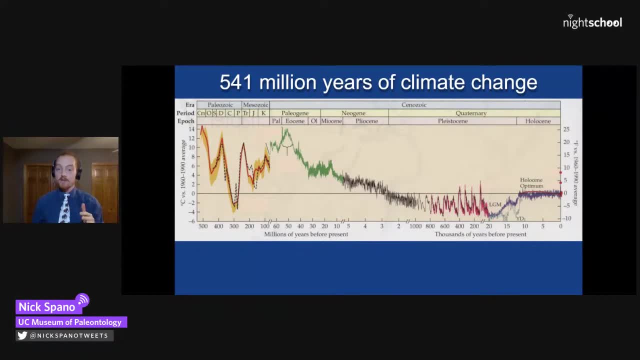 is about two and a half million years ago to 11,700 years ago that the Pliocene had much of an effect. The Quaternary here that box is going to be what I'm talking about most of today, and that is the age of really big Ice Age mammals. 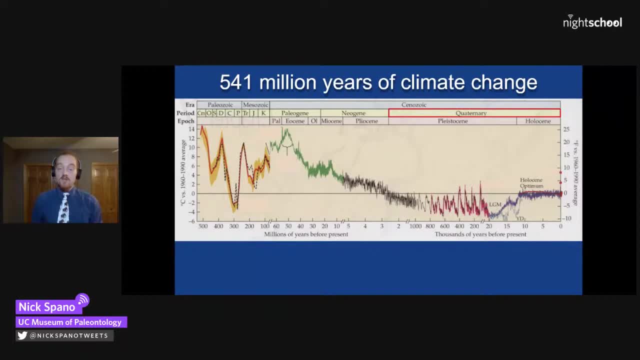 the ones that everyone loves. The most recent, coldest time is going to be what's called the LGM, or that's the Last Glacial Maximum, about 20,000 years ago, and afterwards we get into what's called the Holocene, which is the past about. 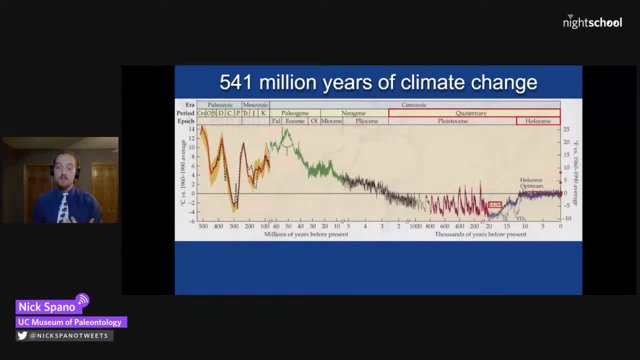 12,000 years of Earth's history where agriculture and civilization started taking off and climate, as you can see here, has been quite stable. Some general takeaways we can get from this graph right off the bat is: yes, things have. 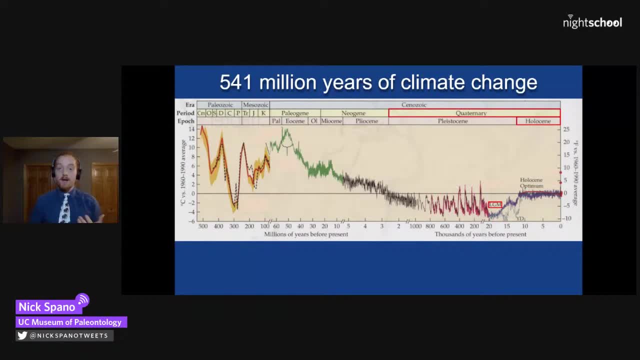 been warmer, but if we keep up greenhouse gas emissions by 2050, that is, 30 years from now- things will be warmer than they have been in the past 130,000 years and it's projected by 2100,- 80 years from now. we could be as warm as never and 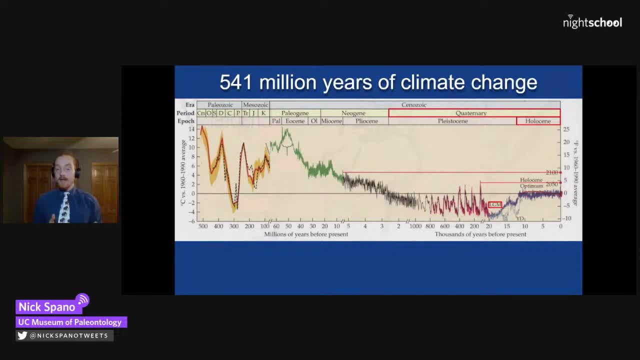 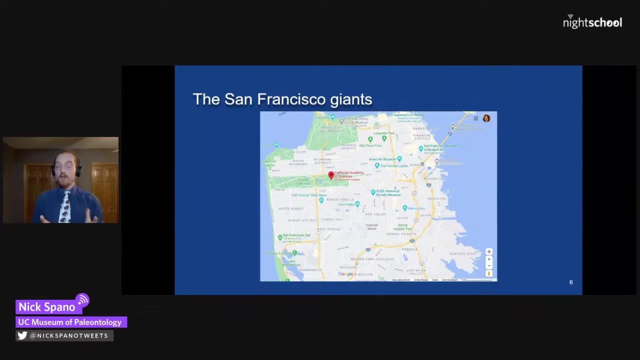 we could be as cold as never in the past- about 8 million years. For now we're still in an icy world, so let's talk about Ice Age mammals. Okay, All right. so here we are in San Francisco. I'm sure a lot of you are tuning in locally There. 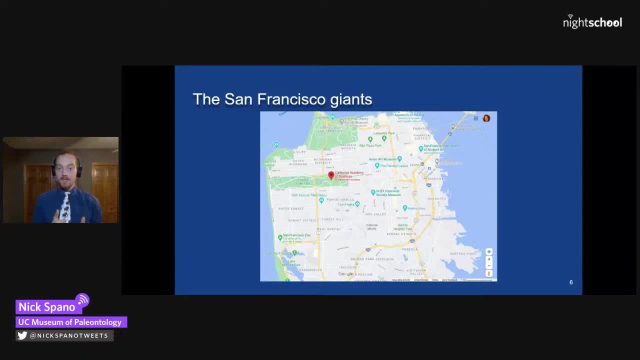 is the red icon showing where the Cal Academy is. and back when Cal Academy was where Chinatown is now, they had a live woman woolly mammoth- Not really live, but a woolly mammoth on display. Some interesting other things. 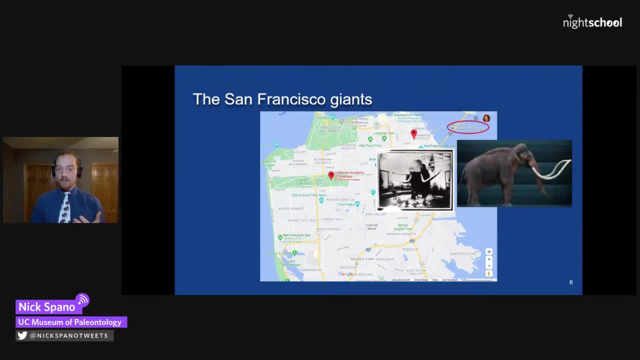 that have been found near San Francisco include a Colombian mammoth fossil that was found when the Bay Bridge was being built. Here is one tooth- It's about the size of a hand That is one molar from a mammoth. This is the Colombian mammoth, not a woolly mammoth, So you can see in this. 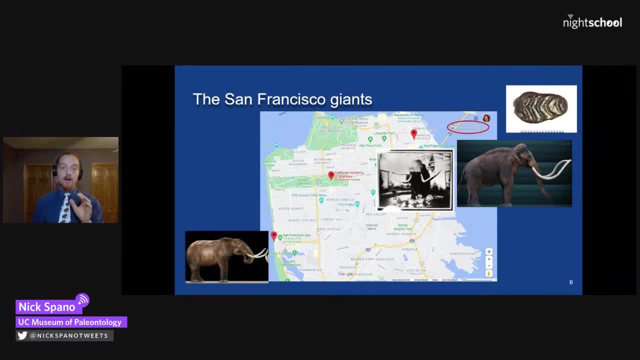 restoration: no wool whatsoever. Over right by the San Francisco Zoo there's been found a tooth about the same size as a Colombian mammoth tooth- a mastodon- And as the Twin Peaks Tunnel was being built, excavators workers found a giant ground sloth- upper arm bone or humerus- Now, no, there. 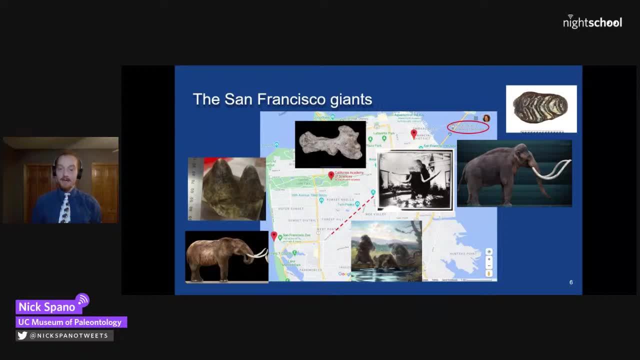 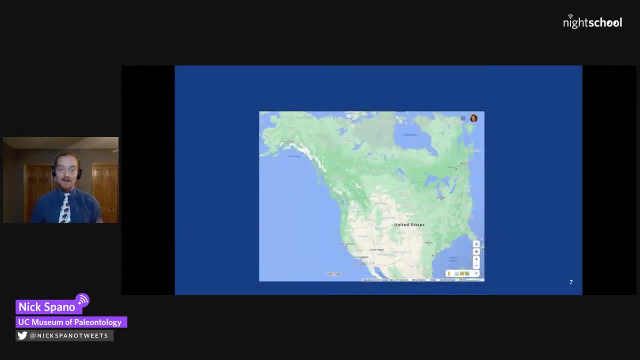 are no living giant animals in the Bay Area left, So let's look at some of these. We'll zoom out a little bit and look to the rest of the US to see if we can find other things out there. If we go down south to the heart of LA, we get to the La Brea Tar Pits- very famous. 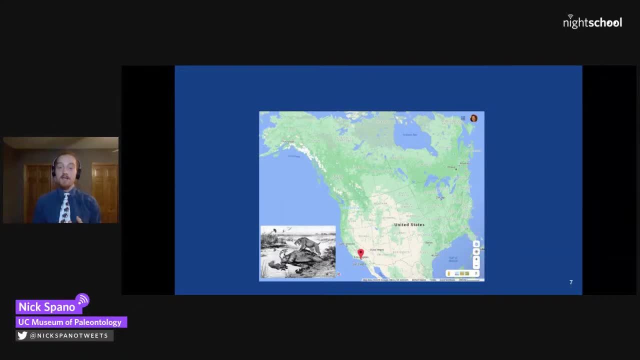 for Smilodon, the saber-toothed cat, California state fossil, and direwolves, the inspiration for the ones in Game of Thrones. But bones aren't the only things that we find as fossils. If we go 15 miles east of Las Vegas, we find Gypsum Cave, which has 13,000-year-old fur. 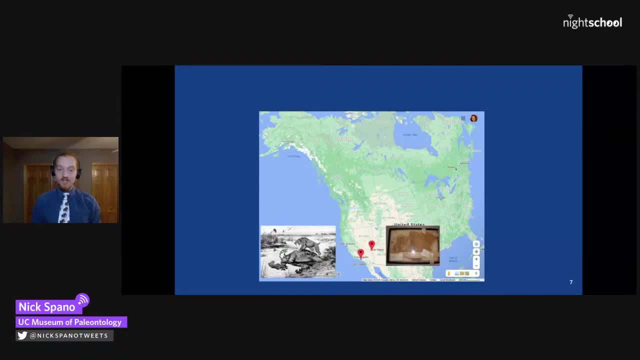 If we cut north to Fairbanks, Alaska, people in 1979 who were looking for gold and permafrost found an entire mummified bison. It's not a modern bison, though Looking at the horns they're much bigger. 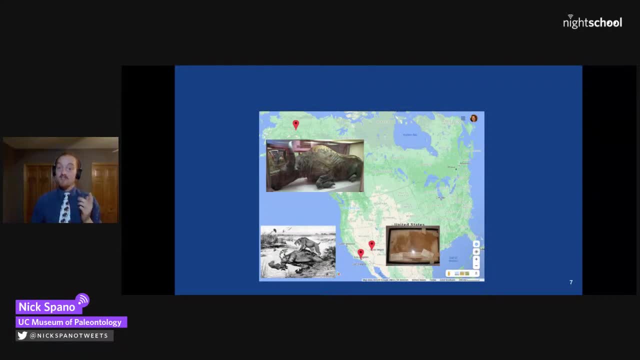 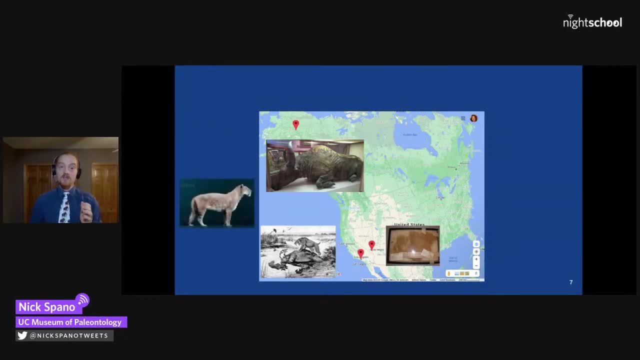 big body. It's a very large body. It's a very large body. It's a very large bison, but it also has claw marks from an American lion, suggesting that that is what did it in. American lions were just like African lions, about 30% bigger though, and bones of American lions can also be found. 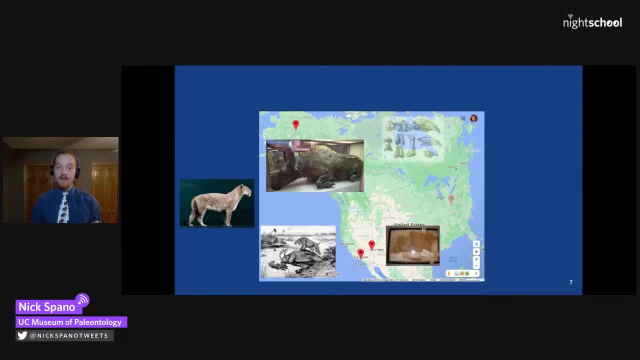 at La Brea and around the Bay Area- David greed area If we head out east- there were fossilized claws found in a Kentucky cave in 1797. They were send to the avid naturalist and our third US President, Thomas Jefferson. he wondering, are those? 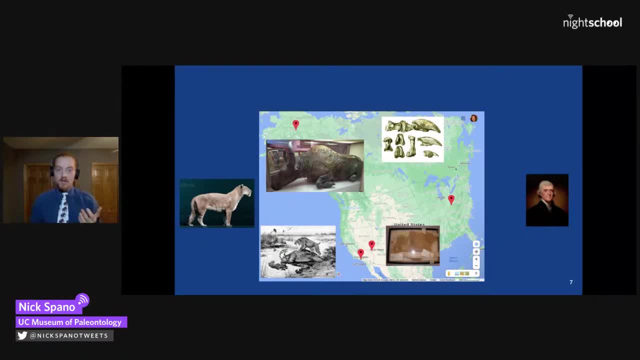 lion claws. are they still live out west? are there other large animals still live out west? so in 1804, a year after the louisiana purchase, jefferson asked his personal secretary, barry weather lewis, to stop by this cave and collect more fossils on his way to meet up with. 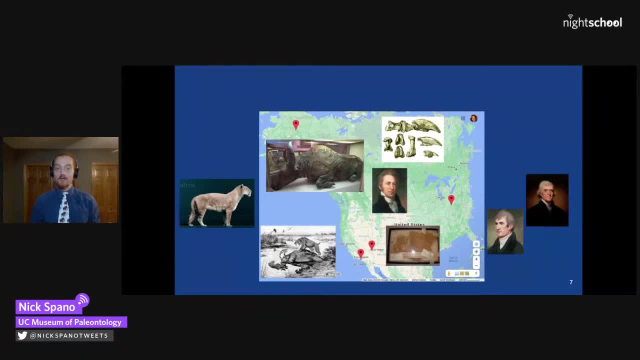 his friend william clark, as they proceeded to find a commerce route to the pacific and they kept their eyes peeled for big animals. this was the first presidential fitness test. just kidding, this was important not as a presidential fitness test, because a famous french naturalist named 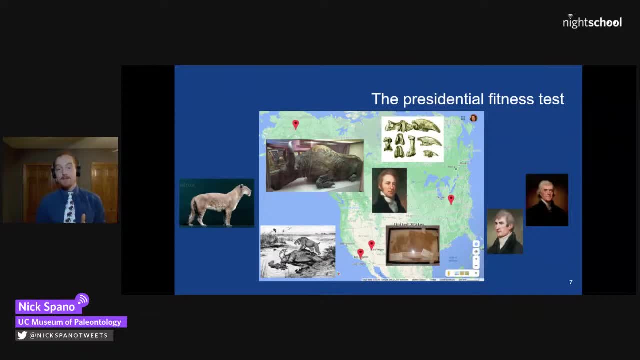 count buffon popularized the idea that at the time animals in the americas were degenerate, the meaning shriveled and diminished compared to those across the atlantic. so national pride was at stake and extinction wasn't established as a scientific idea. so people didn't know if these things were alive really or not. that is, people who were. 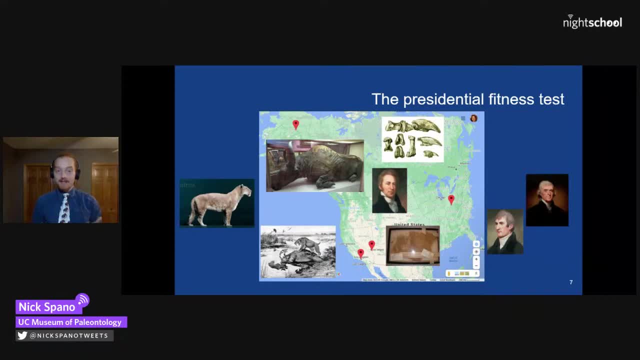 relatively new to the continent. they didn't find any saber-toothed cats or american lions or anything else like that living. they're about 12 000 years too late for that. but lots of bones were collected along lewis and clark's trip and sent back to the white house- the claws that 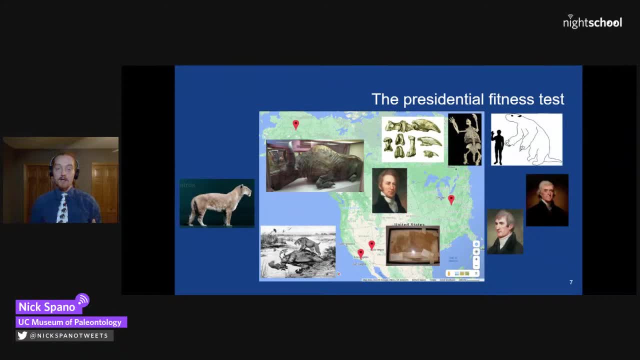 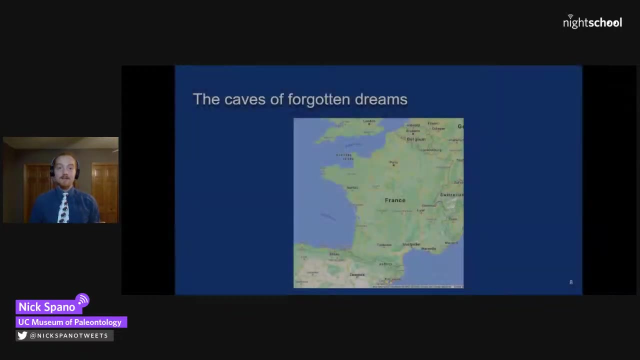 were sent to jefferson. those were of a giant ground sloth called megalonyx, and the species of that giant ground sloth is now called megalonyx jeffersonii. so what did ice age animals look like back in europe then? okay, one of the best ways to look. 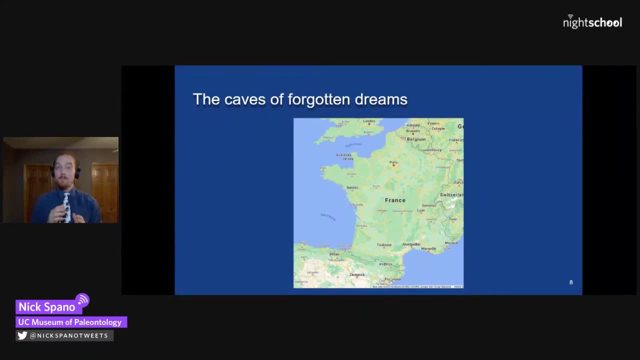 at europe's ice age. history is through its cave paintings. it's a different paleo art from what franz will be doing, but if we start with spain, we have over here. this is the cave of alta miera, and i'll give you a little bit if you want to. 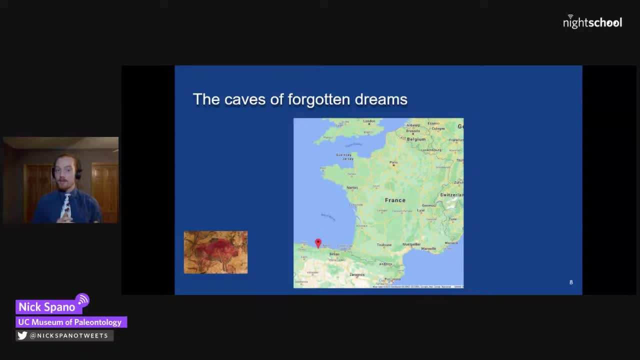 throw in the comments there, maybe what you think this animal might be. i can't see the comments right now, so i'll just take your word for it. but this is our old friend, the step bison restoration vet. and over at another cave getting into france we have a small statue of a cave lion cub somewhere. 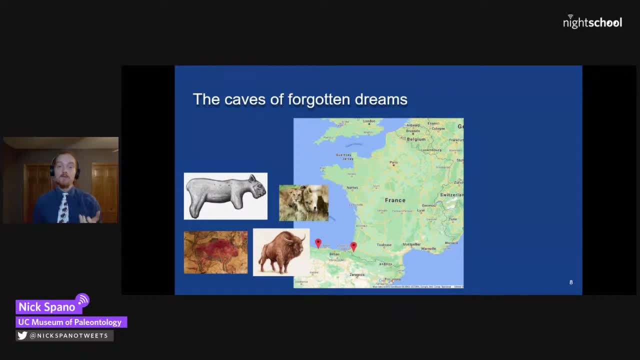 between 80 and 10 000 years old. moving over to leco, one of the most famous cave sites in the world, we find this painting of what looks like a stylized reindeer, but it's probably megaloceros giganteus, the giant deer, which was six and a half feet tall at the shoulders and had a 12 foot wide rack of. 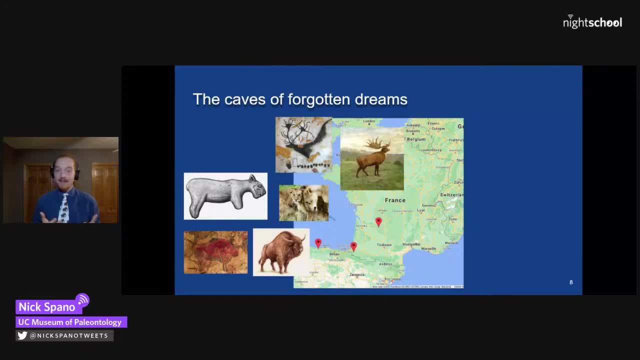 antlers, you can see one of those racks on display at cal academy. once things back open, it opened back up again. and last we have chevy cave, and this cave is really really well preserved because it was sealed at some point. uh, by a landslide. after um in 1994, somebody was exploring around there and found a little tiny. 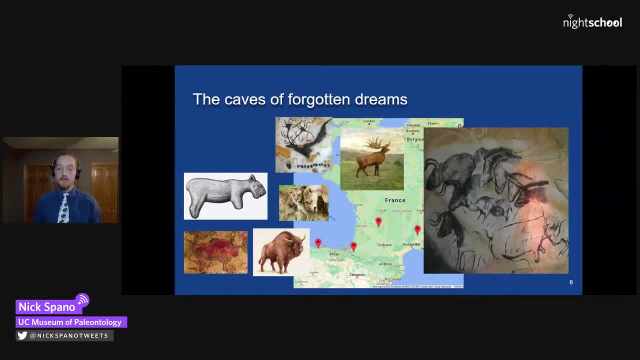 opening to this cave, and so all this stuff is very well preserved in here, and i'll ask for people who are interested in chiming in on comments again what kind of animals they see in this painting. give him a little bit of time, for that we have on top. those look like bulls, those are. 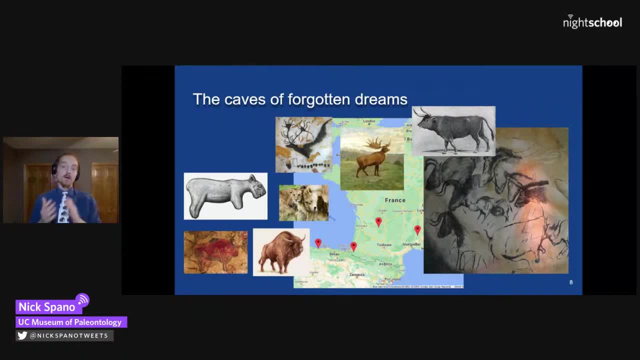 aurochin wolves. Wolves are to dogs as Orokson are to cattle. The last known individual died in 1627 in a forest in Poland. We have- you can see there- some horses which are tarpan. The tarpan was the last European wild horse. 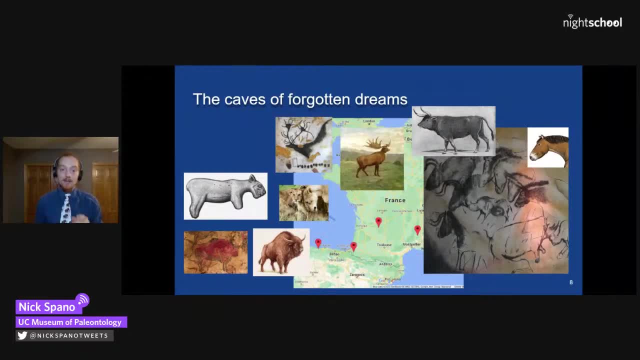 Now horses in Europe are all domesticated And on the bottom there you can see woolly rhinos. There are also non-woolly rhinos in Europe during the Ice Age, And note the two on the bottom right with their faces really close together. 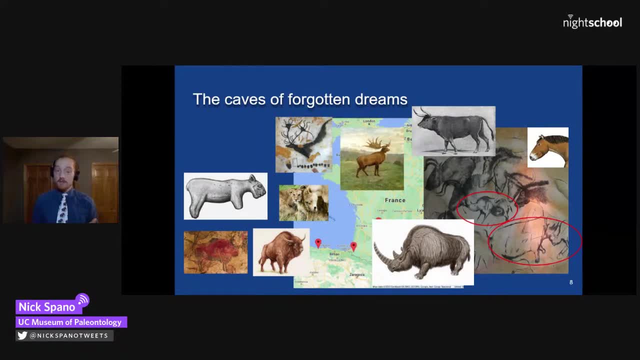 we know that black rhino males today will sometimes fight with each other, So it's interpreted that this is maybe what the artist was getting at. And if you want to look at more- really beautiful, really awesome Ice Age cave art and a whole documentary about it- there is one called The Cave of Forgotten Dreams. 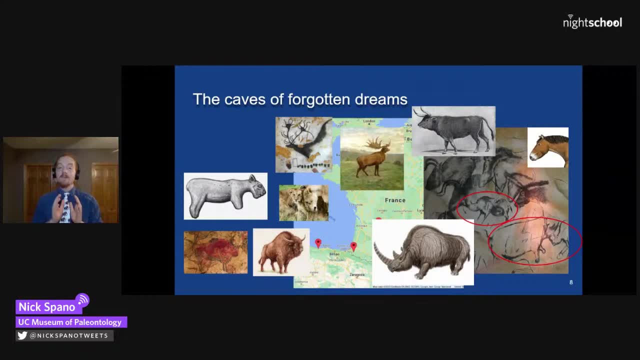 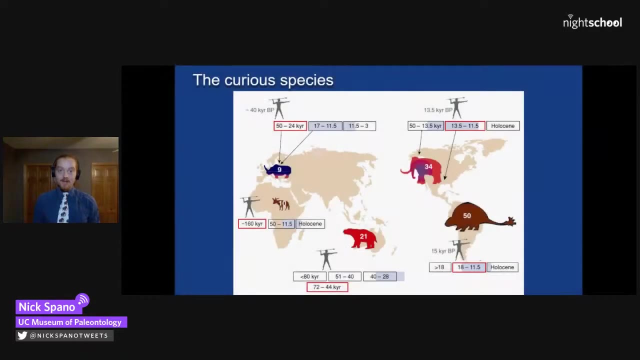 that I highly recommend checking out. So you can see, here everything is slightly different to the animals that we know Really well today, but very similar. So now that we've talked about all these animals, let's talk about us. Here we have a map showing when the first Homo sapiens, sapiens, or us, arrived on each continent. 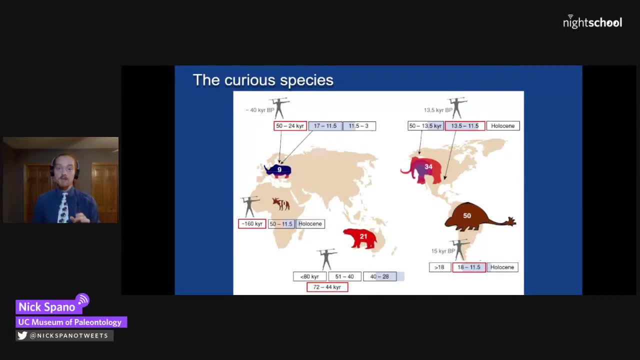 When significant climate change was occurring- that is the blue boxes there- and when large animals became extinct on each of these continents. The age bracket is shown in the red boxes. All those ages are in thousands of years. Animal icons show when large animals on each continent became extinct. 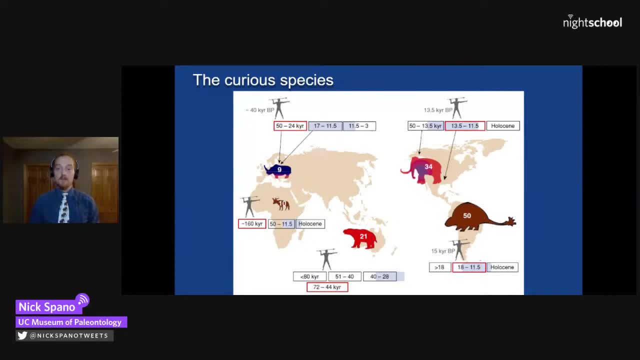 The bigger the icon, the more of those animals that became extinct. The number on each animal shows how many genera, which is a plural of genus, became extinct, And the animal colors represent suggested extinction causes, which I'll get to in a bit. 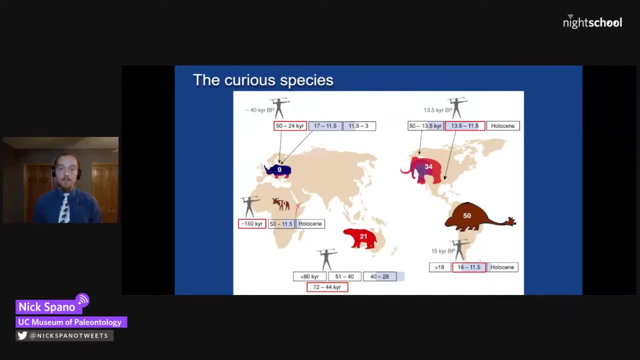 Tracing our footsteps here as we are coming out of Africa. about 10 large animal genera became extinct. At this time, Tool-wise, we only had hand axes, which are cleavers made from rocks. But about 75,000 years ago in South Africa we see some of the oldest art. 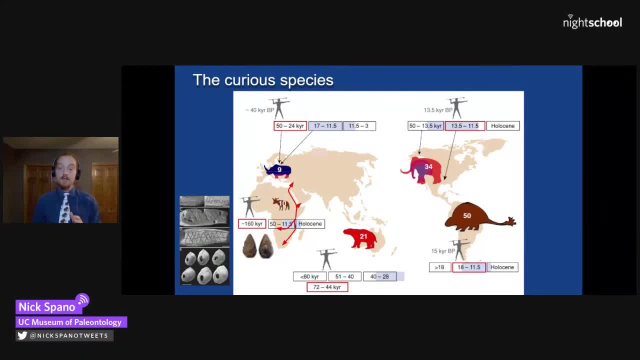 with some complex geometric engravings on bone, deliberately perforated shells, possibly jewelry here. Then we cross the Red Sea to the Arabian Peninsula and spread across Asia quite quickly. Then we went to Indonesia and Australia, followed by a wave of extinctions. that happened in the Middle East, And then we went to Asia and Australia, followed by a wave of extinctions that happened in the Middle East, And then we went to Asia and Australia, followed by a wave of extinctions that happened in the Middle East. 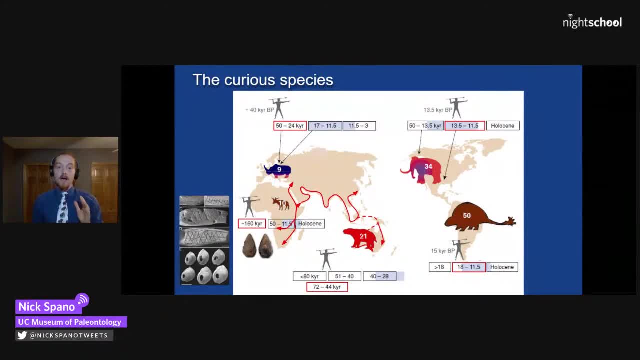 That happened before significant climate change there. The icon we're seeing here in Australia that is of a diprotodon, a rhino-sized wombat of the Ice Age. We also, let's see, got into Europe around this time and invented harpoons for fishing. 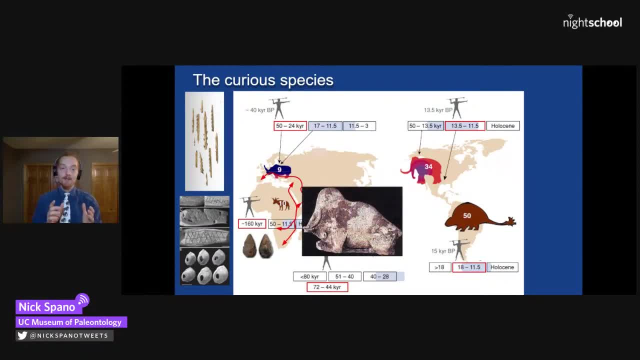 Here we have a very interesting artifact. This is the top of a spear thrower. It's a decoration on top of it, And I want you to take a guess, seeing What you see here, Because there are two different things that come out from here. 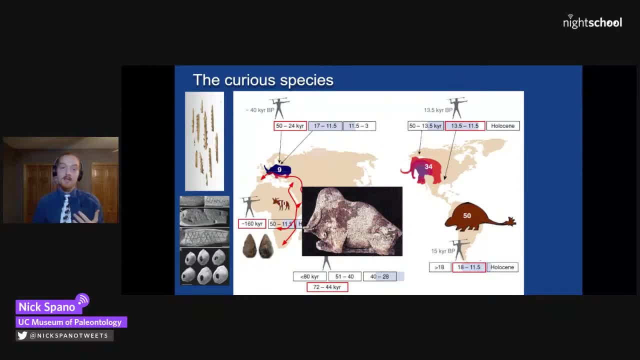 So one of them- at least the first one I saw when I first saw this- is: we look at the bulb on top. It's kind of like a head. We got this curve coming down to the left. Those are like tusks. 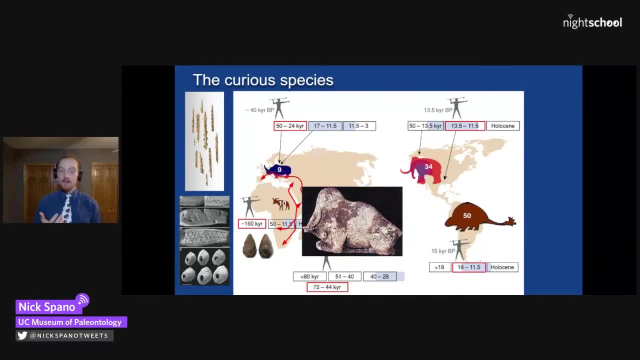 We got maybe a front foot there, back foot there. This is a mammoth, Okay. But then if we look down right where that first leg is, in between the first leg and the tusks, we see maybe what is an eye. 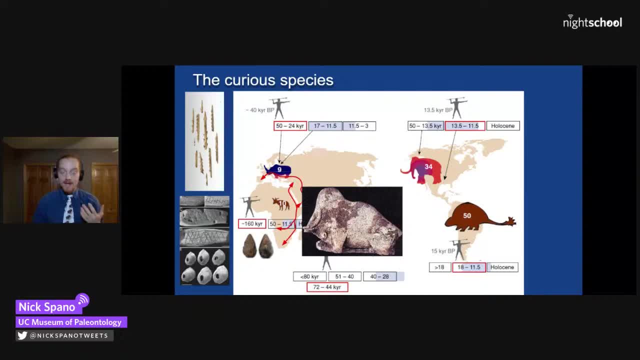 And then the tusks become horns, The head becomes a hump over the shoulders And we see a bull-rated charge. This is the oldest known optical illusion. Very cool. Into Russia, about 50,000 years ago, we find the world's oldest bone needles. 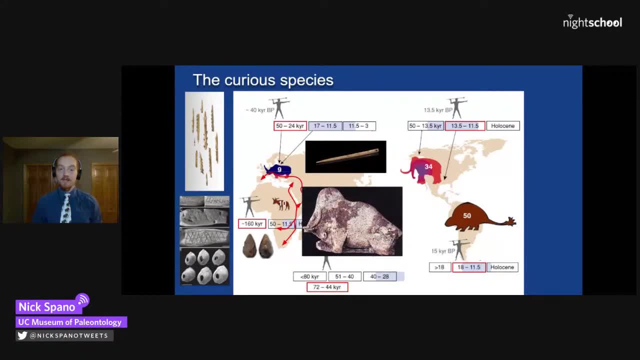 which you know very tiny. It's literally finding a needle in a haystack, And this is very important because finding it in a in a continental or inland location shows that these people were traveling inland, probably because they had these bone needles. Continental winters can be really harsh, so a lot of human populations live by the sea. 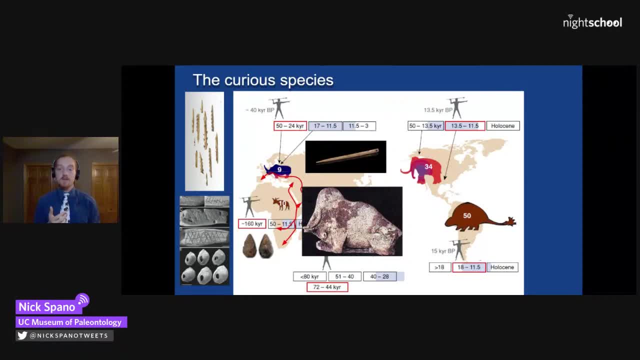 But if you can sew some pelts or fibers together for clothes, you can travel upstream inland and try to weather it out. Then we went up the coast of East Asia across another bridge that was present between Russia and Alaska when sea level was much lower. 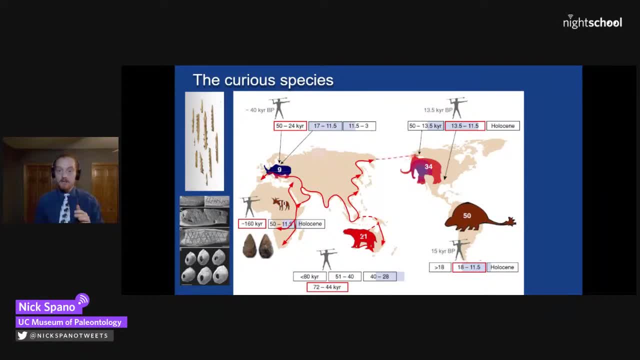 during the peak of this glacial event, into North America around the same time as warming climate and extinctions occurring, And it finally came down into South America right around the same time that climate was changing. The icon here shows a glyptodon, which was a Volkswagen beetle-sized armadillo. 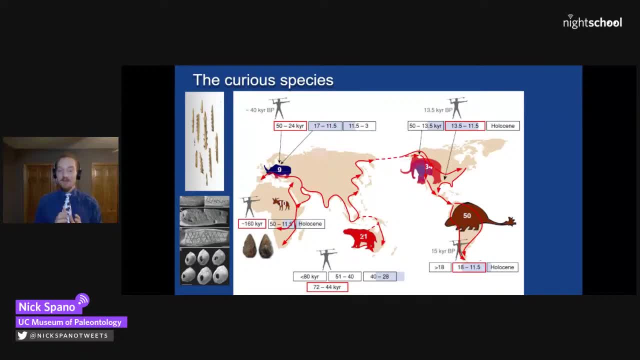 Some takeaway here's. take- excuse me takeaways here. One half of all large animal species have become extinct within the past 50,000 years. Geologically speaking, as we just saw, that is the blink of an eye. 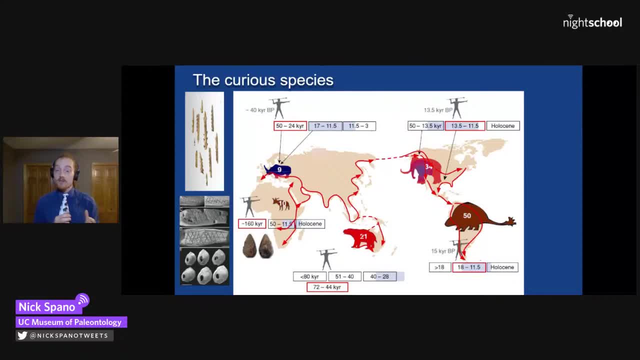 It seems very coincidental that these extinctions mostly occur right around the same time that we showed up. Could be due to overhunting, could be due to habitat loss. However, we know, looking at the past of extinctions, climate change can be a really important cause too. 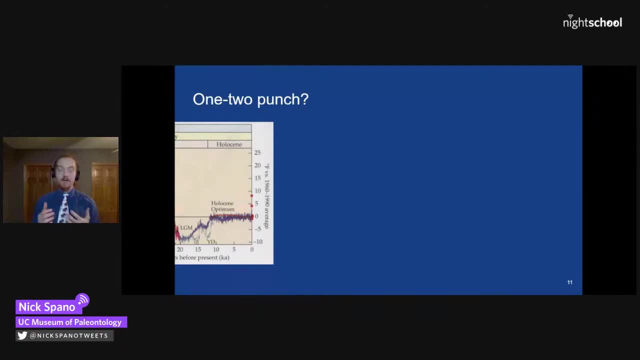 So people have been arguing, bickering, saying, bickering, back and forth for about the past 60 years about whether climate change- given we were coming out from the last glacial maximum into warming for a lot of this- was the cause of these extinctions. 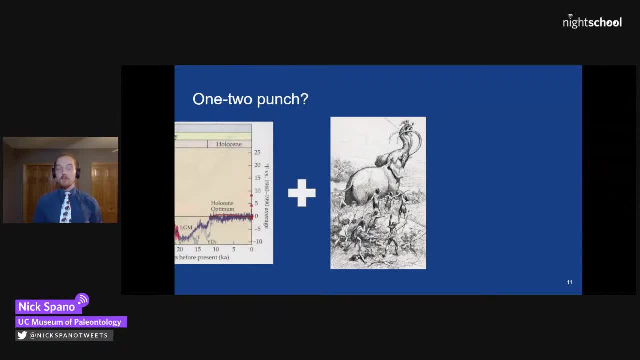 or maybe hunting of these animals and habitat modification, other human pressures, were causing these extinctions. Now we're finally getting to a point where we can ask: well, why not both And these complex stories are challenging to try to understand But become much more interesting if we can put those pieces together. 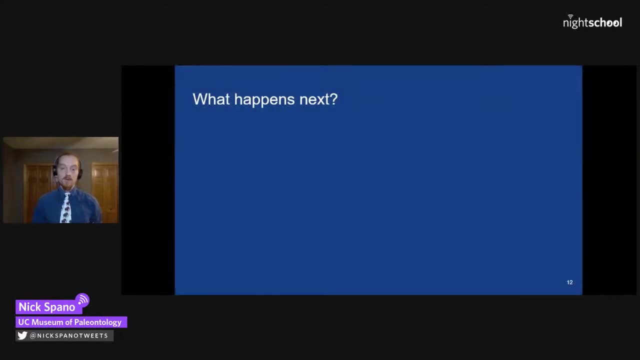 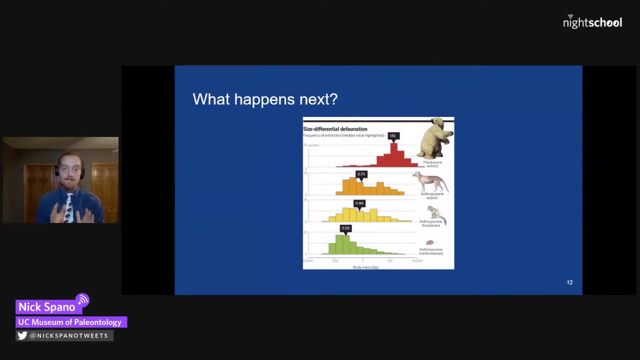 So now we got a question of what happens next. Here we show a figure of body mass distributions of different animals. We see on the top that is Ice Age, and we see things getting smaller and smaller and smaller. Anthropocene here means everything since 1950 going down through time into the future. 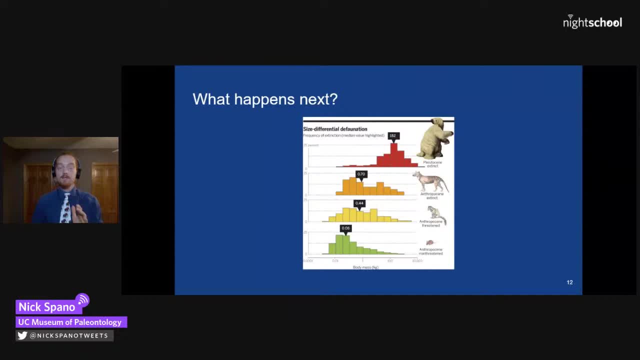 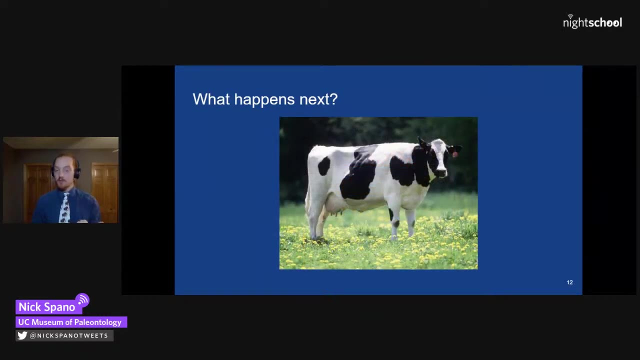 That is looking down this figure. And if we keep up these trends, in the next 200 years, what do you think? the biggest animal on Earth is going to be? A cow. So that means no more giraffes, no more whales. 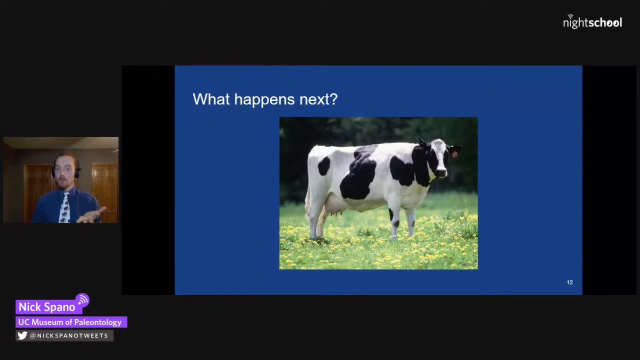 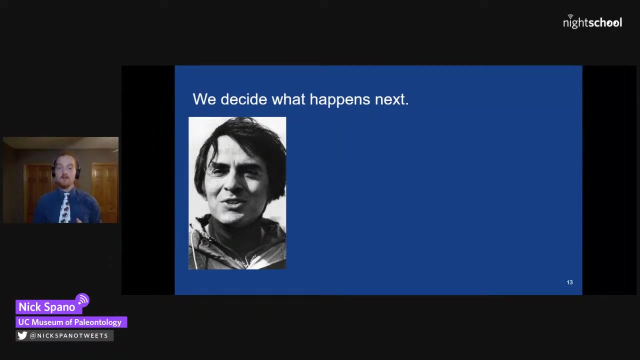 no more elephants, no more hippos, no more rhinos, none of that- If trends from the Ice Age continue with what we're doing today. But we decide what happens next. To end my presentation, I'll quote the great science presenter Carl Sagan, who said: 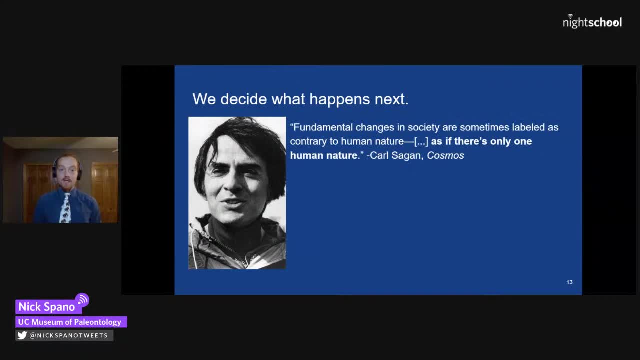 Fundamental changes in society are sometimes labeled as contrary to human nature, As if there's only one human nature. We know better. Prehistoric peoples had no global communications, education or management systems in place to address these concerns, But we do So, although the past is prologue. 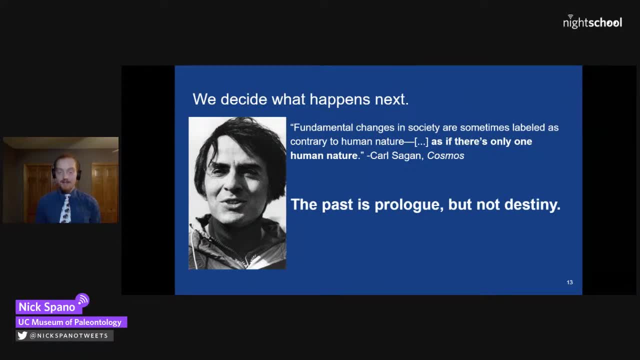 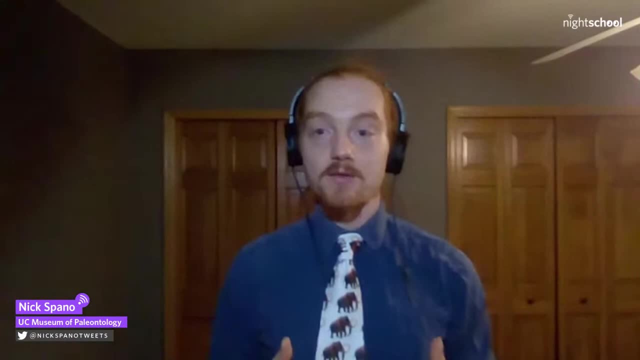 it doesn't have to be our destiny. So with that, thank you so much for your time, And Maricela and I will be signing on now for a joint Q&A And are happy to address your questions. Hi Thanks, Nick and Maricela. 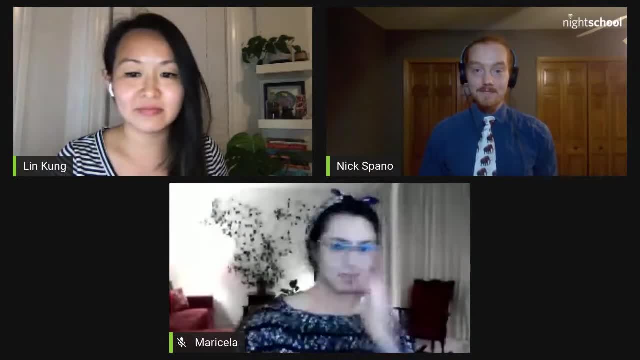 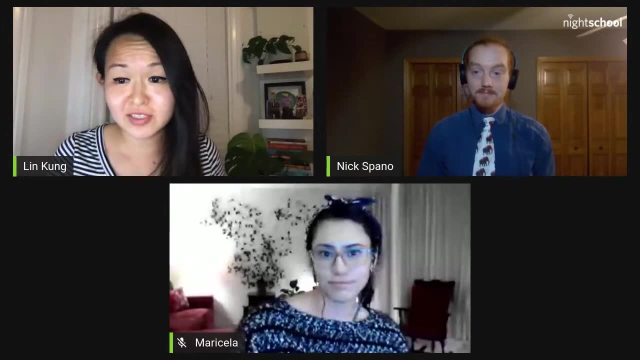 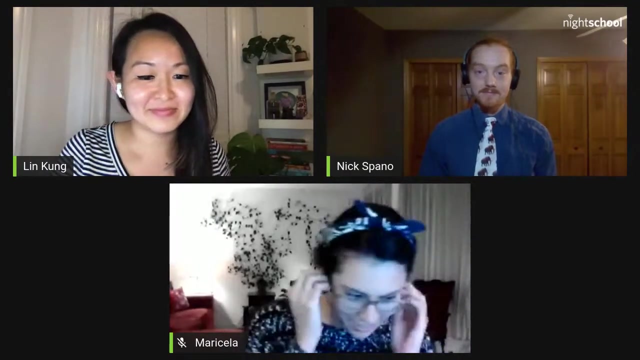 We have a few questions, So let's get started. Maricela, why do some beings become fossils and others don't? AKA, if I want to become a fossil, what do I do? Right, Maricela? I think you're on mute. 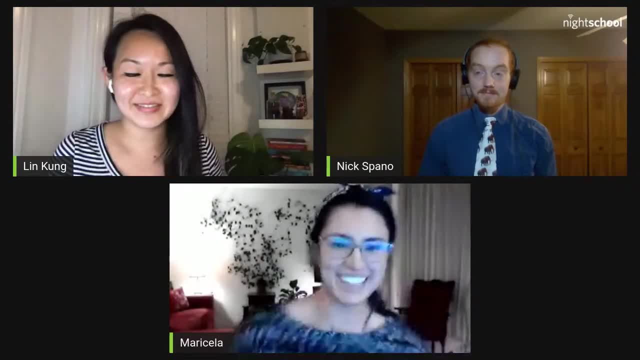 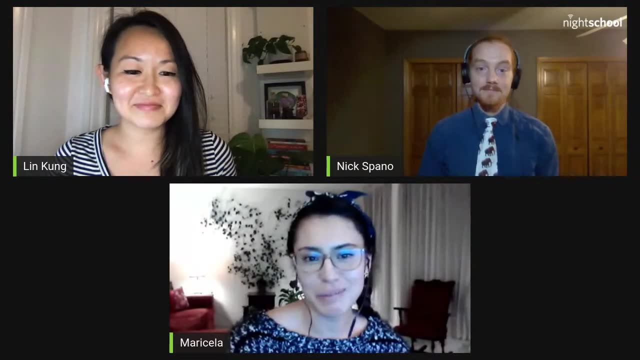 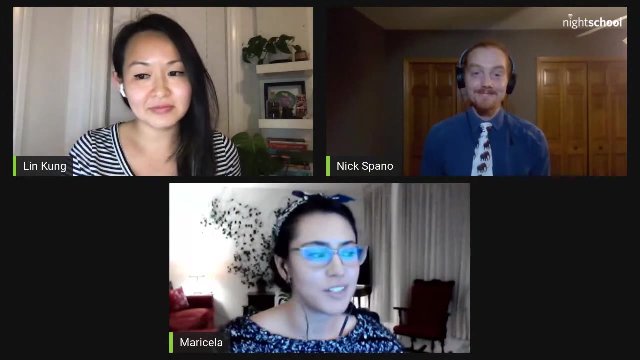 Yeah, Okay. Yeah, that's a really good question And I actually think Nick and the UCMP crew did a really funny how to become a fossil exhibit at nightlife once. But it is really hard to become a fossil. You have to die in the right place. So somewhere that you're going to die get covered in sediment so you don't decompose. You have to die in a place where tectonics aren't going to scatter your bones all over the place, And on top of all of that, you have to be discovered by someone later. Who cares? And it was what they found, Yeah, So if you want to become a fossil, best places to die are the bottoms of lakes. Or just ask someone to throw you The bottom of a really calm river lake bed, Because then the sediment will cover you up. 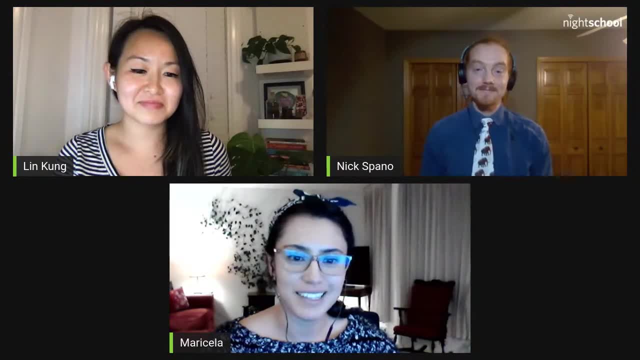 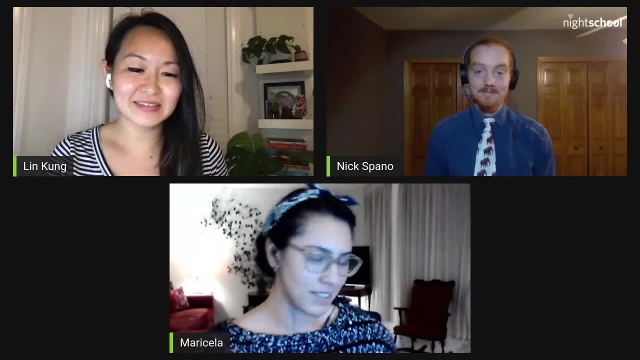 And you'll just be undisturbed for a really long time. Yeah, And then hopefully someone will find you, And hopefully someone will find you. Yeah, There's really cool deposits in Germany and other places in the world called Lagerstätten. 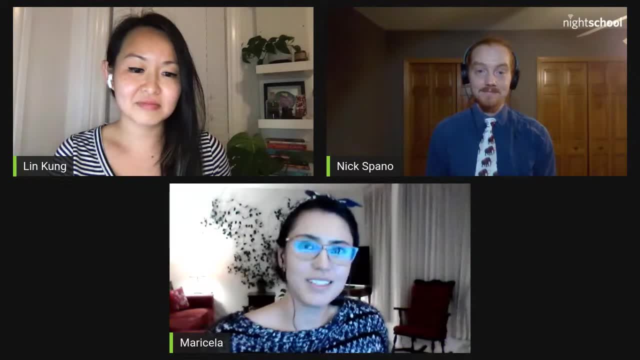 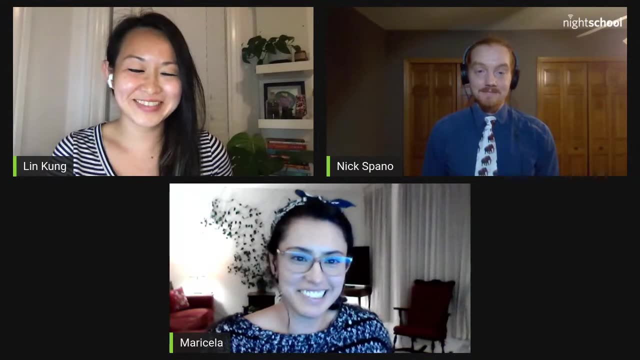 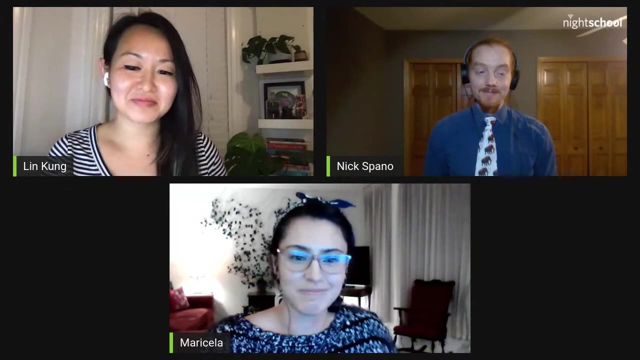 Where they preserve really excellent, really detailed fossils. So you could probably get asked to get buried there. Cool Nick, do you have anything to add to that? Nothing I can think of. Yeah, The first thing that comes to my mind that I would add, if anything, is kind of a sad note. Which is a great place to preserve biological materials, is a freezer, And we have a giant outdoor freezer in the Arctic, But that is rapidly disappearing. But that is also why we're seeing many more of these Ice Age fossils coming out from Russia and Canada and Alaska. 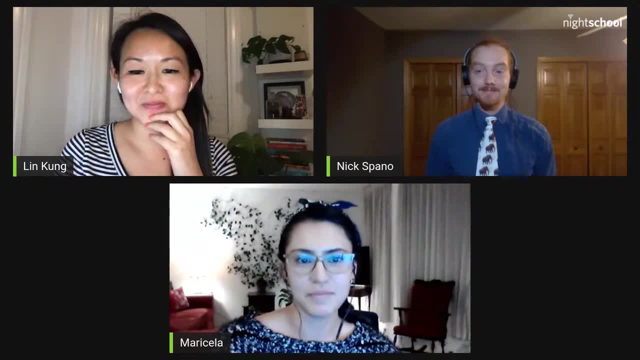 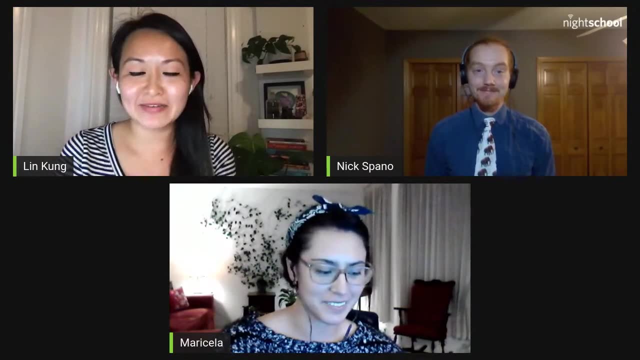 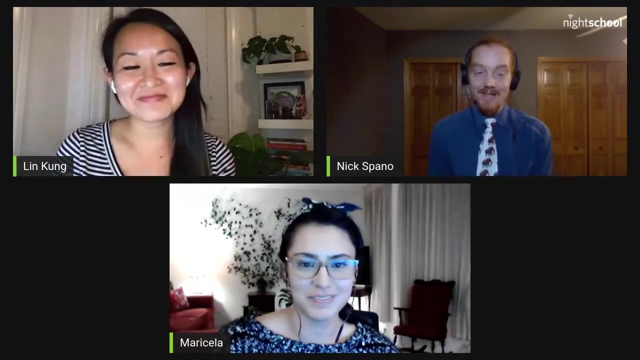 Cool. So if you want to become a fossil now you know, Yeah, Nick, why is everything so big in the Ice Age? Yes, That is an excellent question, And I cut out those slides In the interest of time, But two possible reasons that I'll touch on now. 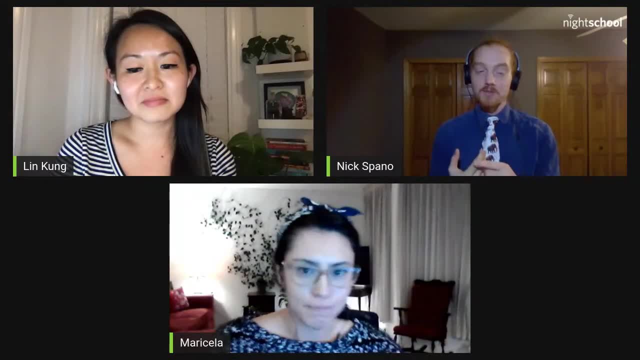 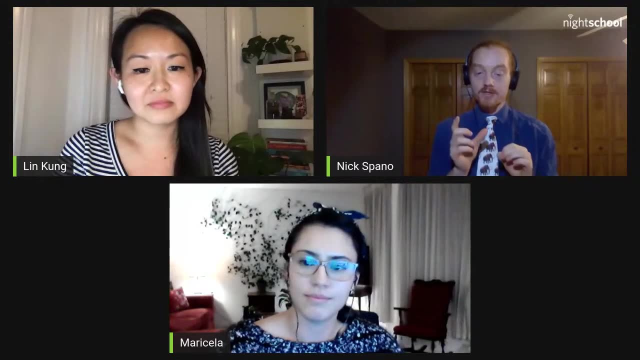 One is this idea of Cope's rule, Which was named after a paleontologist who made this observation- that groups on the tree of life In particular- he was looking at horses, for example, But it may also hold true for dinosaurs. Tend to get bigger through time, And so there are some advantages to being bigger through time, That is, you are much less likely to be bullied around, predated upon. You are much more likely to be a better bully And fight off potential competitors. 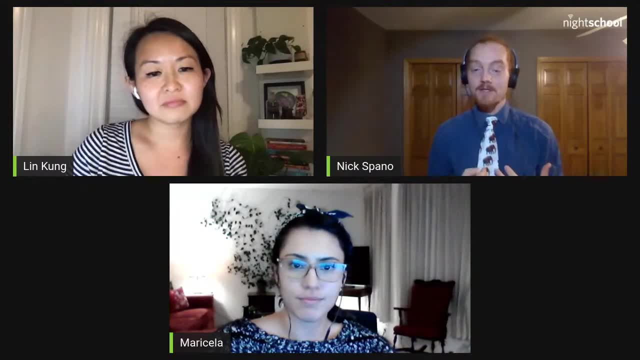 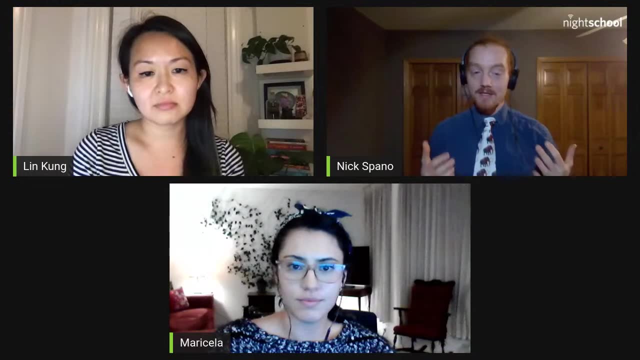 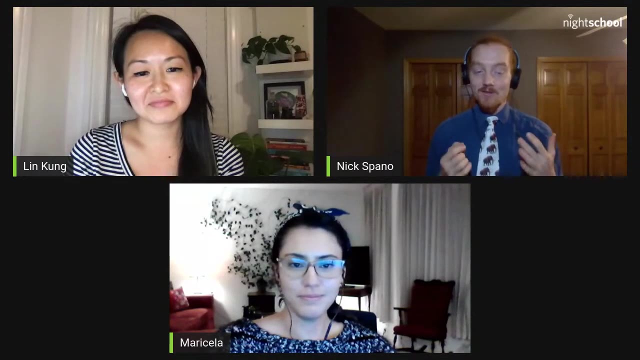 And you, in tough times, might be better able to deal with lean conditions. If you have more body mass, you can eat yourself in a way By metabolizing your tissues. But it turns out that might be more of a statistic, That might be more of a statistical artifact. 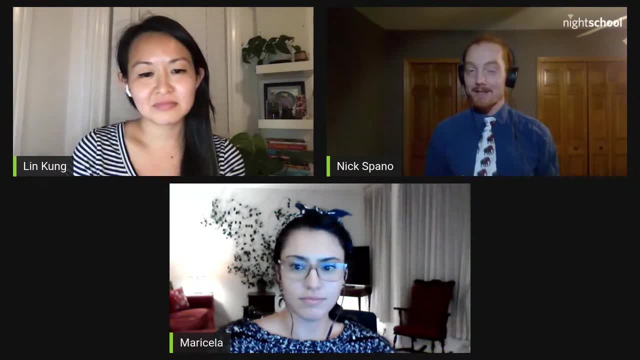 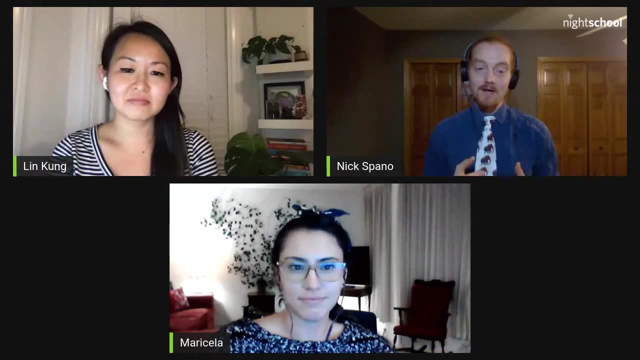 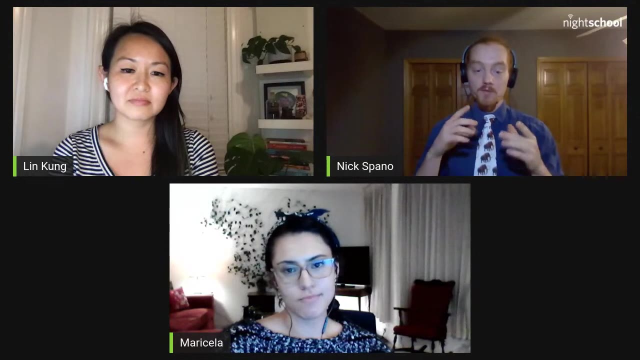 Of people really liking to find big things And finding bigger things. So another reason, especially when it comes to the ice ages, Is this idea of what's called Bergman's rule, Which is that because your volume grows at a cubic rate, And your surface area or your skin grows at a square rate. A given lineage is going to do much better in colder conditions And it's going to gain volume much more quickly than the game surface area, And so it will be much harder to lose heat in colder conditions. 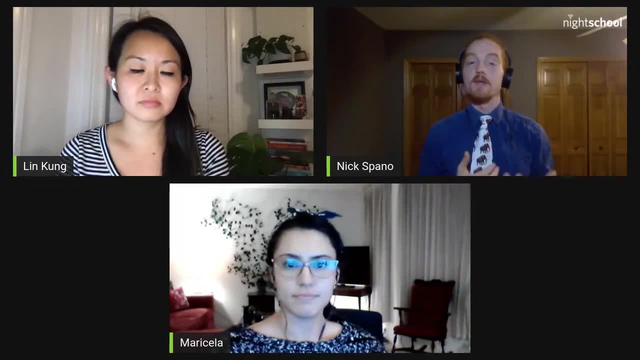 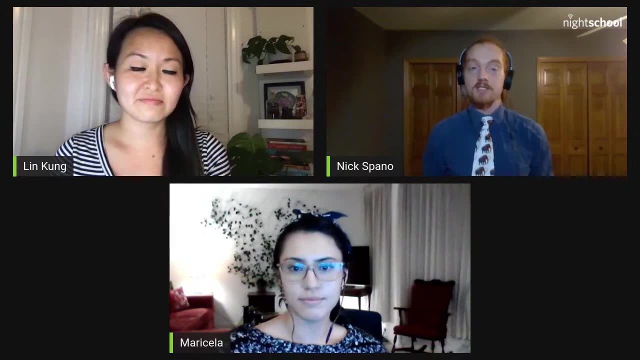 If you grow bigger And so it's thought that maybe with a cooling climate overall, That is why things got really really big. But there are other things like oxygen concentration That go into deeper time that play into it as well. Cool. 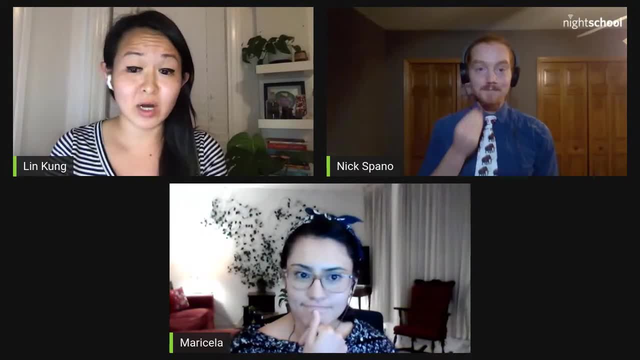 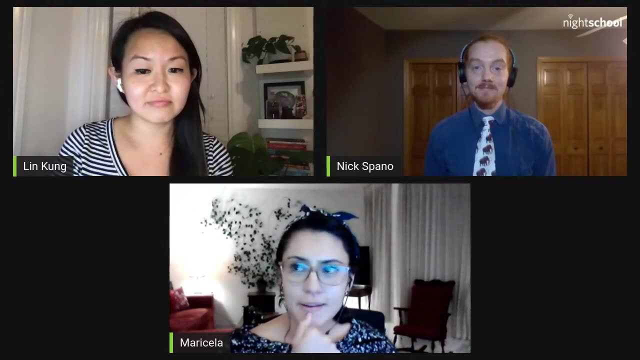 Maricela, you showed a CT scan of a wasp in amber earlier. What kind of data and stories can that tell you? It can tell you about what the setting at that time and place was. So that wasp was found in Baltic amber. 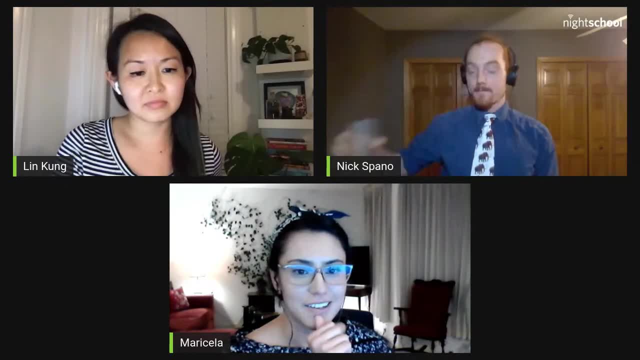 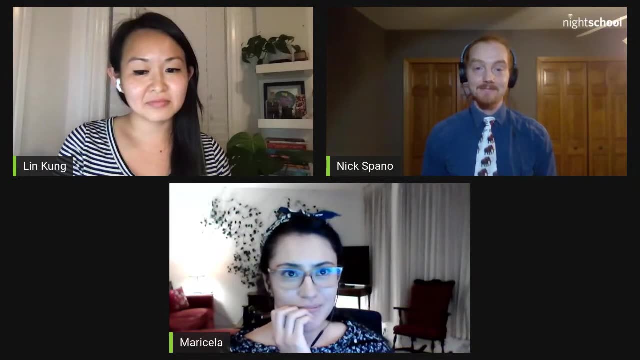 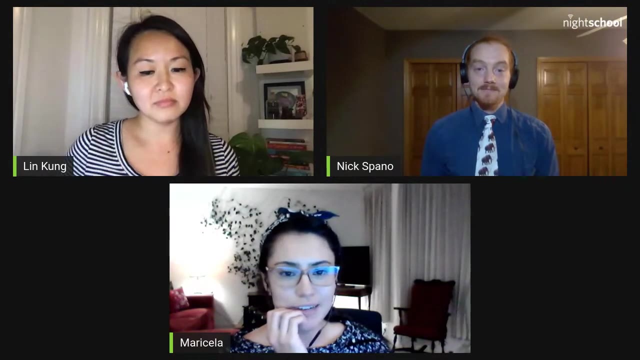 And the Baltic Sea right now is not the most forested place in the world. I don't think It's really cold, Yeah, But since amber is just fossilized tree resin, It tells you a little bit about the environment Back then. 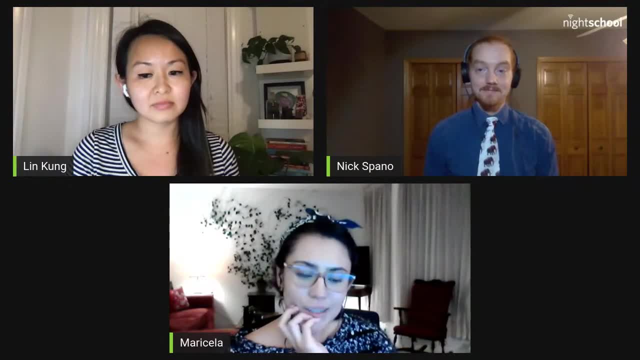 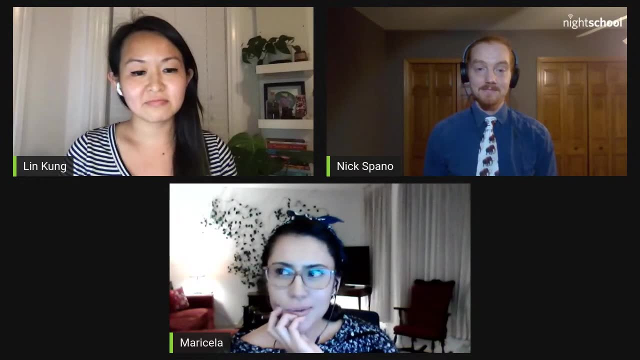 It can tell you, based on what's trapped inside, What kind of animals were living there. There is like a really cool Piece of an ammonite trapped in amber That was published in a paper a couple years ago, So I can kind of tell you. 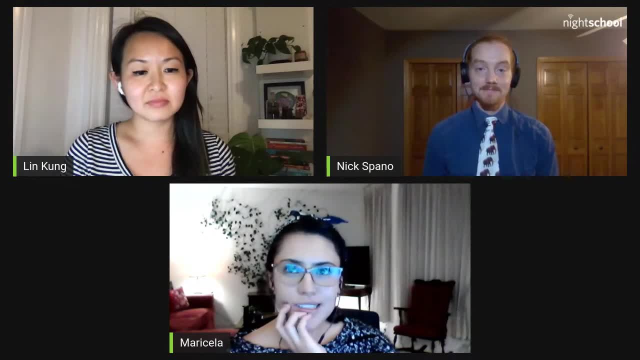 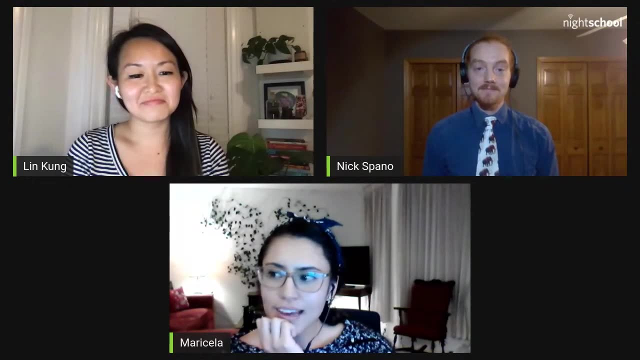 About the ecosystem too, because there can be more than one thing trapped in a piece of amber as well, Yeah, And just it can help like fill in the fossil record too A lot of like soft body things that don't Get fossilized as easily. 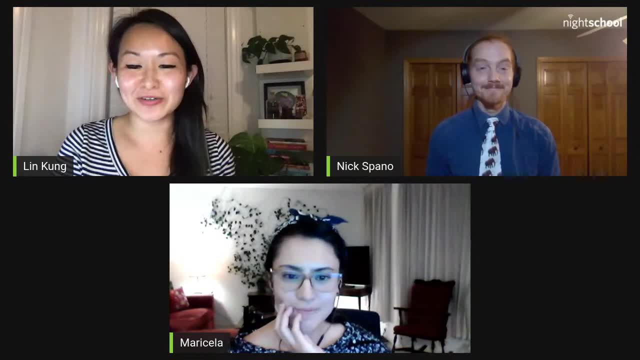 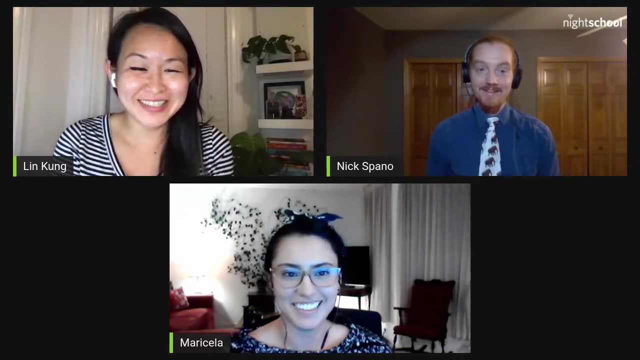 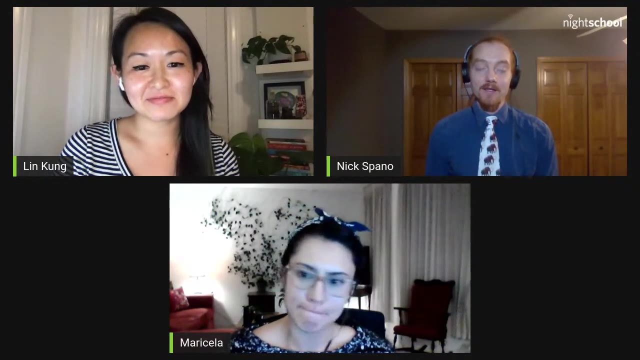 Nick, I'm just going back and forth. Nick, You showed An image earlier of a fully rhino And we just want to know more. Okay, Yeah, So woolly rhinos, We're a Species of rat? No, I think. 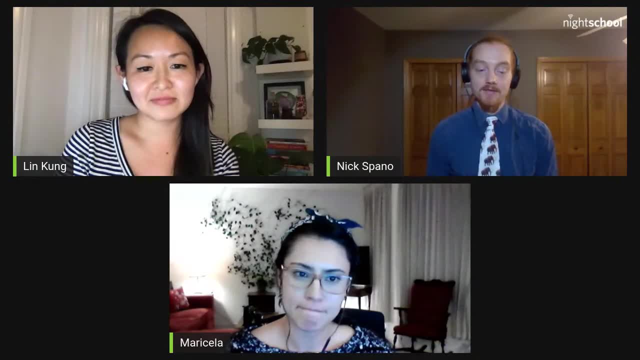 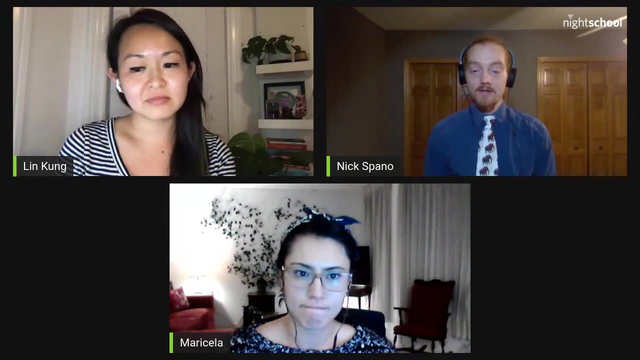 I'm done, My head is sealed. Dante and tickets. But they were alive throughout Europe And Asia And Russia into Mongolia and China. There was even Woolly rhino That was just Excavated and found in some permafrost. 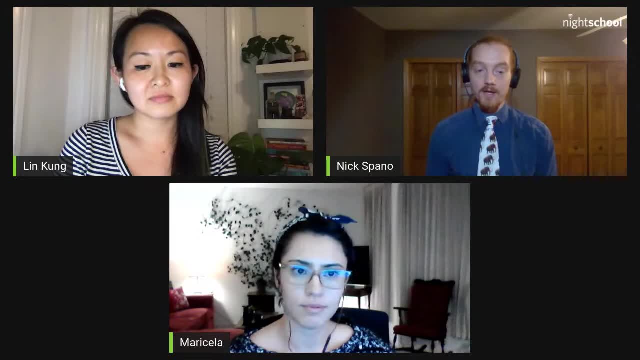 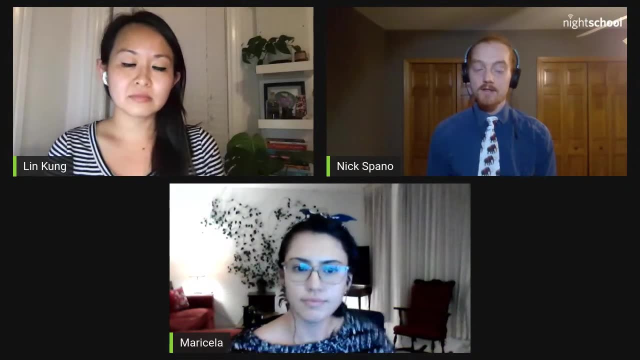 Pretty recently too, And they were around Until about, Yeah, 40,, 30.. Somewhere between 40 and 20,000 years ago, I think off the top of my head And yeah, it's not that just like. Woolly mammoths. They had a lot of fur. That was a really good adaptation in living in very cold places. It's a really interesting point That woolly rhinos never. There are a lot of things That crossed over from Russia to Alaska. 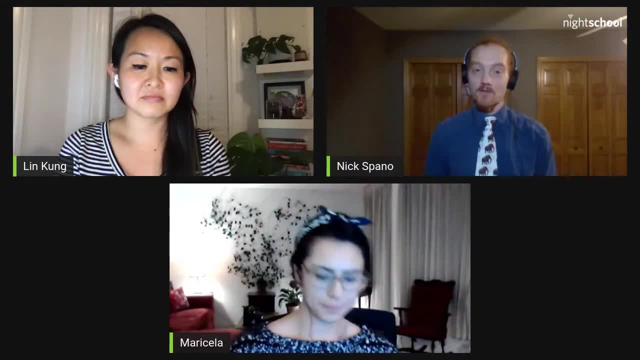 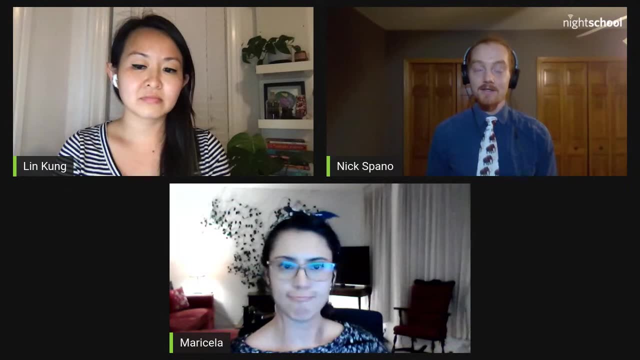 When sea level was much lower. but woolly rhinos were not one of those things And I haven't looked that much into why, but I know that's been a question in paleontology. There were At least three other species of non woolly rhino in Europe. 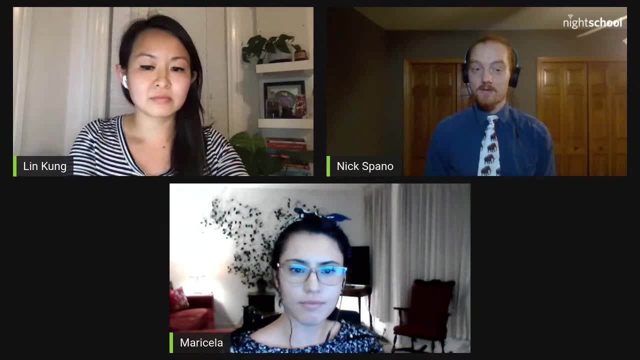 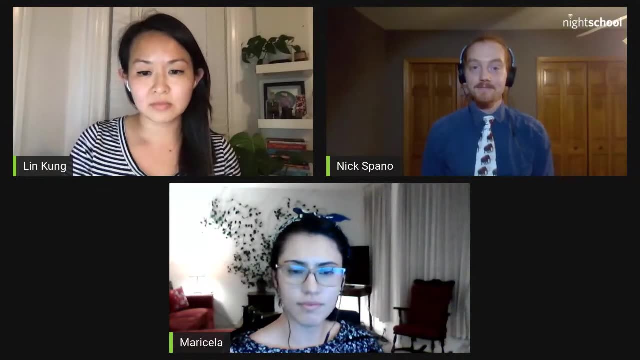 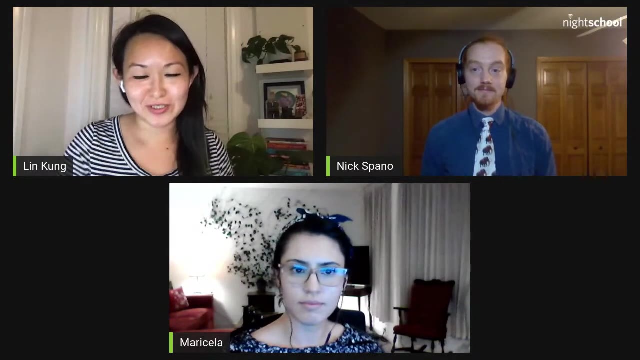 During what's called the last interglacial, about 130,000 years ago, Along with Woolly rhinos, Which is very cool. I think we have time for one more question, So I'm going to ask you both this. 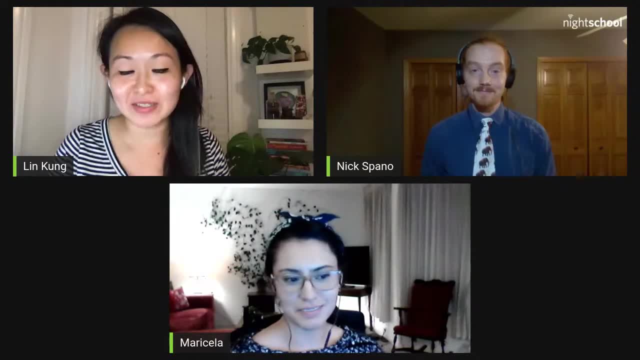 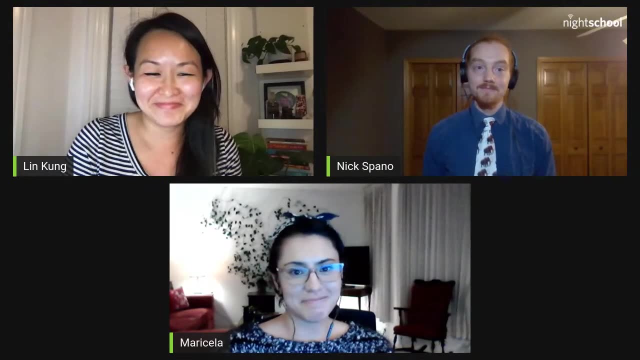 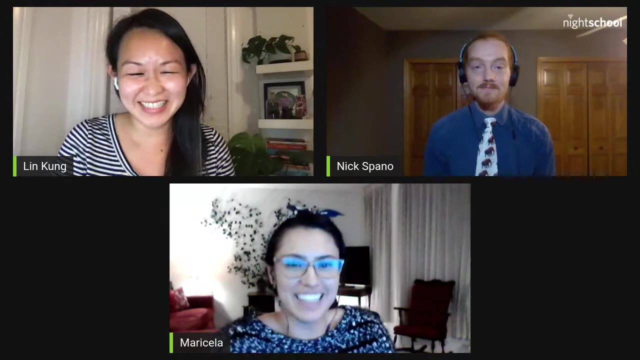 What is the most concise thing you can say to someone who is on the fence about the fact of climate change? Being concise is not my Strength, But I think I would just try to hammer in the fact that The climate change that we're experiencing now is happening really fast and really rapid. 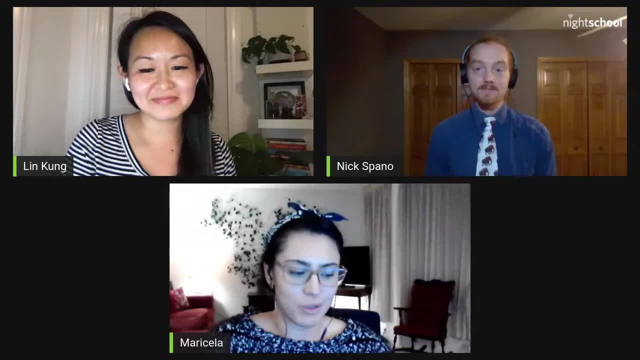 And A lot of people are like: well, the climate's been changing, And I think in both of our presentations: Yeah, The climate is changing, but now we're we've just accelerated It so fast that that that's what's concerning now. 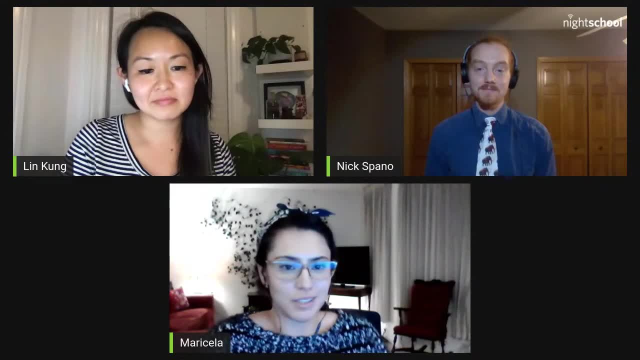 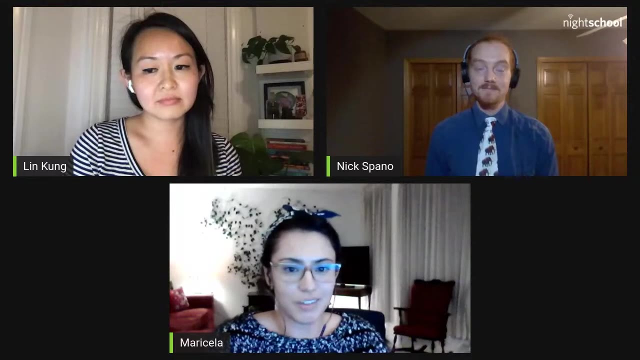 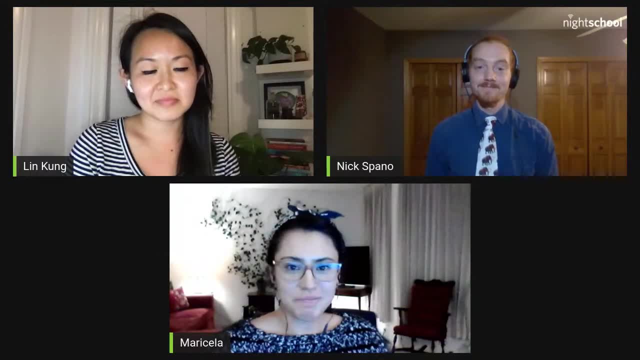 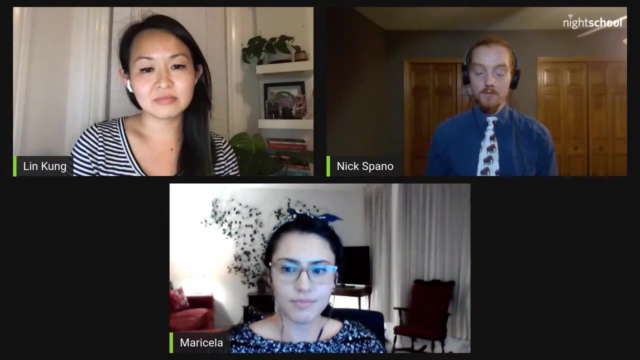 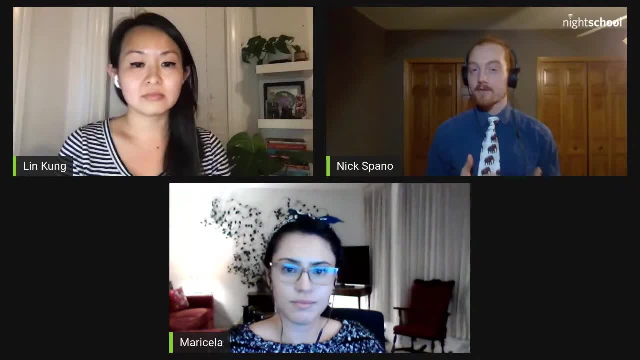 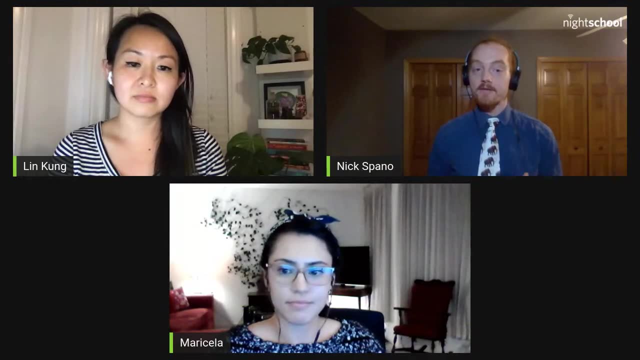 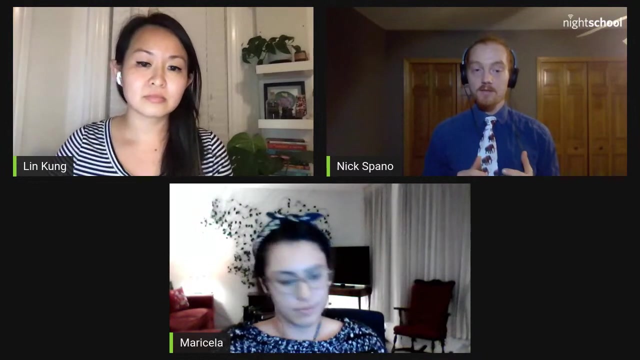 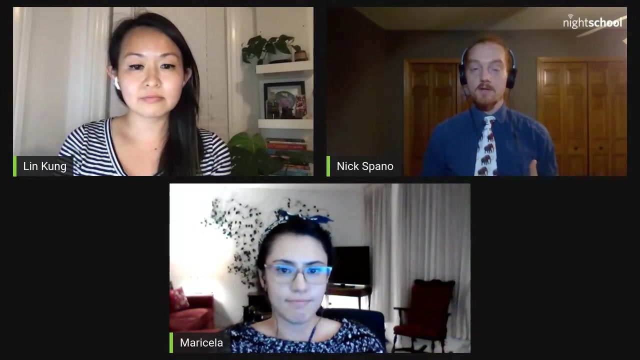 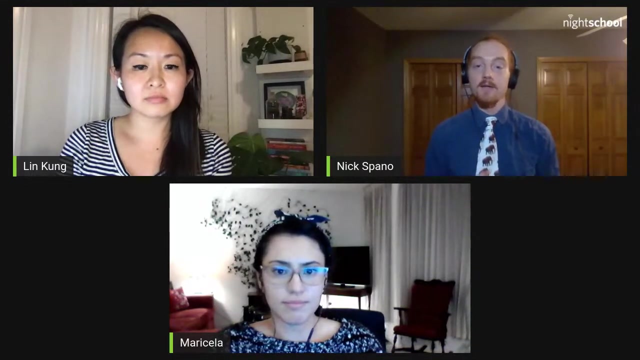 conversation with somebody who hold that belief, to really just start with the question of Not And really get at this question of where they're coming from and where they're getting their information from. to really have that conversation with them And- although the evidence behind climate change and the human cause nature of it is very solid and sound, to be able to figure out where this person is coming from and really have some dialogue so that they don't feel like you're just shutting them down and you know they can go forward in the world, really feeling like 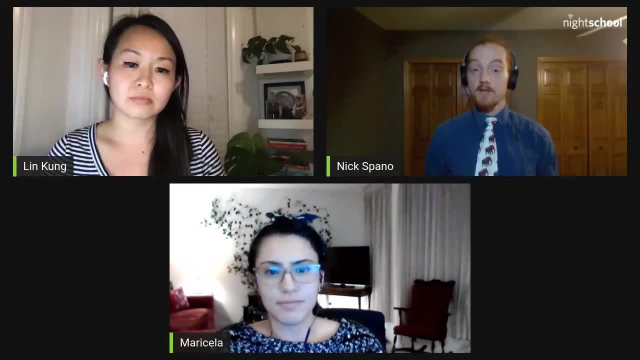 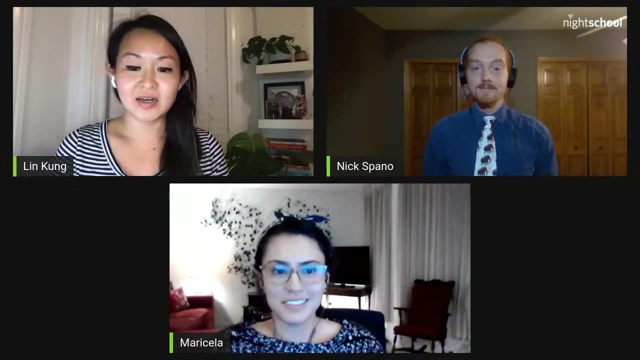 oh, this person who knows things about climate change wasn't a jerk to me is really important too, even if you don't say: change their mind. Yeah, Good advice. I think that's all the time we have for Q&A. 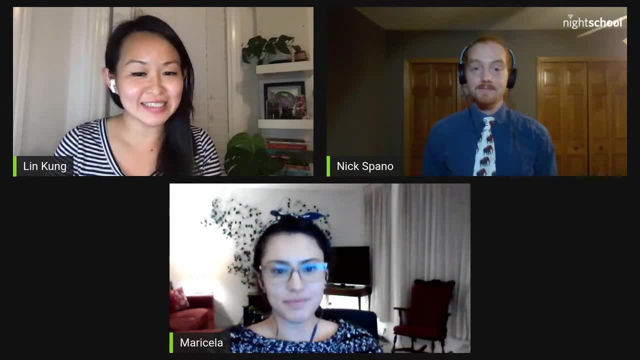 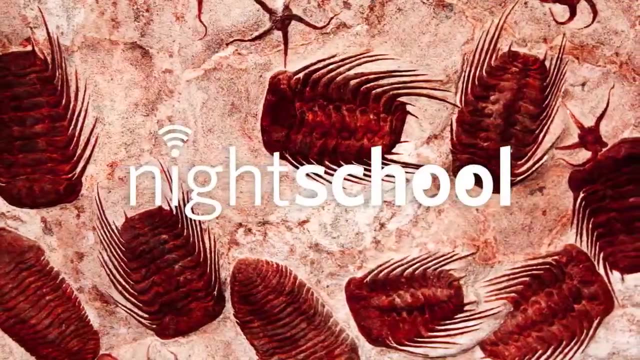 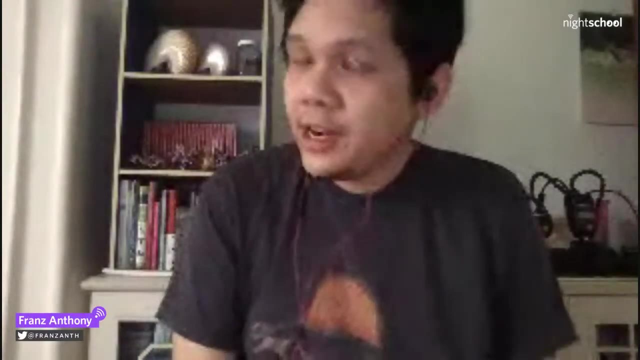 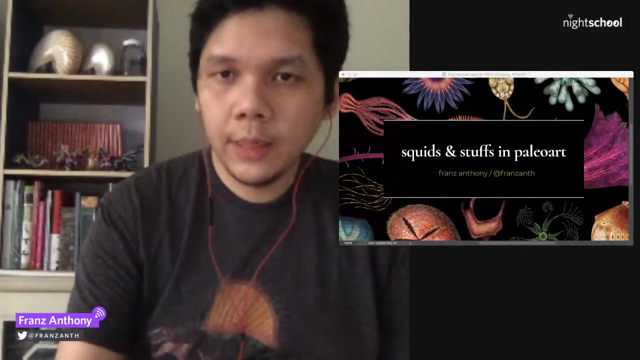 Thank you, Maricela and Nick, for joining us tonight. Next up we have illustrator Franz Anthony. All right, Hello, And good evening everyone, or morning if you live in my part of the world, Okay, Okay, my screen is shared. 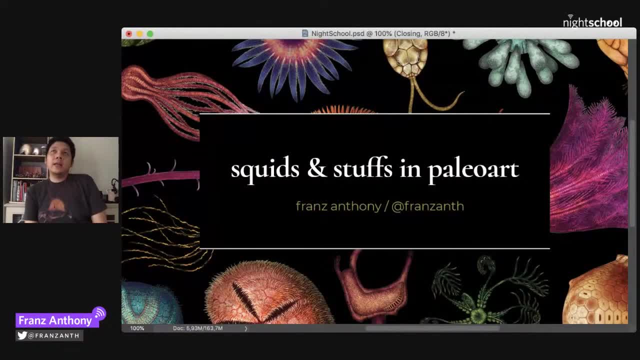 So my name is Franz and I do paleo art And, if you're new to anything, paleontology- paleo art is basically a branch of art or illustration where we try to recreate what life would have looked like in the past. So I think I was in and out during Maricela's talk but I saw that she showed a lot of really cool fossils, but you know that fossils are basically rocks. 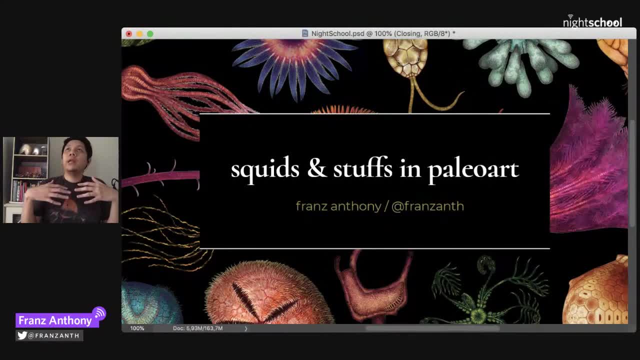 So if you want to figure out what the animals look like in life and present them to the general public, you need someone like an artist to recreate that kind of life, to make it more presentable, to make the people understand what the animal looked like and how it looked like. 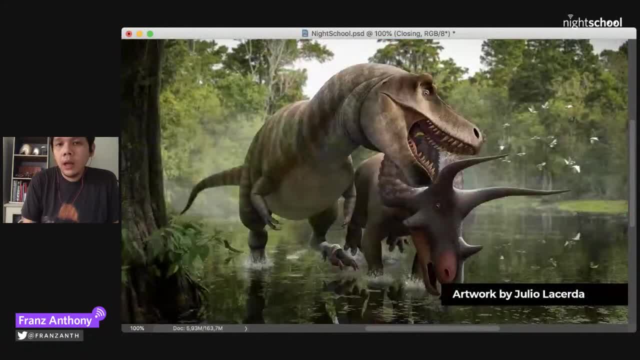 How they behaved. So when I talk about paleo art, most people would think about dinosaurs, because of course they're really iconic. They're amazing. There's no doubt about it. There's a lot more than dinosaurs in paleo and paleontology in general. 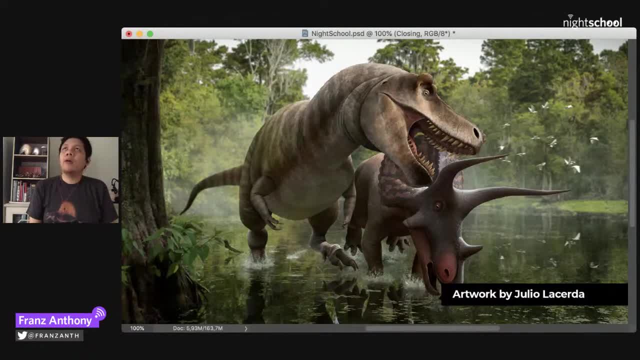 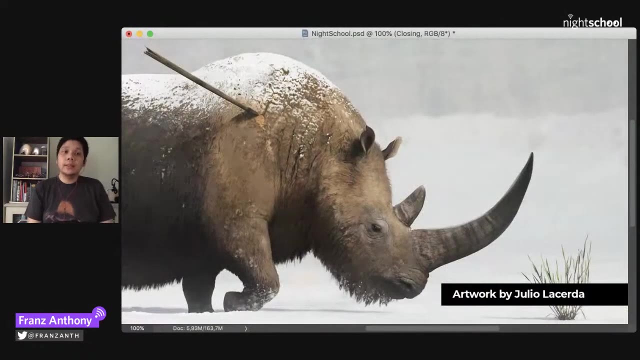 Like Maricela talked about earlier, life has been around for well complex life has been around for 500-something million years, Right? So there's been a lot of things that lived and died a while ago. So, for example, like the mammals that Nick and Maricela loved. 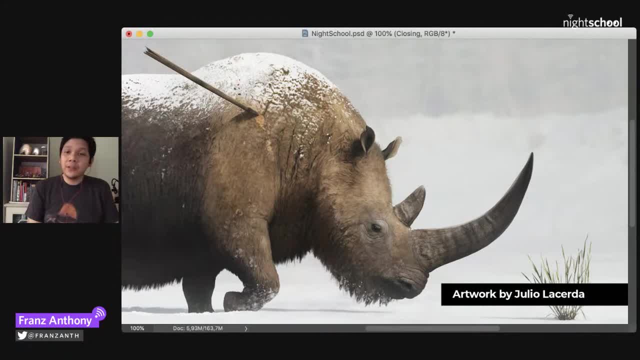 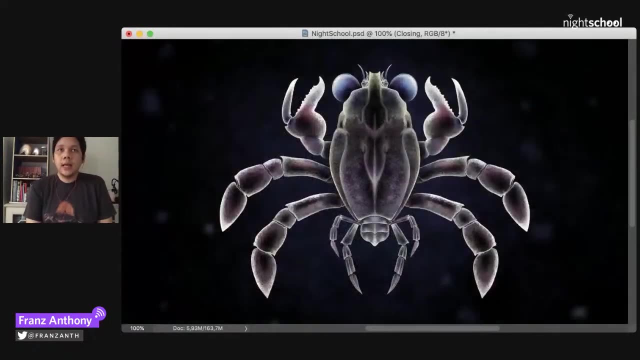 But I personally don't specialize in dinosaurs or mammals, so I borrowed these images from my friend Julio. You need to follow him if you're into dinosaurs and mammals. He's really amazing. You just look up his name. So I personally prefer to specialize in invertebrates because I feel like there's a lot of 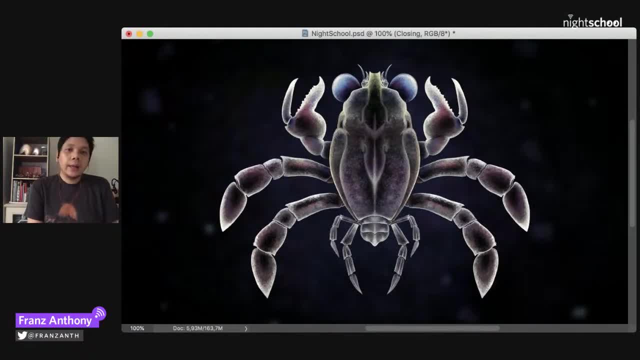 So I personally prefer to specialize in invertebrates, because I feel like there's a lot of animals that people don't pay attention to, like this crab, for example. People don't think of crabs as being ancient creatures, but just so you know, crabs have been around since the Jurassic period at least. 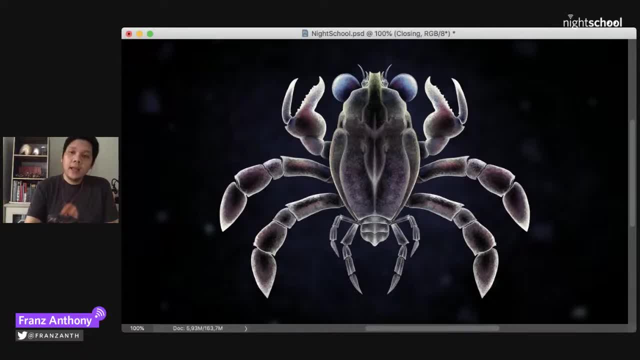 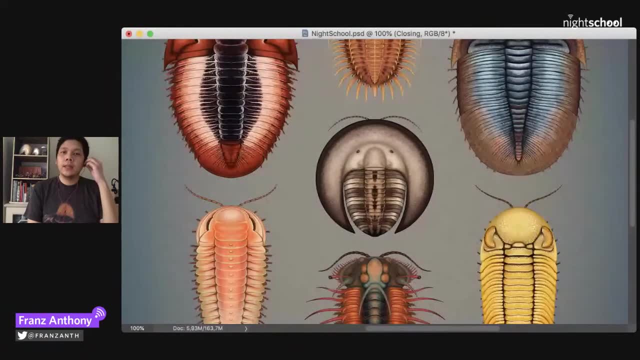 So the oldest crab is older than the Rex, And there are also things that more people are probably more or less familiar about. These are trilobites. These are trilobites which are mostly found as black or maybe brown rocks. 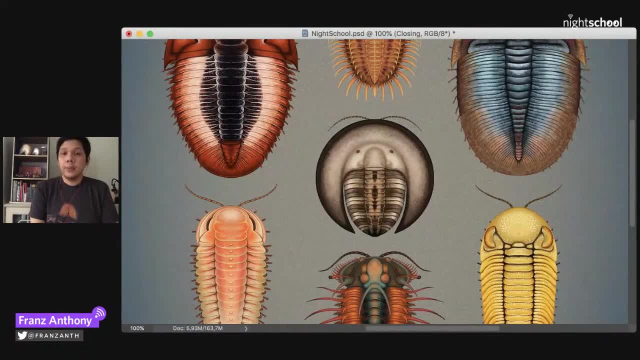 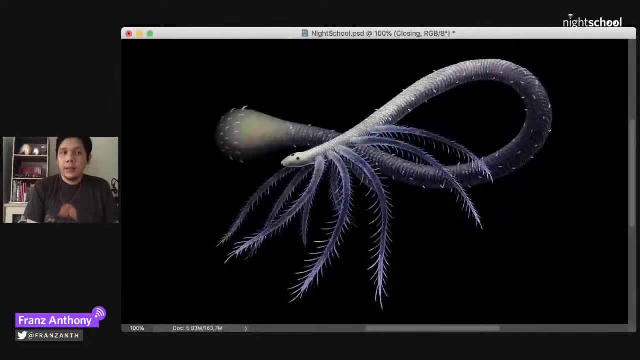 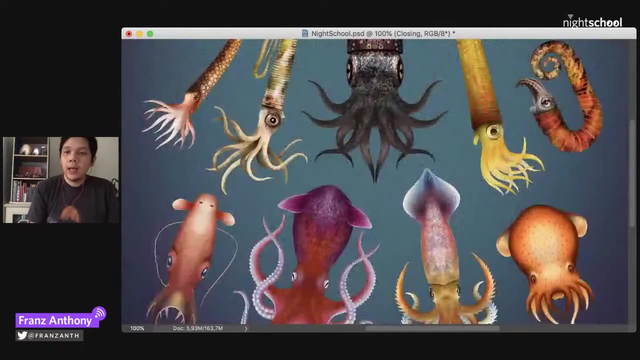 And it is an artist's job to recreate these animals so that people could probably guess what they look like in life. And there are also things that don't resemble any living things that we see today, like this worm, for example. But today I'll mostly be talking about pteropods, because apparently that's what people love. 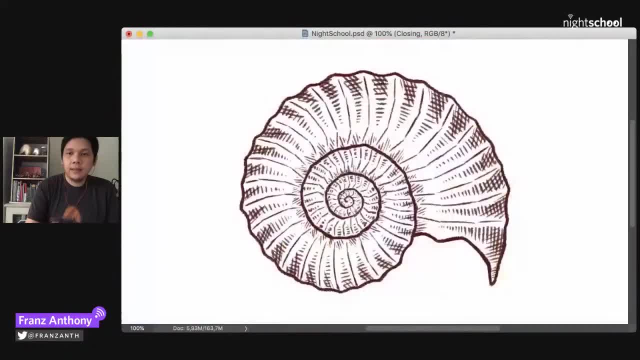 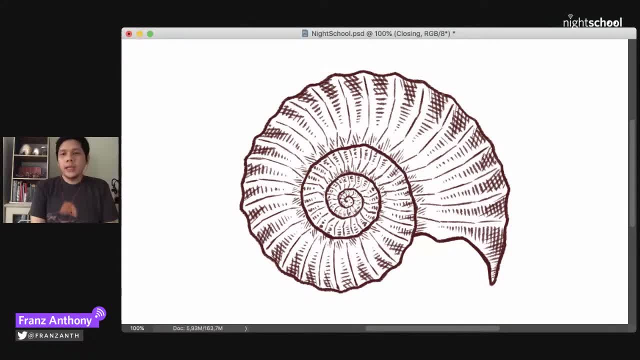 So let's say, you found a fossil ammonite. I saw that Maricela shared some ammonite photos earlier. There are actually so many different species of ammonites that come in different shapes, But since it's a little bit too much for this talk, so I'm just going to simplify and call everything the ammonite, because I don't have much time. 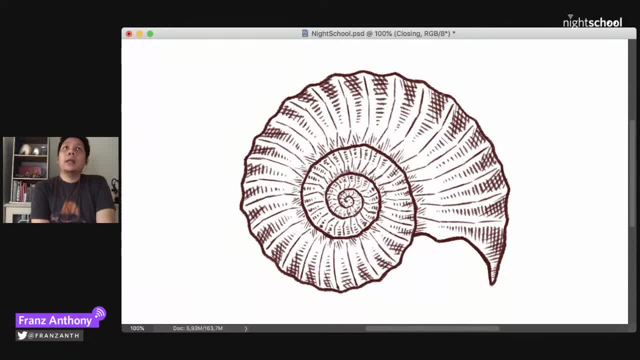 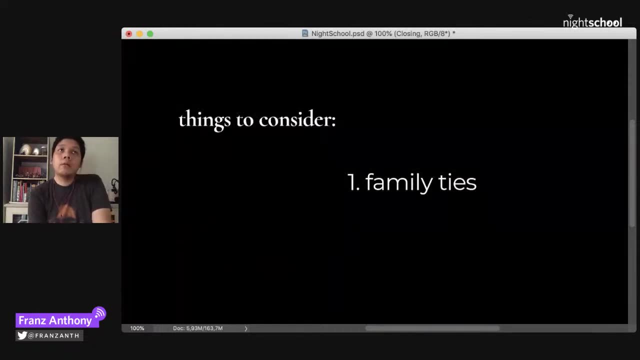 So if you, Let's say, you have an anemone, how do you think the animal would look like in life? There are a few things to consider when you try to recreate an animal's life appearance. The first one is what the animals are related to. 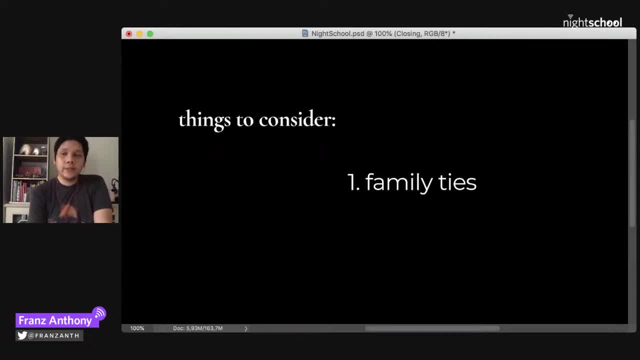 You know, you need to figure out what its closest living relatives are, And since most people are probably not familiar with cephalopods because they live in the oceans, I'm going to give you an example that most people are probably going to be more. 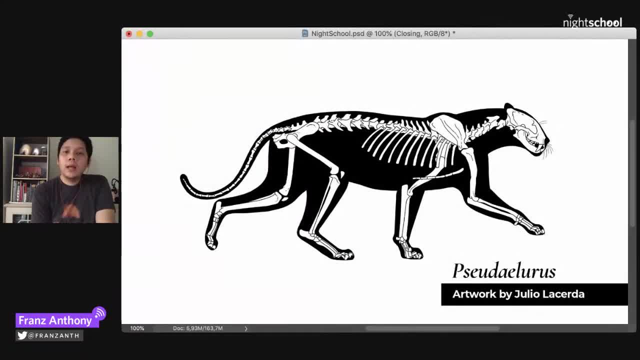 familiar with This cat, for example. You probably have one at home, so you know what a cat looks like in real life. But if you found the bones of this cat, for example, you probably wouldn't think right away that it's a cat. 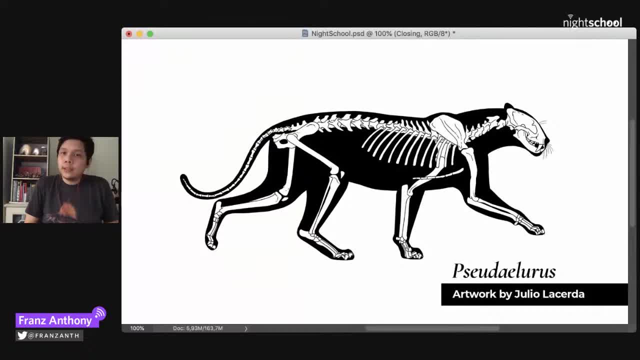 But if you look closer, for example, if you look at the face, maybe the fangs, the body shape, the tail- You could probably tell that it's some kind of a cat. but you don't know what it would look like in life. 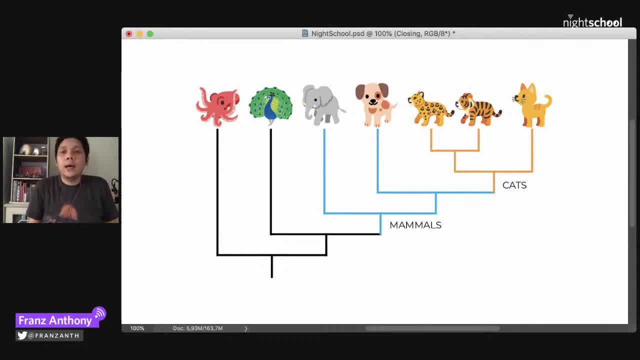 So this is where we need to look at the relationships between animals. Artists and paleontologists in general use a technique called phylogenetic bracketing. So phylogeny is a study that focuses on- well, to put it simply, it's basically about the. making of the tree of life. So phylogeny is a study that focuses on- well. to put it simply, it's basically about the making of the tree of life. So phylogeny is a study that focuses on- well. to put it simply, it's basically about the making of the tree of life. 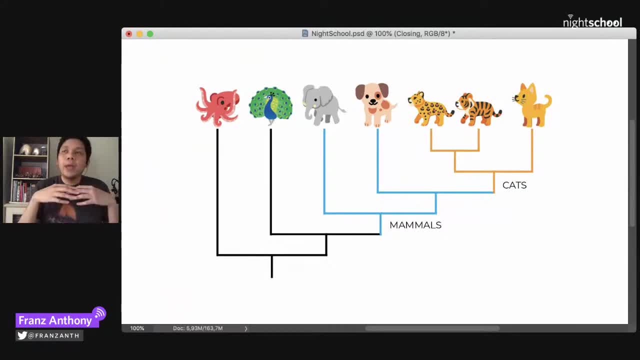 It's figuring out where things sit in the tree of life, And by bracketing it means we're looking at brackets of things that are related together. For example, we know that the animal earlier was a cat, So its living appearance would have probably looked like something in this area, in this. 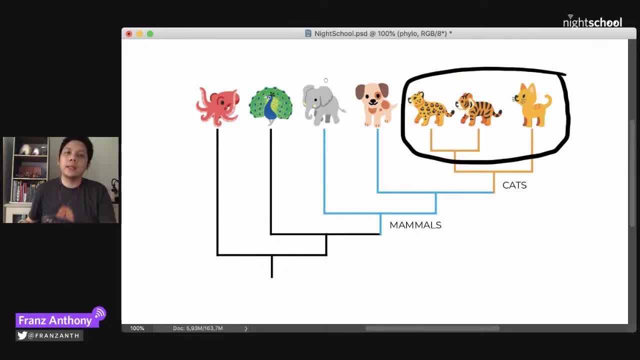 bracket and not like something like an elephant, for example. So if you want to, If you want to draw an extinct cat, you would probably think it's probably somewhere in the yellow-orange color range, or maybe it's going to be stripy black, something like that. 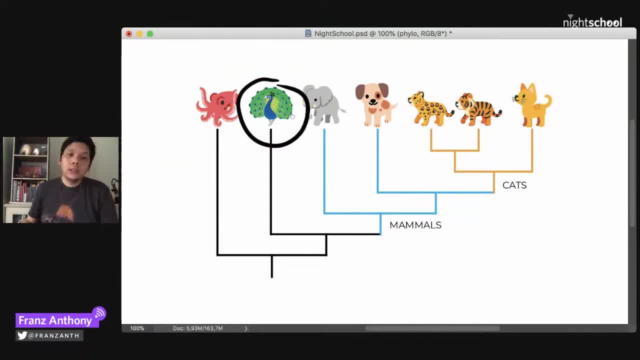 But it wouldn't be a bright green like a peacock is, or maybe a pink-purple like a nocropus? Well, because we don't see any living cats or maybe even mammals in general today that are green. Yeah, Another good example that I put here is the elephant. 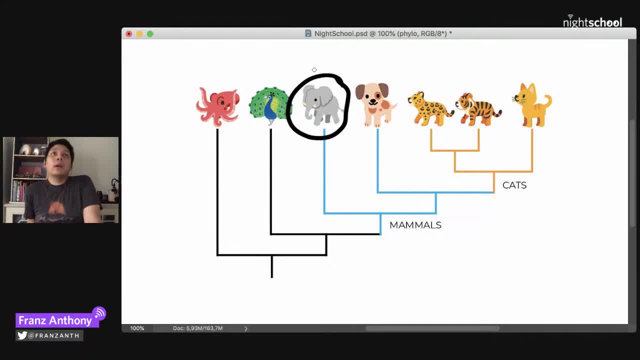 If you found the skull of an elephant or an elephant relative, like the mastodon, for example, you wouldn't be able to see the trunk or the ears, You would just see a big skull with a big hole in the front. But since you know that the bones closely resemble what you see today in living elephants. 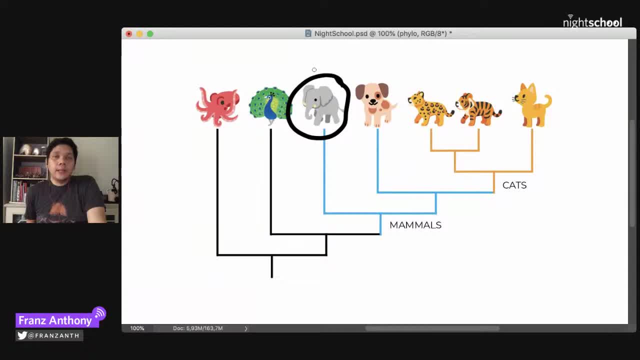 you know that it's going to be a creature that had a long trunk and tusks, and definitely it would have bigger ears than most other mammals. So that's what phylogenic bracketing is. So, using this principle, my friend Julio reconstructed some fossil cats. 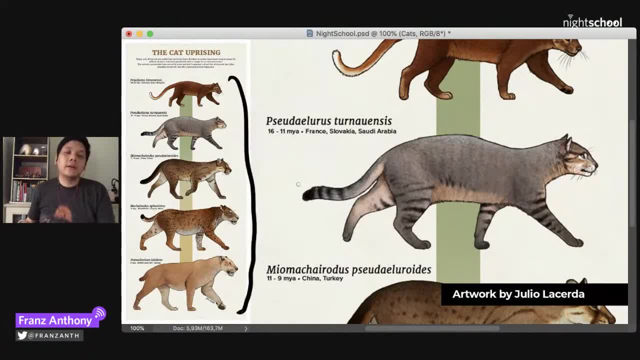 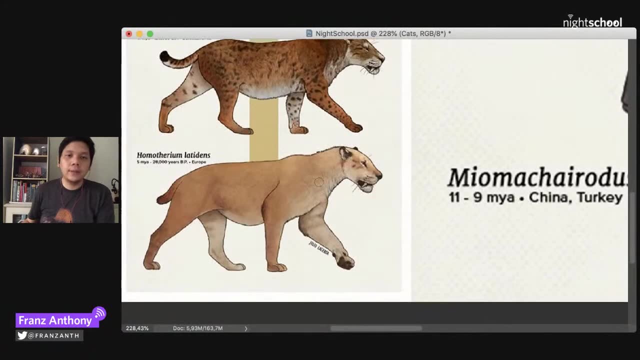 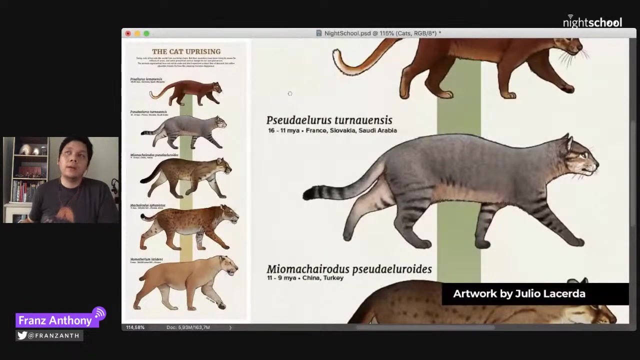 And you can see on the left here that fossil cats are well, probably somewhere in the brown-gray range And you could see it could probably be stripy, dotted, mottled, something like that, And you wouldn't even. These are cats that could possibly live today and you wouldn't even think that. 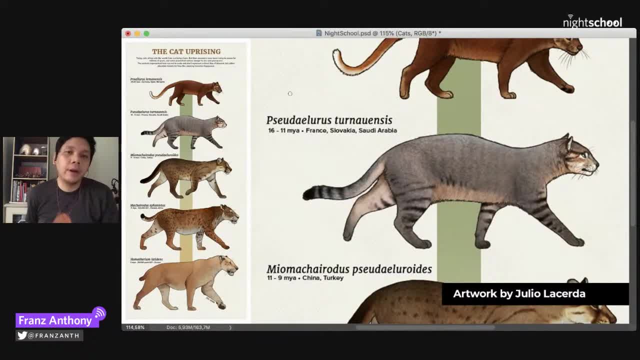 It's something weird because it's really possible. It might not be what the animal actually look like in life, but it's possible that they look like this, And this is the exact cat that we saw earlier as bones. So Julio reconstructed this cat as a gray cat with some stripes on the legs and so on. 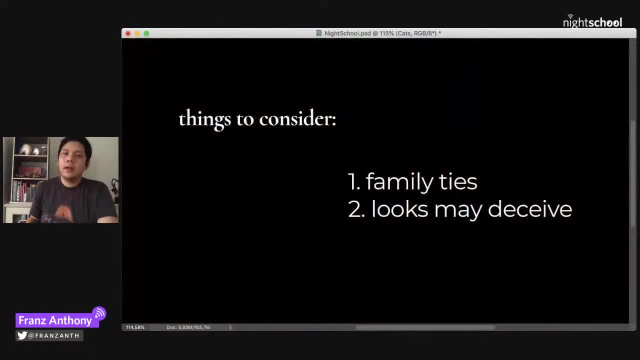 So there's another thing that we need to consider. The second one is that just because something looks similar doesn't mean that they're actually related. So let's say, you and someone else are wearing the same clothes And the same cat is wearing the same clothes. 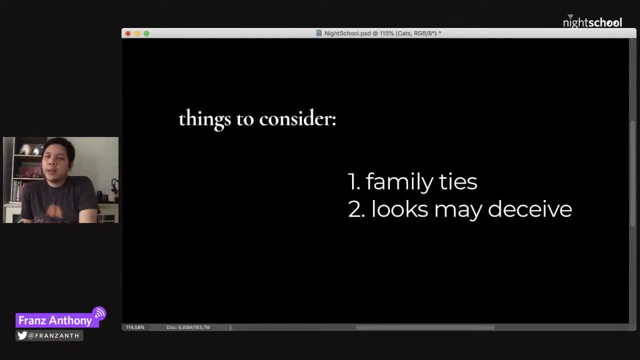 And the same cat is wearing the same clothes. The same cat is wearing the same clothes. The same cat is wearing the same clothes. And the second one is: if you have the same hairstyle, it doesn't mean that you are siblings or even family, because there are things that can easily change more than other things. 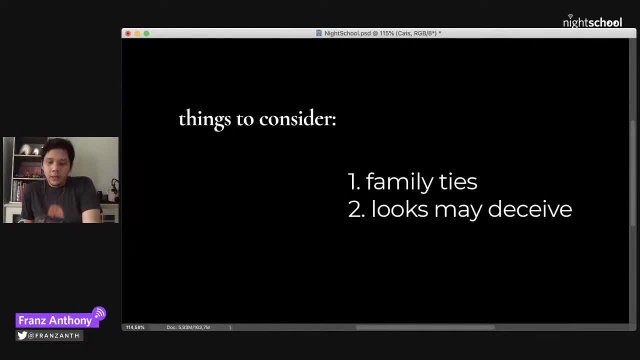 So you could probably, if you're trying to identify people's family relationships, you would probably look at things like their bone structure, their height maybe, or maybe their skin color, because it could indicate their relationships better than something like their hairstyle and so on. 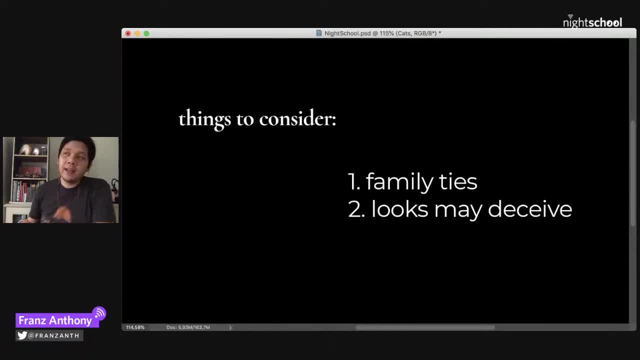 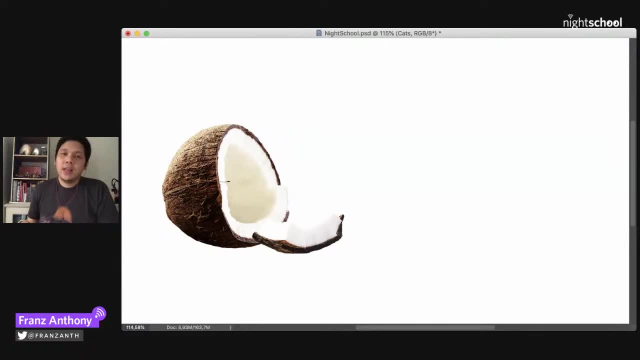 So another. this is an extreme example, but a funny thing that has been floating around the internet is: let's say you consider a coconut. You know that a coconut is hairy and milky on the inside, But would that make a coconut a mammal? 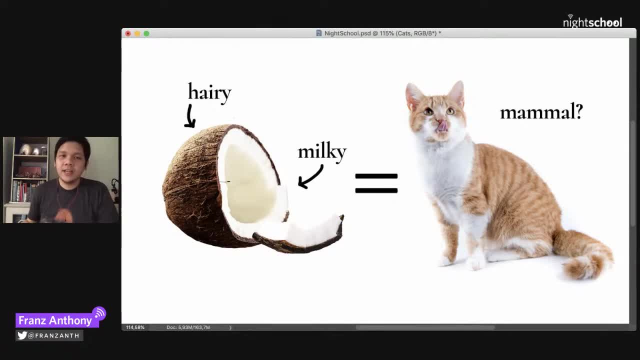 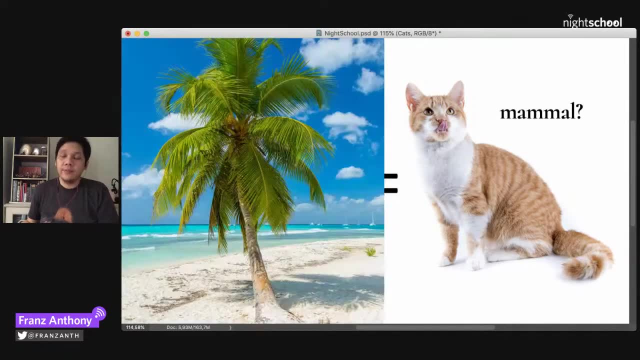 Like a cat. It's brown, sure, it's hairy and it's milky, But if you look at things in general context, you know that a coconut comes from a tree and cats came from kittens. So no, they're not actually related. 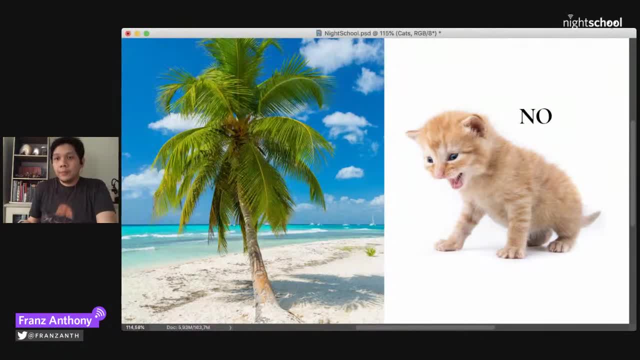 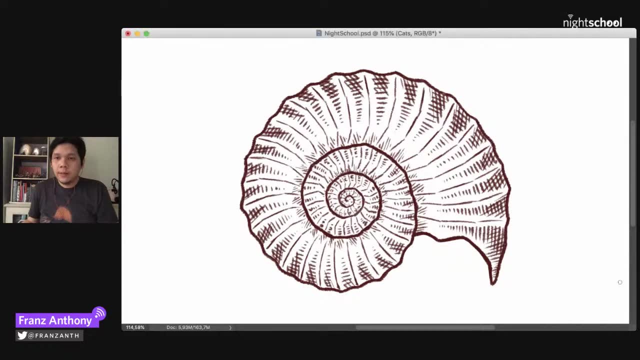 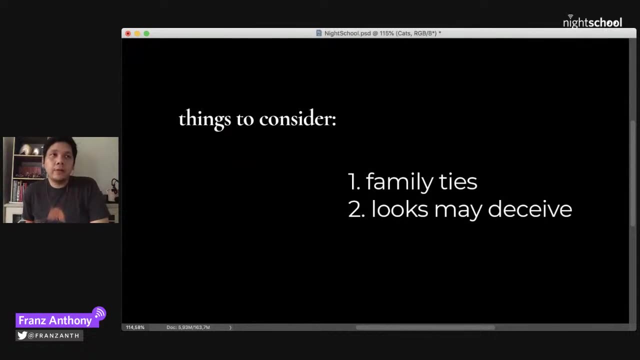 So, using this principle, we could roughly guess what our friend, the ammonite here, would have possibly looked like in life. So, just as a reminder, we're going to talk about the ammonite here. First we need to figure out the family ties. 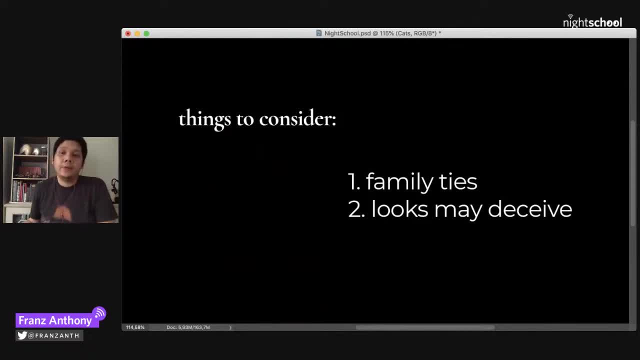 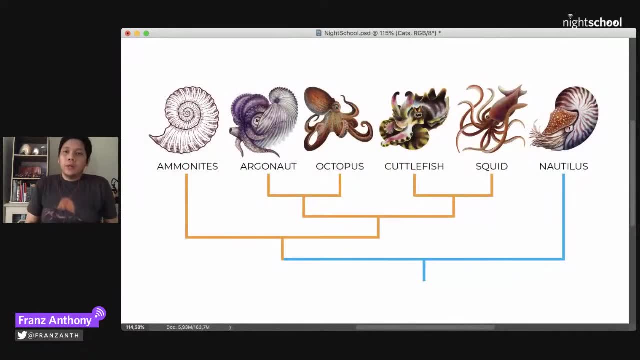 but we also need to remember that looks may deceive you, So things that look similar may not actually be related. So this is the family tree of the cephalopods. As you can see here, people are probably going to be most familiar with the octopus and the squid. 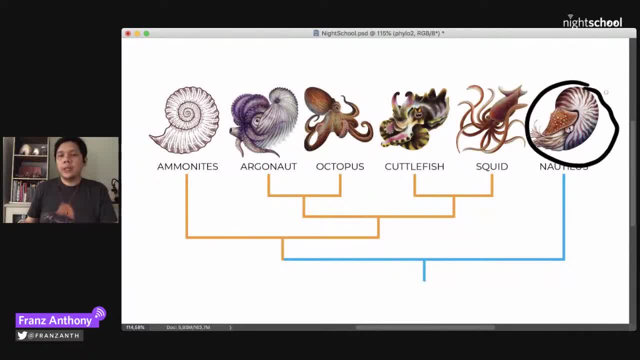 But there's also the nautilus. that is probably pretty iconic because it looks ancient, but it's the only true shell cephalopods, at least today. But there's also the arconaut that most people are not really familiar with. Its other name is the paper nautilus. 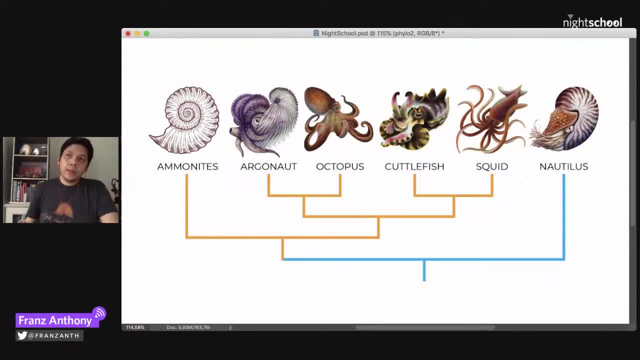 and it looks shell, But if you look closer it's not actually related to the nautilus, because deep inside it is actually just a nautilus with a shell that it can detach. But if you try to detach the nautilus shell it's going to die. 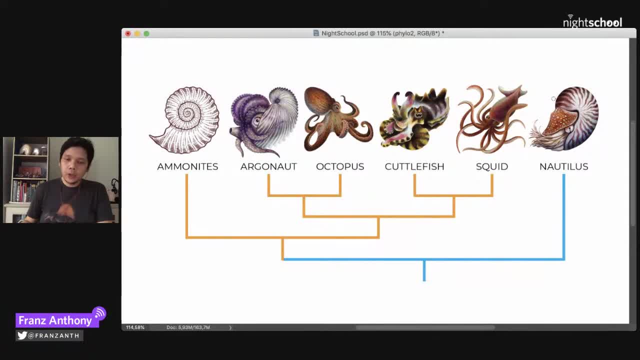 because the body is anchored to the shell closer to something like a snail, for example. It's just so anchored. By the time you try to detach it it's going to die. But the arconaut is basically just an octopus with a shell. 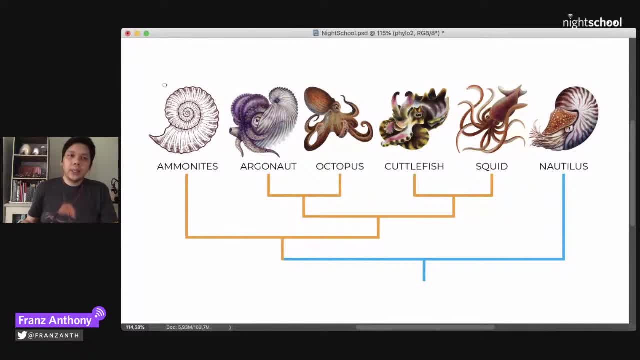 And I'm not going to go too deep into the science, but the ammonites, despite their hard shell, are not actually related to the nautilus, But they are based on the internal anatomy of the ammonites. They're actually more closely related to the squishier part of the cephalopod tree. 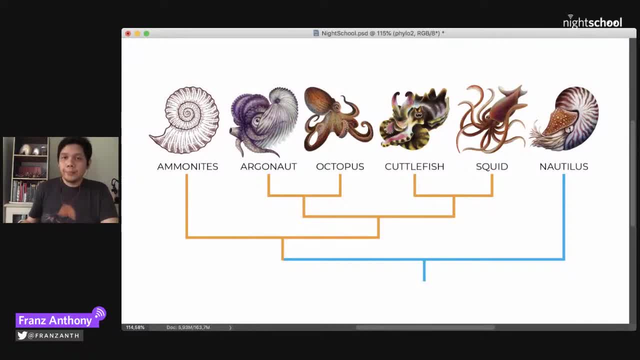 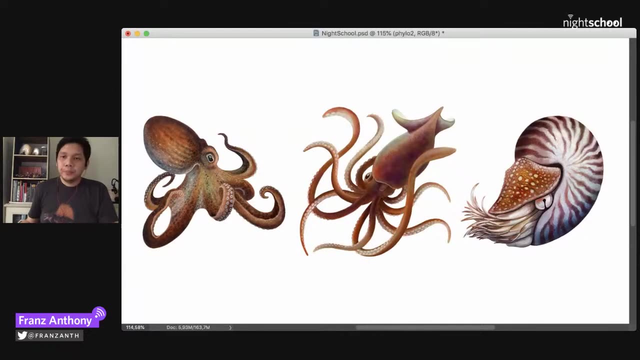 So, using this knowledge, we could probably compare the features that our squishy cephalopods have, So we can probably figure out what kind of a body shape the ammonites would look like. So, for example, these are the most commonly seen body shapes of cephalopods we see today. 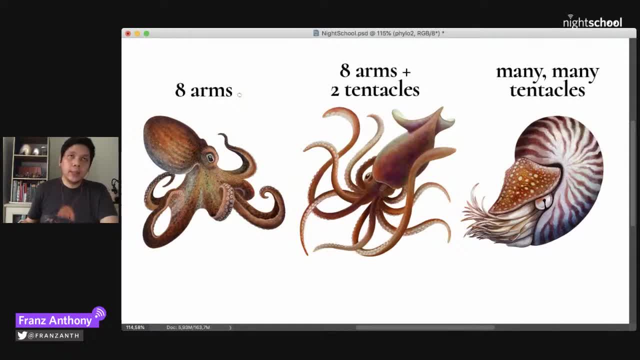 And we see that the octopus, like its name suggests, has eight arms. What people usually call tentacles are technically called arms. It's mostly to distinguish its appendages from what people call tentacles in squid. So basically, arms is the thicker ones, the main ones, and tentacles are in squid and cuttlefish. 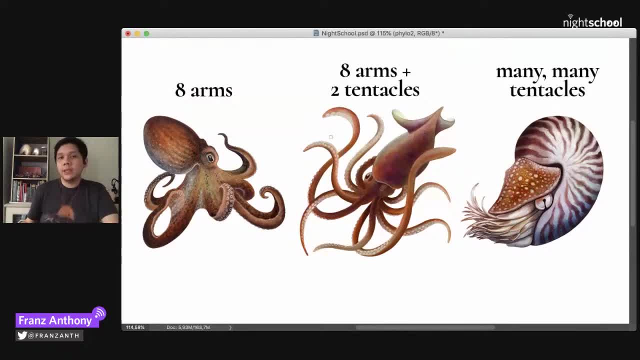 they're usually longer and they might or may not have clubs in the end, But the nautilus has many, many tentacles, little tentacles. It could range between 60 to 90, I believe. So it's a really big difference from 8,, 10,. 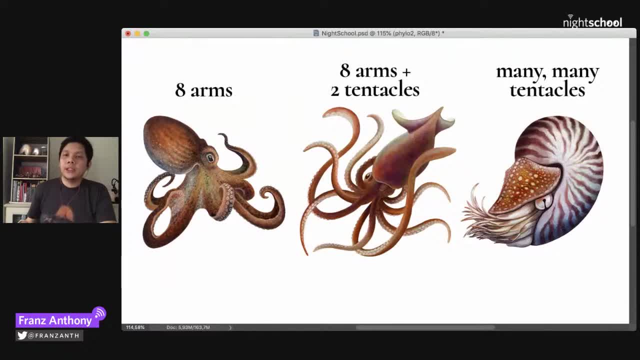 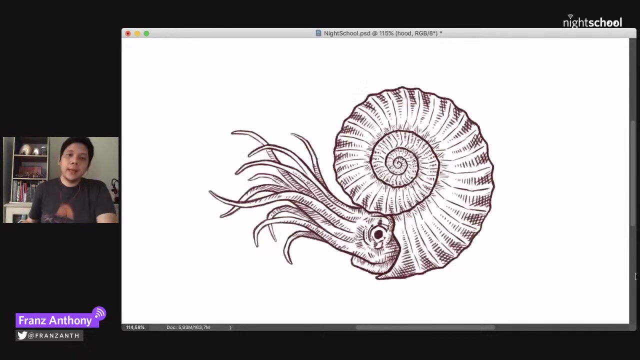 and then 60 to 90.. Because it shows how actually distantly related they are. And the last thing about nautilus is that it has this really really cool hood, This one here. So if you apply that knowledge to our friend the ammonite, we could say that the ammonite 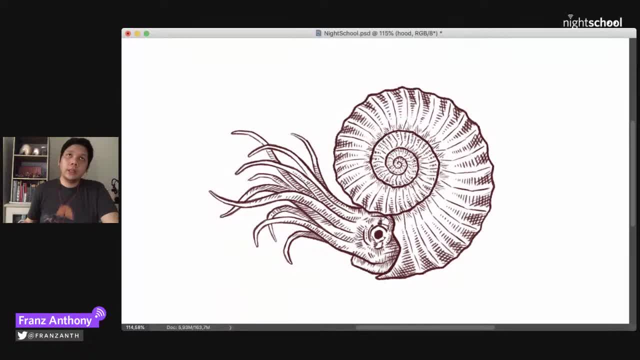 since it's more closely related to squid than the octopus, it's more likely that it would have 10 arms, because apparently a lot of extinct cephalopods have 10 arms And it seems like the octopus just reduced their arm count later on. 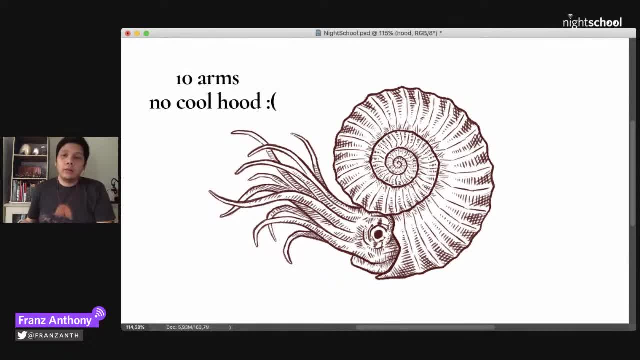 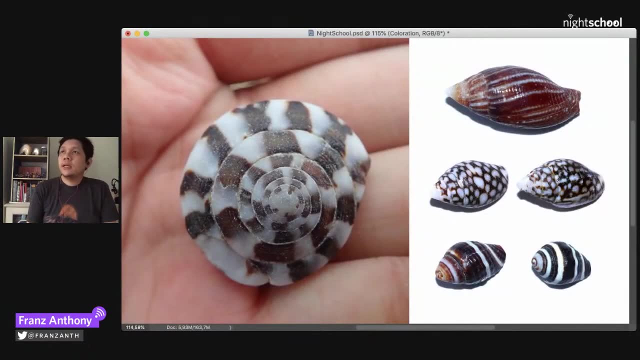 And the ammonite is not likely to have the cool hood that the nautilus have. So now that we know what the body looks like in life, we could start talking about the coloration. The problem is, as I said earlier, the nautilus is the only true-shelled cephalopod that lives today. 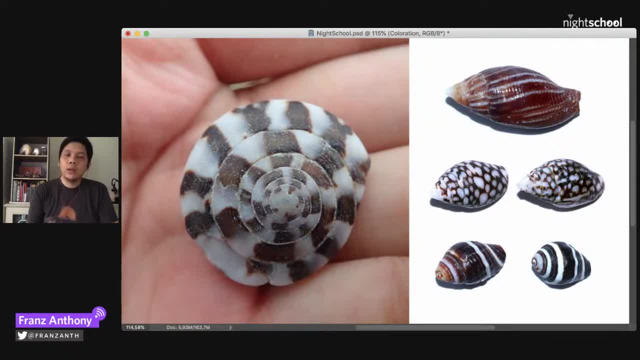 So we don't really have anything to compare the ammonites with. But if we look at the tree of life in the Beaker scale, we can see that cephalopods are closely related to the gastropods, which are snails. 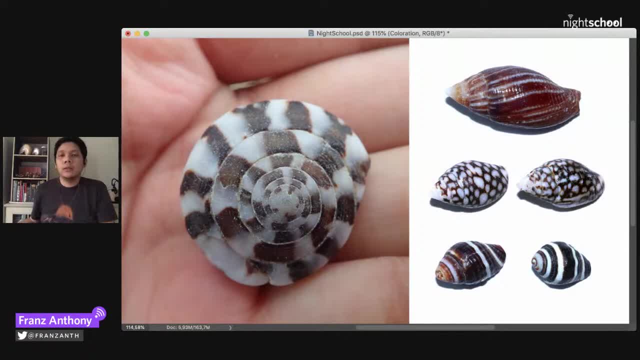 So bifals, clams and so on, And you can see here that snails can have fixed stripes like these ones They could have. as you can see here and here, their stripes can go both ways. It could be like horizontal or vertical. 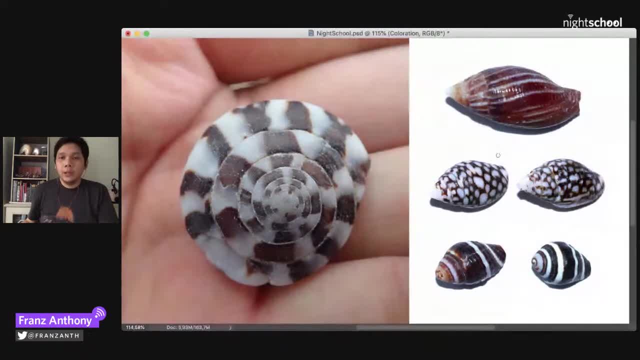 It could also be mottled like this. So there's a lot of possibility, because If you look at the chemical structure of a snail shell and a cephalopod shell, it's roughly more or less the same. So we could still bracket them together and apply this kind of coloration to our ammonite friend. 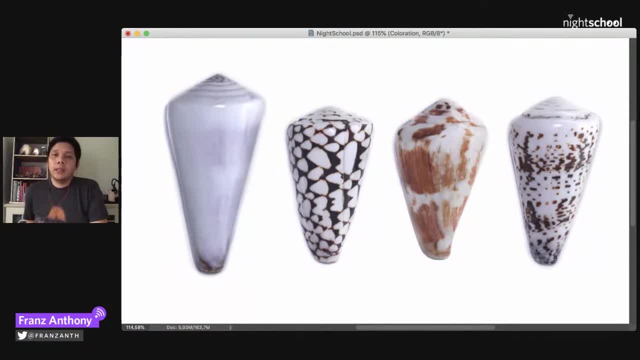 Another example is that these are conus shells, also known as cone shells. They are highly venomous, But if you look at cone shells, they are actually really diverse. You can see, on the left there's one that is more or less pure white with some subtle streaks in the middle. 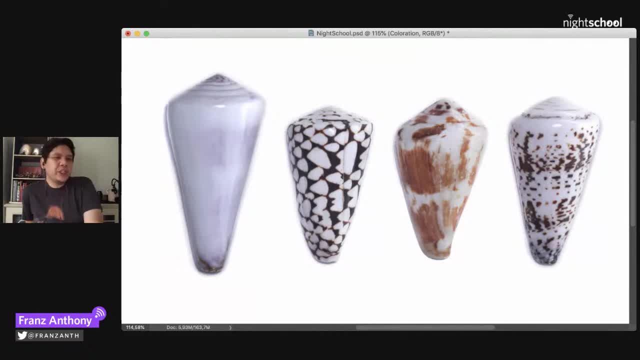 It doesn't really show here, but in real life it's a little bit purplish And you can also see there are also shells with triangular patterns, like the one in the second one here, And there are also shells with Kind of random patterns or maybe dots. 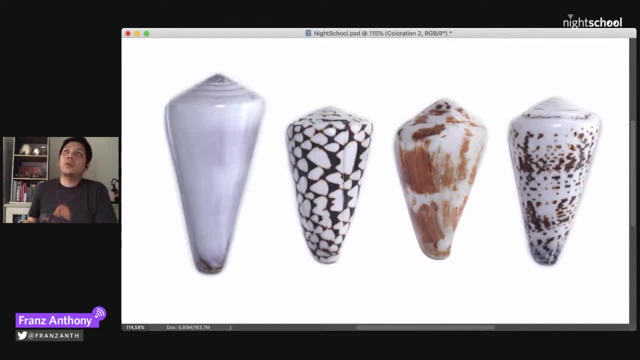 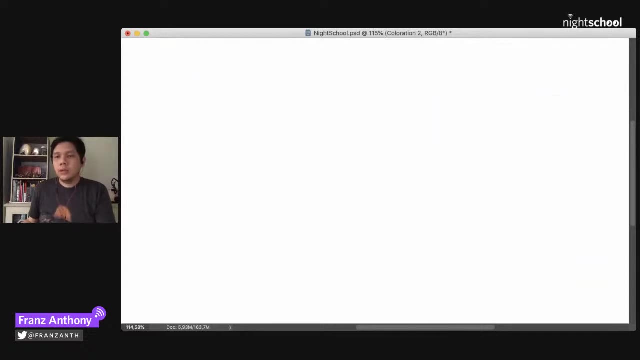 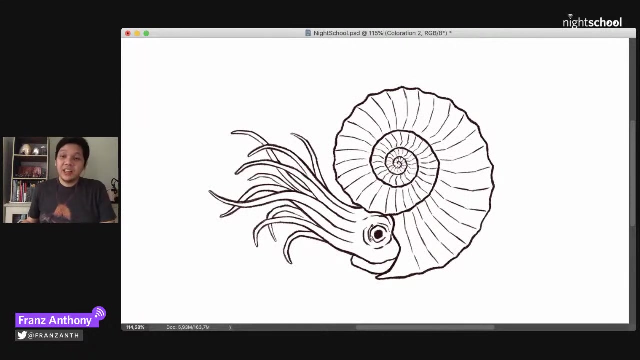 And these are all shells that belong to the genus conus. So even within closely related species, there's still a lot of variety that you can probably play with if you're an artist. So let's try to color these ammonites. I do not have much time here, so I cheated a little bit last night. 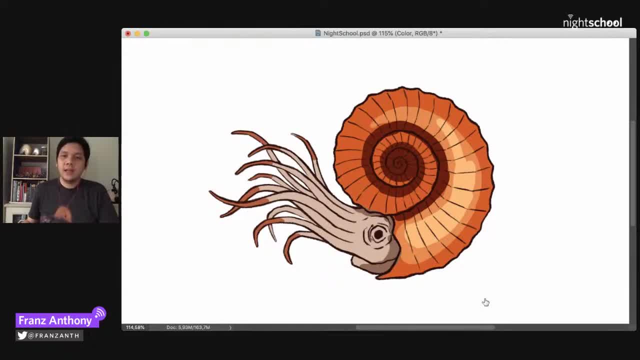 So I'm going to start by putting some basic colors So we could try to do a little bit of painting. Let's see how far I can go with this, But I think in the meantime if Lynn wants to join me and start asking questions or whatever, that's fine. 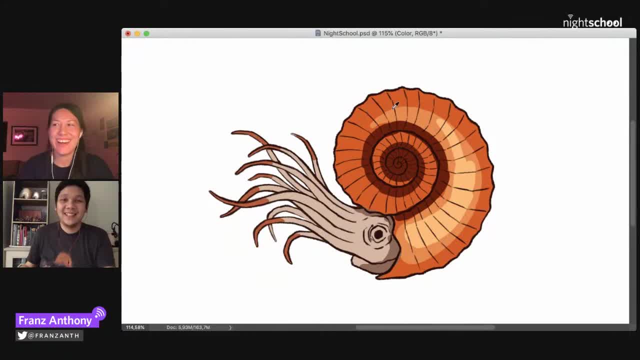 Hi, I'm here. Hi, Yeah, this is great, And I think Lynn and I are both cracking up during. your Is a Coconut, a Cat thing, Haha, Haha, That's such. I mean it kind of makes sense. 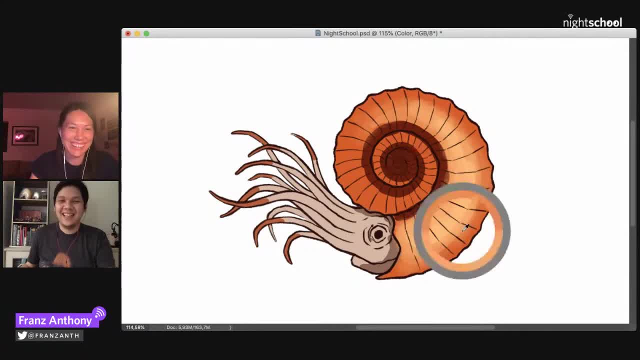 Yeah, furry outside, milky inside, Yeah. But yeah, it just does kind of go to show like how we obviously know what those two things are. So it's like what a silly question. But when you don't know, when you're dealing with stuff that's, you know, millions and millions of years old, you're not familiar. 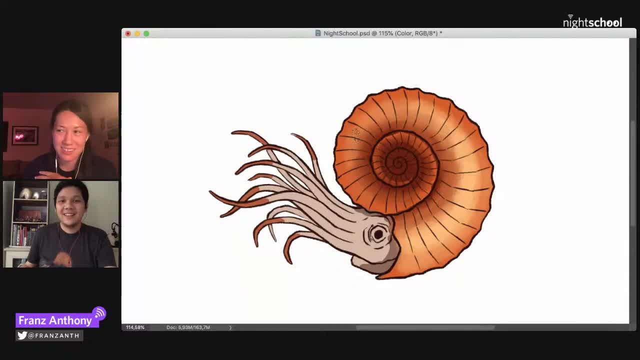 So that helped me understand what you're talking about. Yeah, Yeah, It's extreme, but yeah, that's the point. But yeah, I'm just. I'm just going to be here hanging out. If any of you watching have questions, I'll see them right away. 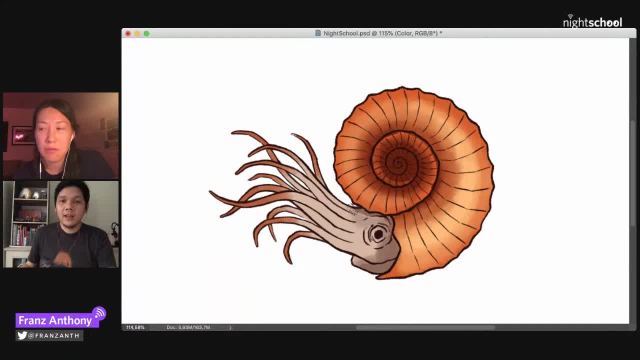 So you can go for it. But, yeah, And if you want to, I wouldn't be able to see the chat, So Lynn is probably going to be able to see the questions better. Yeah, Yeah, we'll be able to see them. 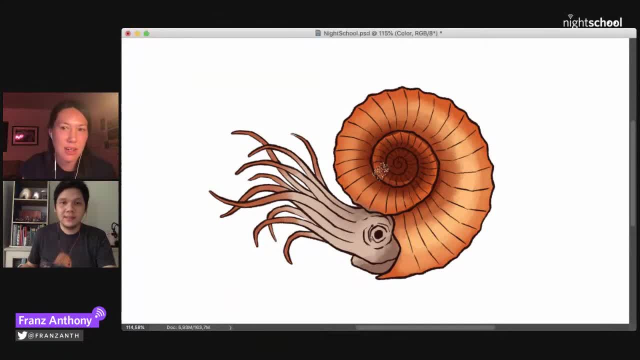 But this is such a specific type of illustration. I'm wondering just like how you got into it and how steep a learning curve it is. So I actually have been drawing animals since I was a kid, So I pretty much knew the general shapes of animals. 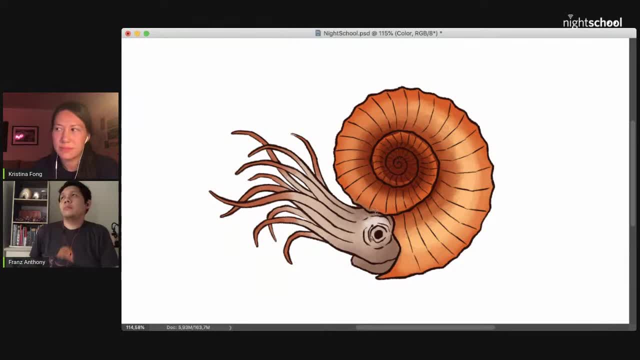 But I only started doing this seriously, maybe very seriously, Maybe five years ago or so. But I've been reading animal books, So I kind of know the technical terms here and there, which is kind of my saving grace, Because biology is kind of hard to get into if you're not an expert. 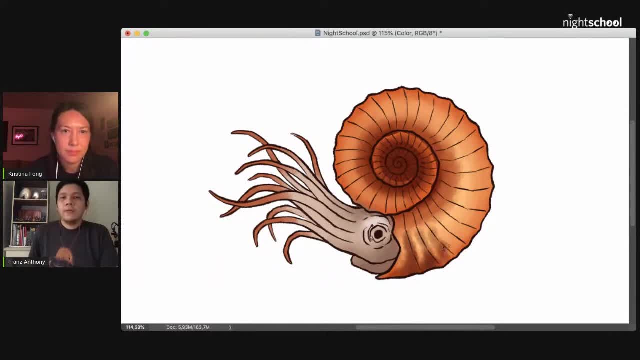 Because there are a lot of technical terms Like, for example, what the thing that people used to tell that ammonites are actually not closely related to the Nautilus is something like it's called the radula. It's something closer to like the tongue in our body. 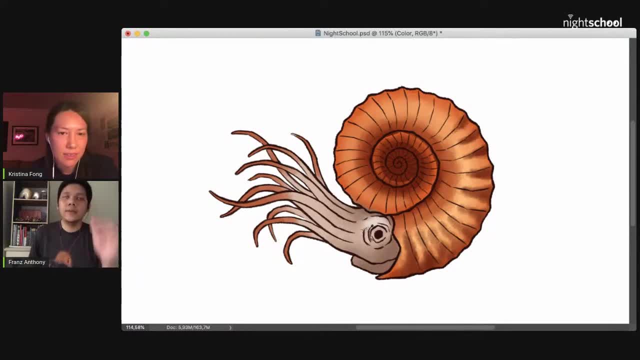 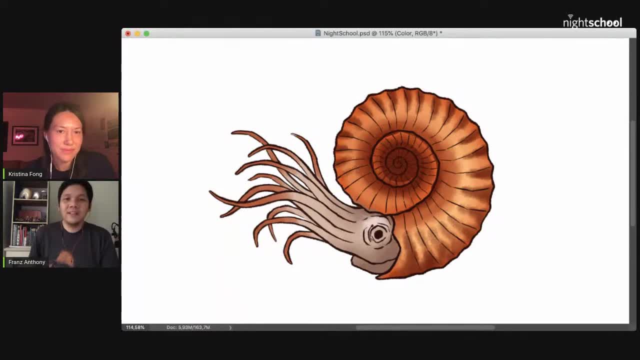 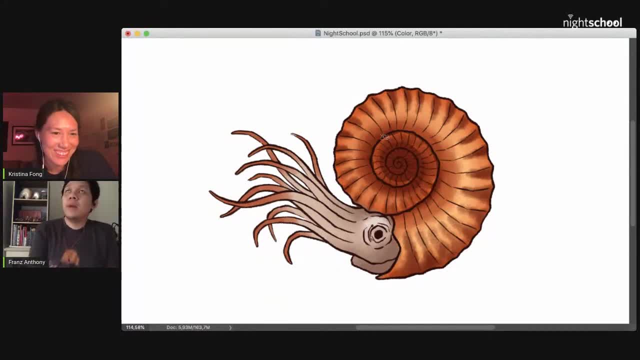 since they're so squishy, Right? I think Maricela said earlier that some things fossilize better than others, Because squishy things well, they usually decompose pretty quickly, They rot Or maybe they get eaten by other things like crabs and so on. 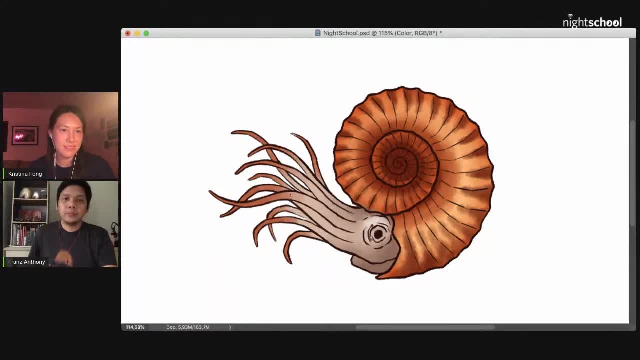 But there are actually really good fossils of squishier things like the worms. It actually depends on the site where the fossil is found, because there are fossil sites where really really good fossils of squishy things are preserved in such high details. You can actually see the filaments, the hairy parts of the body. 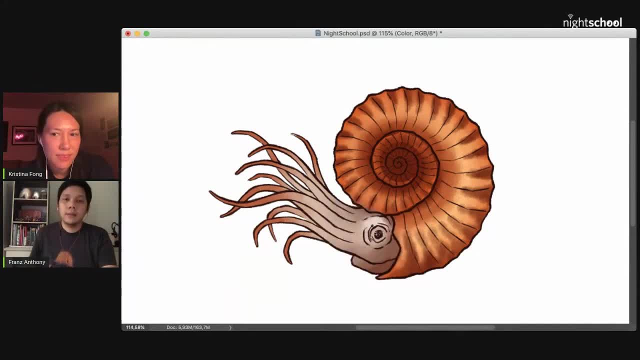 So there are fossils out there, Awesome, Oh, and what are you using to draw right now? Oh, I'm using Photoshop, which is my main thing. Are you using a tablet? Yeah, I'm using a tablet, Cool, Oh, this is interesting because you were talking about, yeah, working with scientific papers. 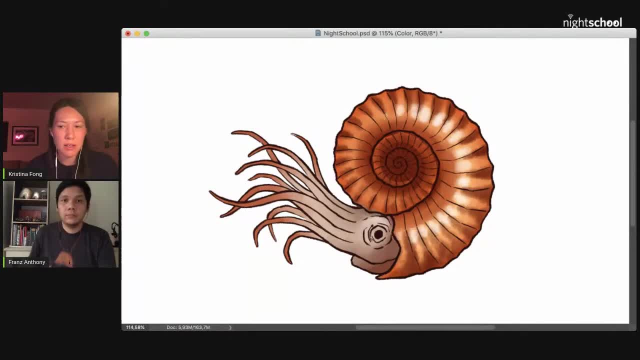 and learning how to read those And when you're doing work. somebody asked: how do you do that? How much feedback do scientists give? Do you ever feel a tug of war between scientific interpretations? Right, It actually depends on the artist, really, because I personally don't consider myself. 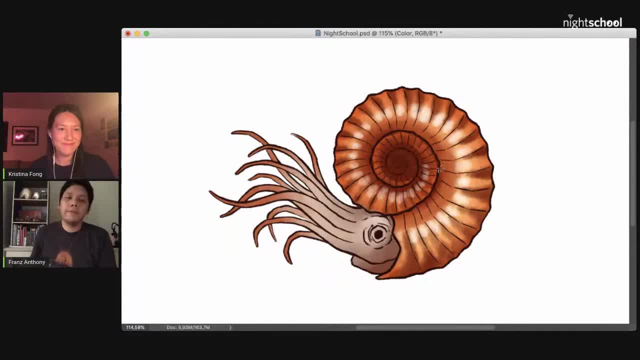 as a scientist. So I usually defer to the scientist and I kind of follow their advice pretty closely. But there are some artists who are also scientists and they might have their own opinion about things. So I'm not sure if that's correct, of course, because they actually handle fossils and so 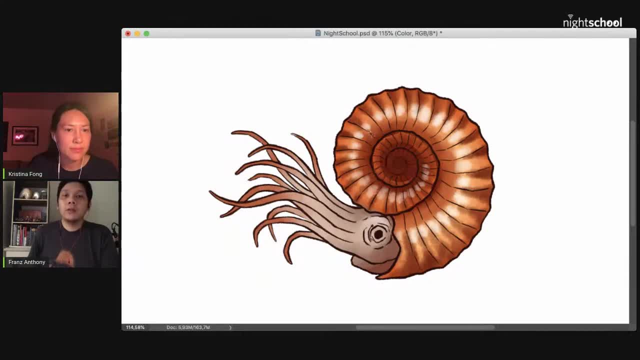 on, But since my background is actually graphic design and illustration, so I prefer not to comment too much on the accuracy and so on, because it's not my expertise and I know it. Yeah, yeah, Oh, this is good. This is related to trying to draw worms from. 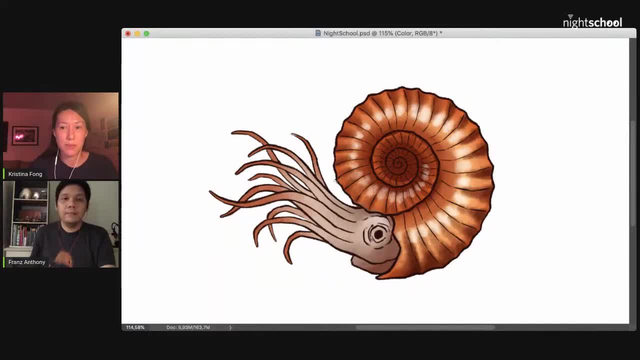 Oh yeah, So you were saying that they're fossils. but when you just see kind of a flattened fossil, how do you fill out its 3D shape? How do you figure out how it would look in three dimensions? Yeah, it's mostly about finding the right fossils, really, because when you look at 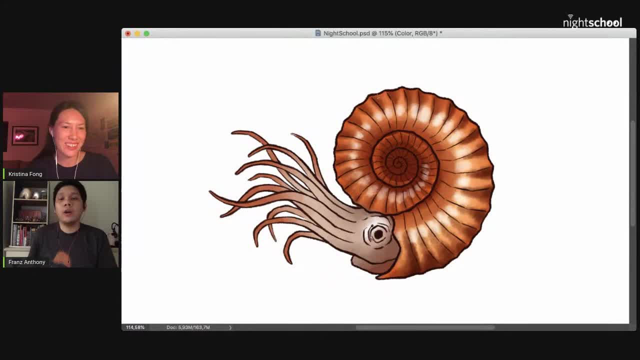 trilobites, for example. trilobites are pretty common in North America, I believe, right, Cockroaches in the ocean, Yeah, basically, Yeah, Yeah, And that some fossils are more common than others, and let's see if you have a lot. 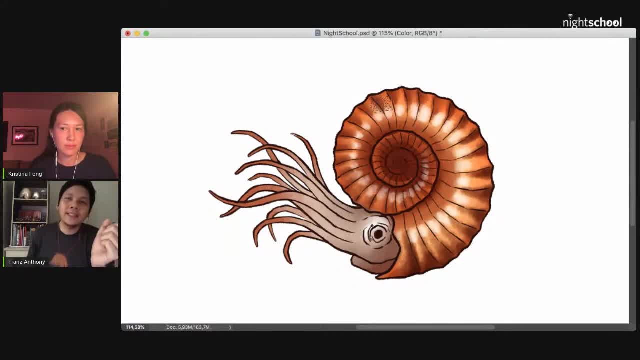 of little dead things. some of them are going to be dead, not in the same position, right? So it's a matter of finding fossils that look, Maybe are lying down side or something like that that shows you a different side of the. 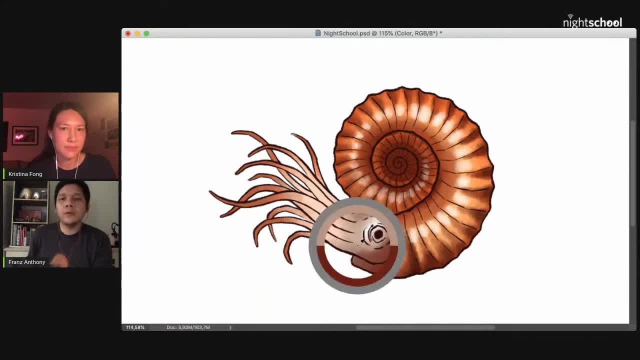 body, Mm-hmm. So, for example, I also work with fossil crabs, Oh yeah, And you can't really tell what they look like underneath, unless you found a fossil that is flipped upside down, or maybe the fossil is kind of sandwiched. the animal is. 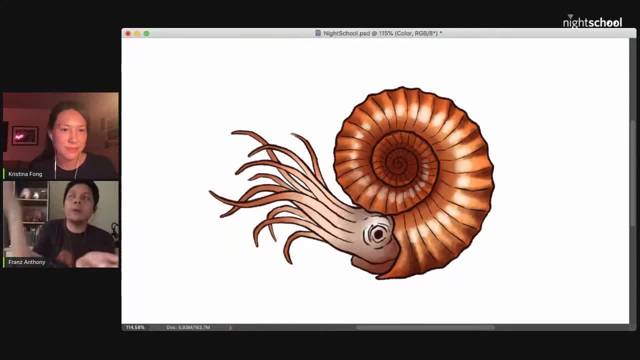 kind of sandwiched between plates so you can actually rip it open and see both sides of the crab, But otherwise sometimes you only see one part of it and sometimes there are just animals that you can't really reconstruct because you don't know much about it. 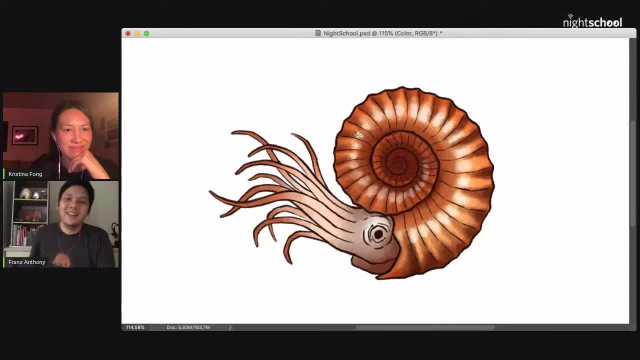 Yeah, You just have to keep up. Yeah, I was, yeah, I was interested in when you were talking about you were showing off Julio's art and about the different cat, like the different fur, like sometimes he depicts it as striped or spotted, and right now you're doing a kind of orangish. 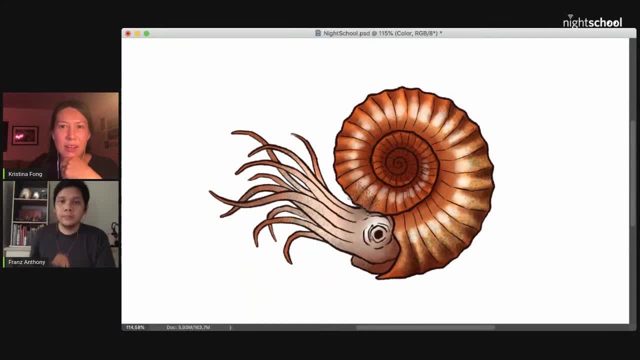 Yeah, So like how I know you talked a little bit about color, Yeah, I know you talked a little bit about color, but like, ultimately, how do you kind of decide whether to give something stripes or spots, and 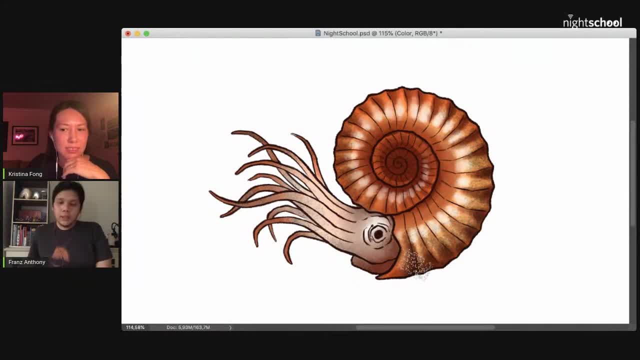 Right, what kind of pattern. So I know we talked about family relationships earlier and we know that a cat, for example, is not likely to have like false eyes, like on the tail of a peacock or a moth, for example. 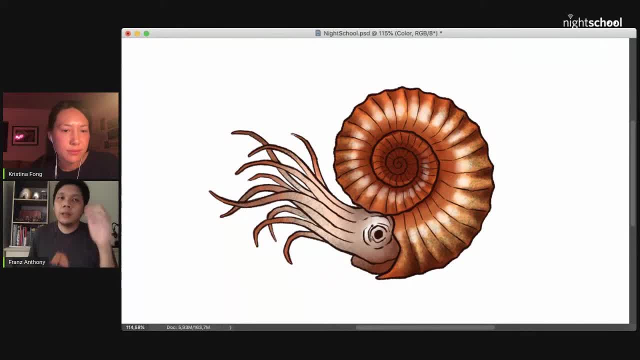 But so we know that it's more likely to be spotted or maybe striped. Yeah, So maybe in terms of like, if I have to like have a Bolsonaro, like cat or something, I know that it's easier to keep it around. 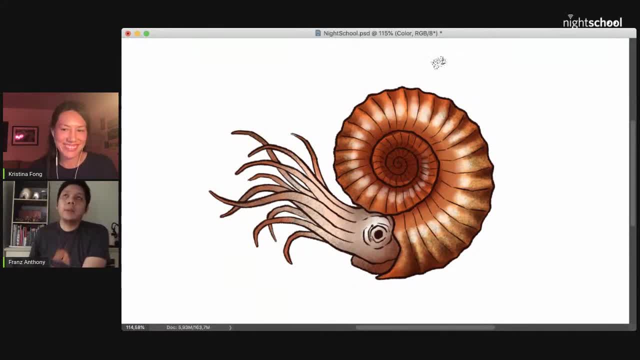 I don't know, Yeah, Uh Like, I think that you just needed to. Well, Yeah, immediately you're making a difference, right, Yeah, in terms of like, when I first came like a lot of my life, I always was you. 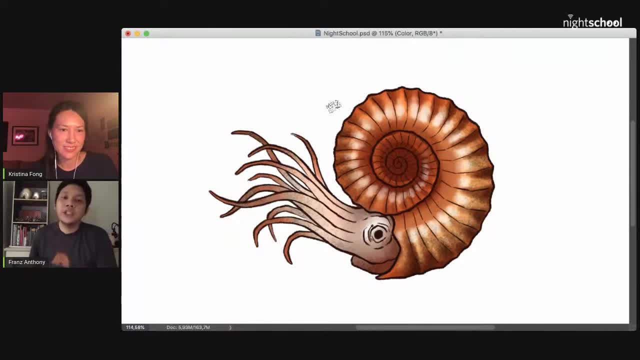 know a bit more like positive, Because Yeah, Yeah, Yeah, You know, I think that, like, what I like to do is kind of like give a little little bit of a compare, Mm-hmm. 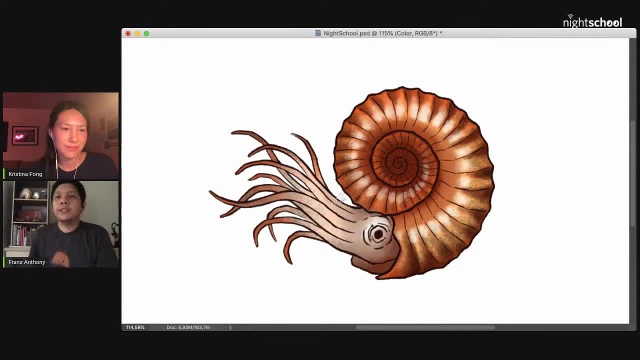 I mean like I was working at you know after University for a couple of years. I, If you compare that to fish that live in the coral reefs, for example, the coral reefs is really vibrant and colorful, So a fish who lives there can be colorful and still go undetected by predators. 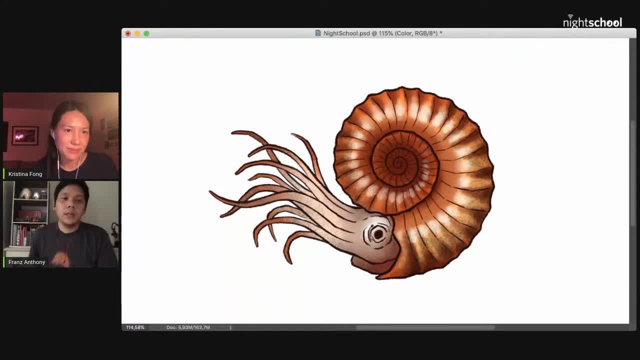 So there's a lot of ecology that plays out when I look at, when I decide colors, But also sometimes there are fossils that you don't even know where it was found. It was just one fossil. You don't know what kind of other animals live in it. 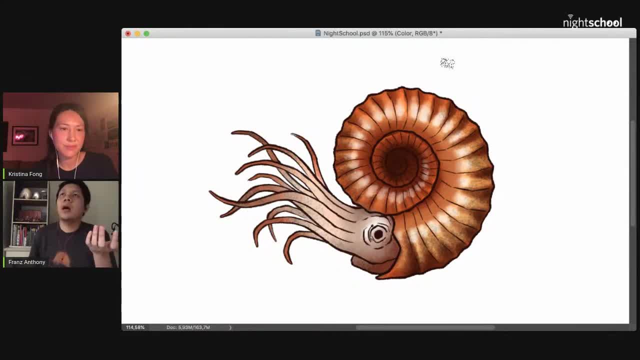 So let's say you found a fish and you found a fossil anemone next to it. So you know it's probably going to live somewhere in the coral reef, maybe. But if you found a fish that is just there alone, you can't really tell where it lives. 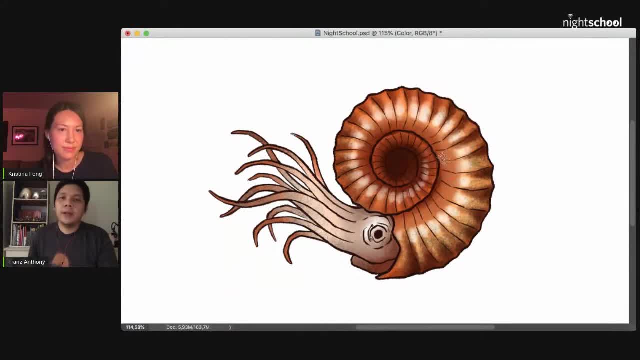 So you kind of sometimes you just have to decide what looks attractive To the viewers, But also you have to make it more or less reasonable. Yeah, no, polka dotted. Yeah, no, polka dotted. Is anything polka dotted? 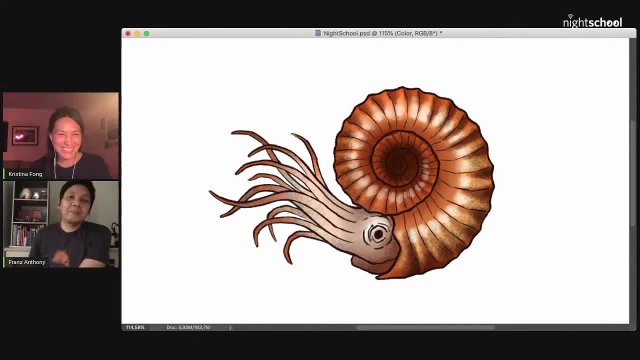 I guess there are shells that are polka dotted. Yeah, actually it's funny because different animals seem to have different color patterns. Maybe it's- I believe it's something it's tied to their chemical structure or something like that. But we see that maybe shells or even fish can be polka dotted. 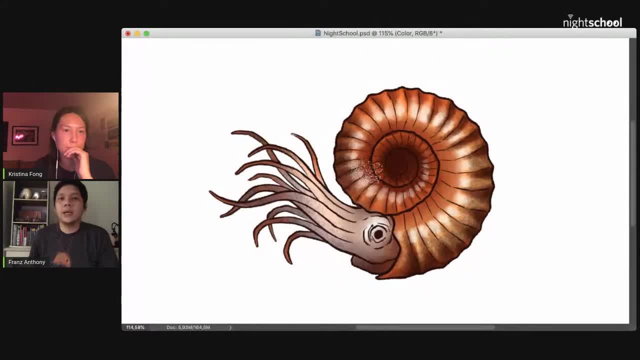 Or maybe some fish can have really, really complex patterns, But mammals don't usually have them. But also it's because mammals are mostly more or less color blind, Because I believe mammals evolve at night, when dinosaurs roam the day. So mammals are usually a little bit more drab compared to invertebrates or birds. 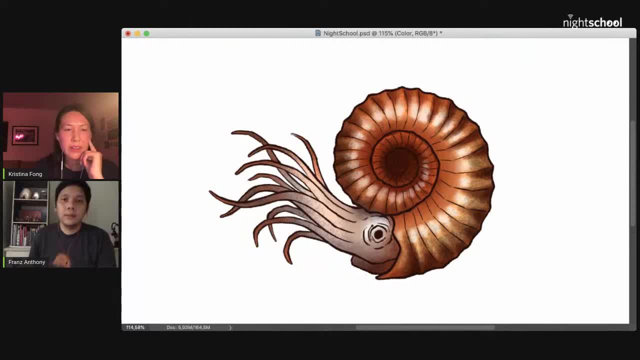 Hmm, There's been a lot of mentions of Animal Crossing in the comments. Are you getting lots of people asking: do you collect fossils in Animal Crossing And what do you think of their animations? A little critique, Yeah, Let's hear it. 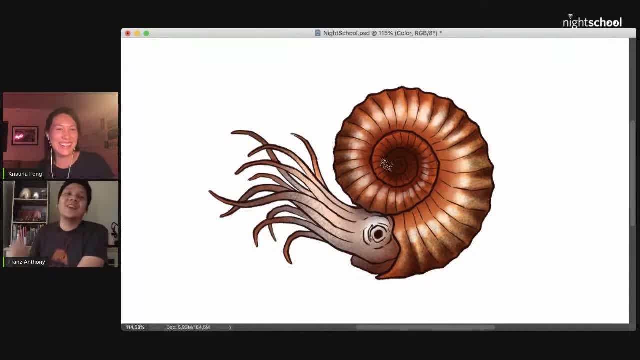 Oh my, I'm a heavy Animal Crossing player And if you look at my play time it's just astronomical. But yeah, I think It's pretty well done for a mainstream game that is not really focused on paleontology, Because a lot of the depictions are pretty up to date. 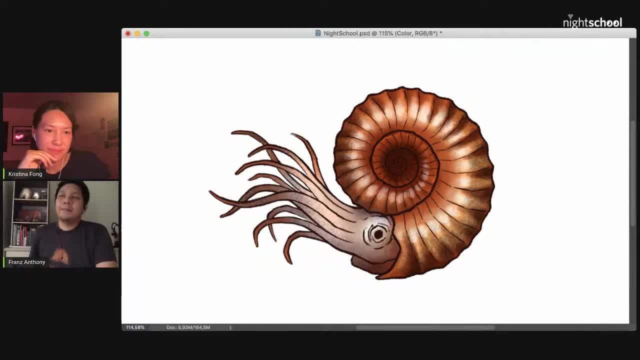 Even though there's a funny thing that happened a while ago Is that Spinosaurus just got a new tail. There's a new tail of the body. A new fossil tail was found a while ago And it happened just after the game's launch. 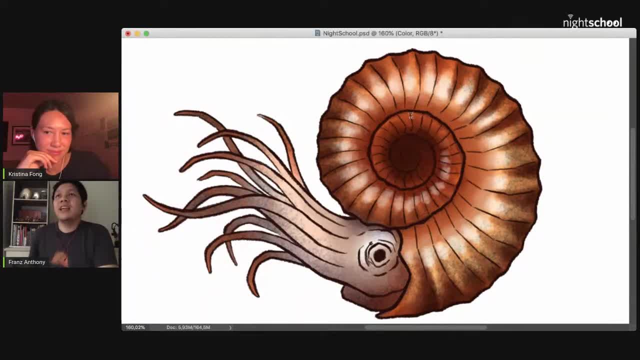 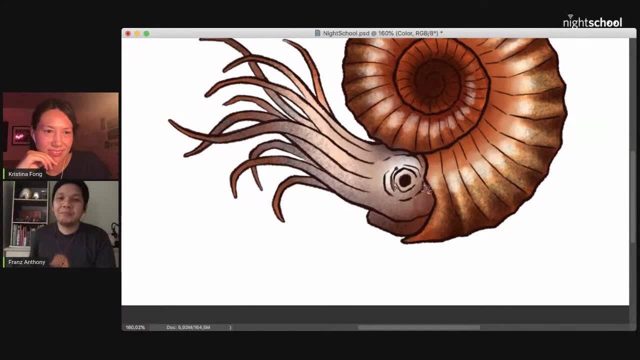 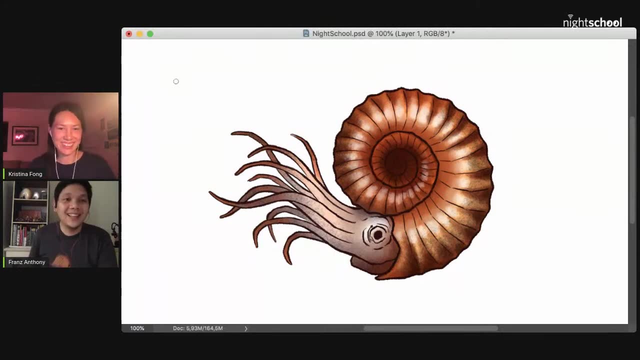 So the game- The fossil in the game- was technically inaccurate Just weeks after it launched Because a new fossil came out. So the tail When we think of Spinosaurus- Sorry, I don't draw dinosaurs often, But So the head shape like crocodile, like this. 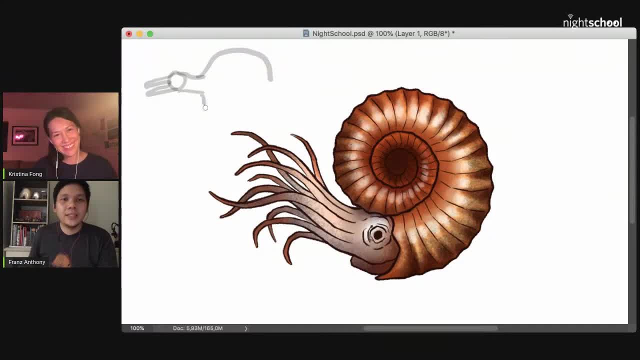 And we see it has like bump on the back, Spine on the back And the tail. Most people would depict it something like this, But I believe the new tail was something more like a fish, Something like this, But I forgot the details. 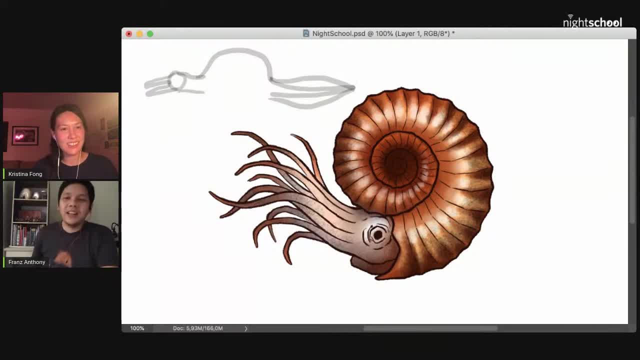 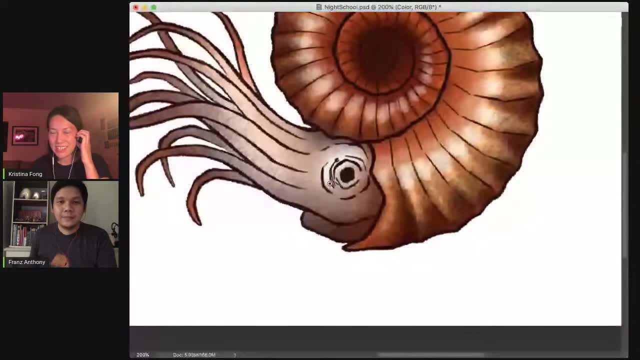 It's pretty new. It just came out this year. It's pretty funny To watch people talk about it online. Yeah, Yeah, it was actually fun. Like a while ago, We did a little Instagram story series with Maricela. 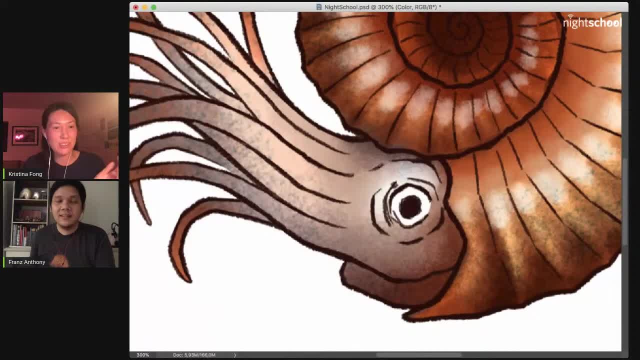 And she was talking about. She showed us fossils from the academy's collection That Pokemon were inspired by, And so like that was like she showed the Pokemon next to the fossils And I was like, oh yeah, That's really nice. 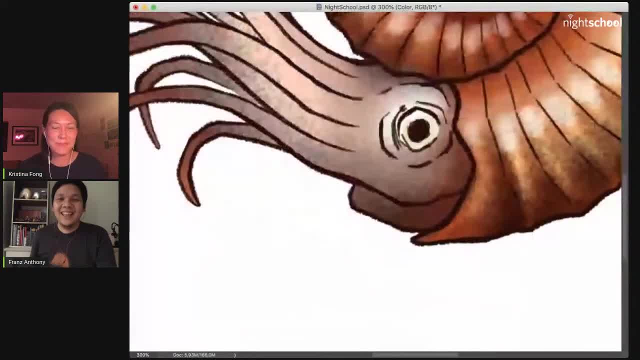 Yeah, They're paying a lot of attention. So, Yeah, That's one way to get people's attention. Yeah, Yeah, But I think that's why paleo art is really important, in my opinion, Because it shapes. We know that scientists talk to each other a lot. 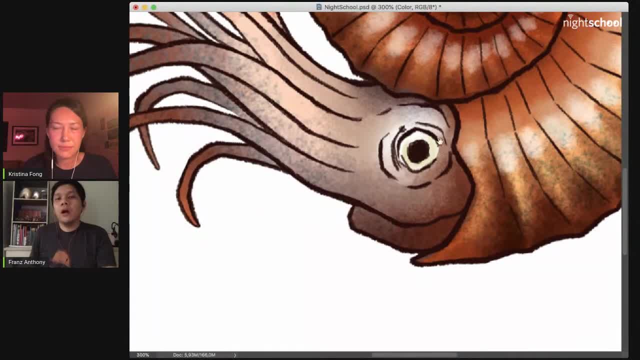 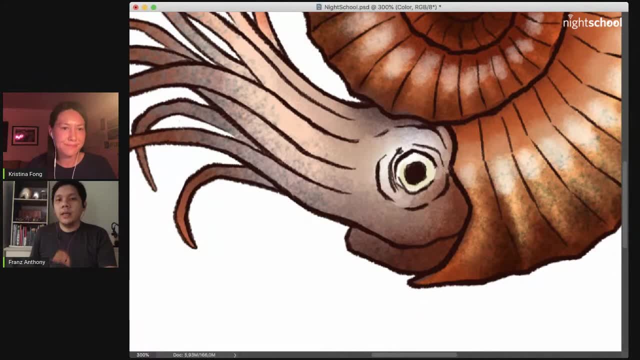 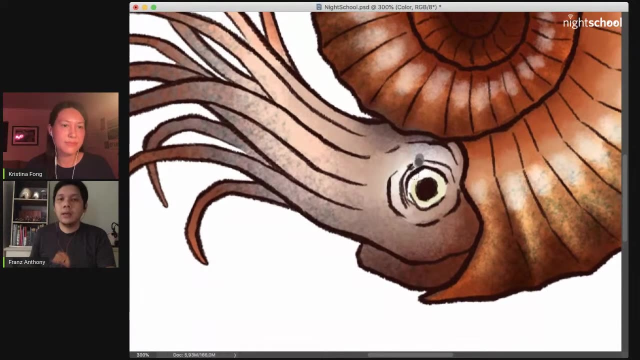 In like conferences And so on, But a lot of that information don't really actually make it to the public. So Pop culture and art in general like this is what actually shapes the public's opinion And what they think animals look like. 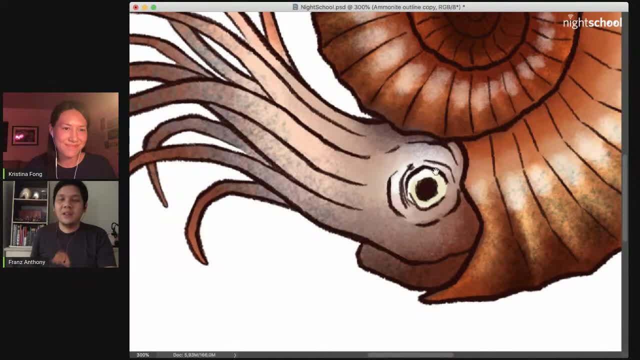 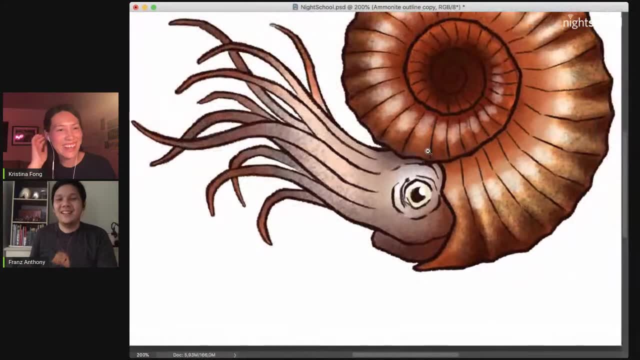 So that's actually our job: to make it look, To make animals look presentable, but also, I guess, reasonable, Yeah, And I think that's one way to just spark people's interest in science too. Yeah, With something I mean like this: 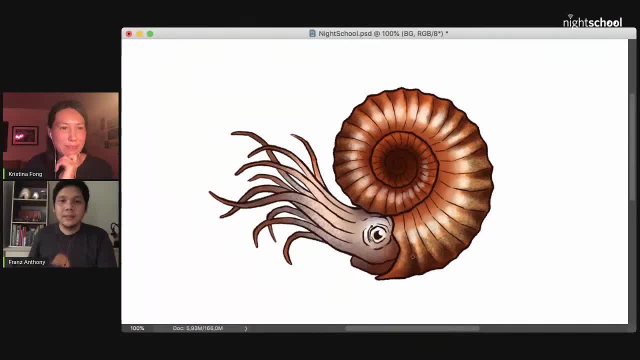 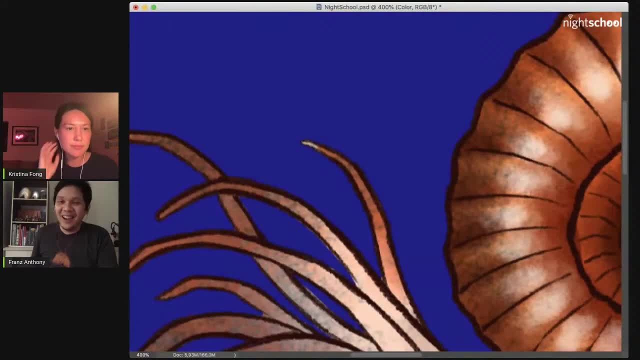 This looks amazing after What we've been. you've been coloring for 10 minutes. Yeah, Because I. What usually takes longest for me is deciding what color I want to use. Okay, So I kind of cheated a little bit last night and just pick some color already. 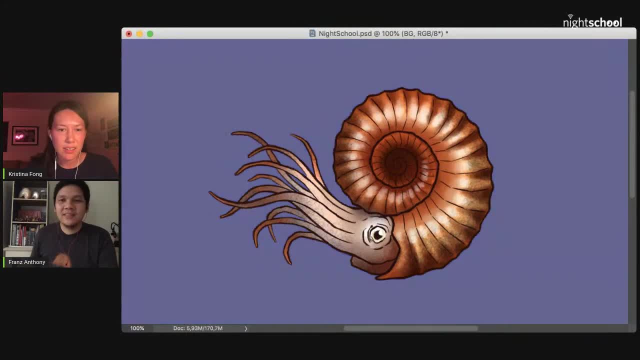 Mm-hmm, Yeah, So is it. Is it kind of close to Close, to finish? No, Or what would you? We could probably call it finished, because otherwise I would keep tweaking this for a whole day. Somebody asked- and this is always just a fun question- 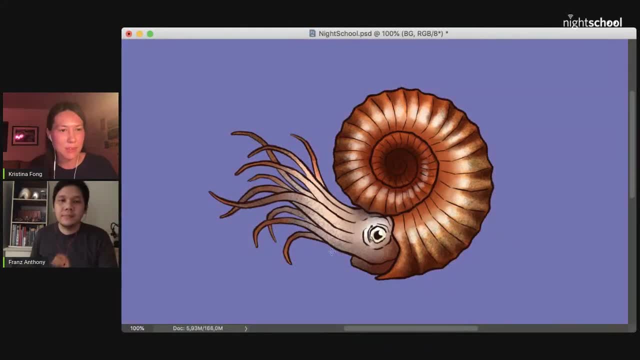 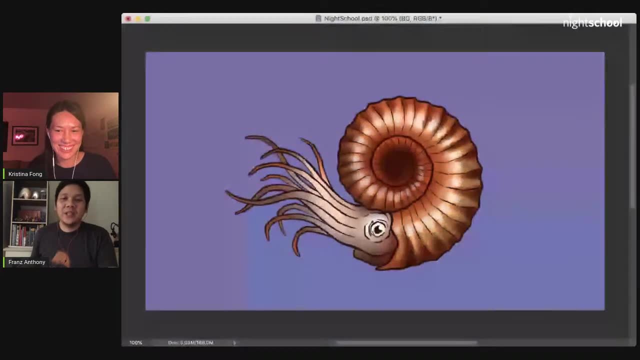 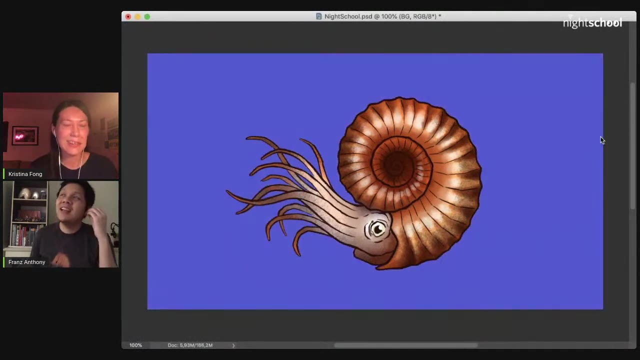 Like: what's your very favorite animal to draw? I know you like the Nautilus with its cool hood, but what else? That is a difficult question. I've been drawing a lot of crabs lately. Okay, Yeah, Mostly because people don't think about crustaceans a lot, but they actually have a lot of funny little parts. 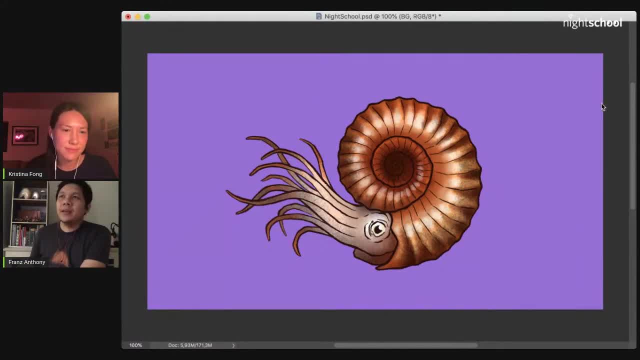 Like their body shapes can be. you know that the crabs we see on a daily basis are more like the emoji crabs- right Yeah, But there are also crabs that look like Dorito: The body is just a triangle and it had like tiny arms on the side. 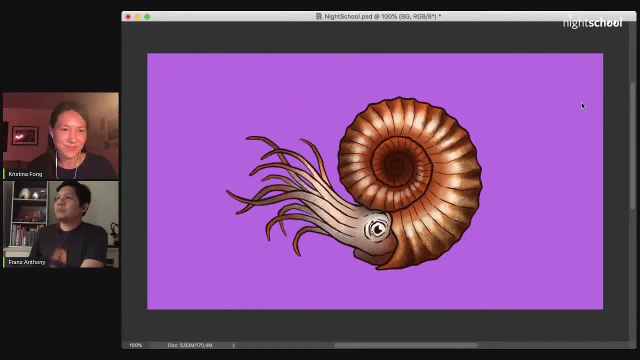 Yeah, And there are also crabs with a really really long elbows, So it looks something closer. Let's say: this is the body, So the claws are like this, So it's the crab is mostly elbow. It's not something that most people will think about when they 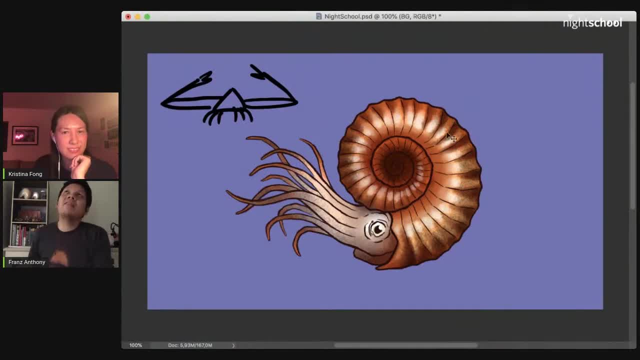 When they say crabs, because they're really diverse and kind of underappreciated. I think Nice, Is it a chip or a crab? How will we ever know Crab and chips, I guess? Yeah, Well, thank you so much. 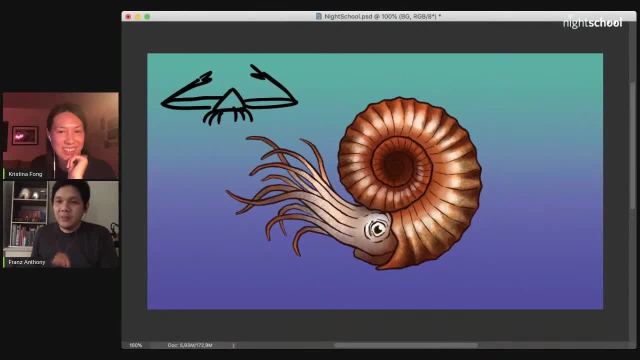 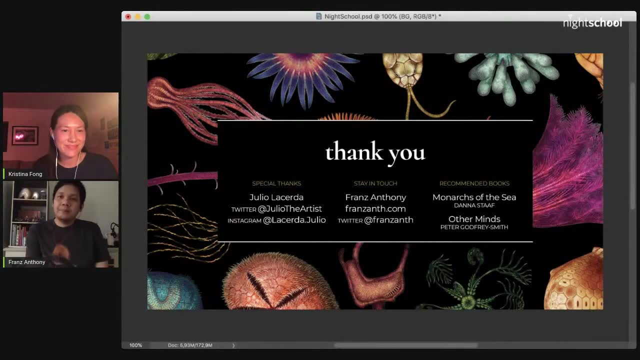 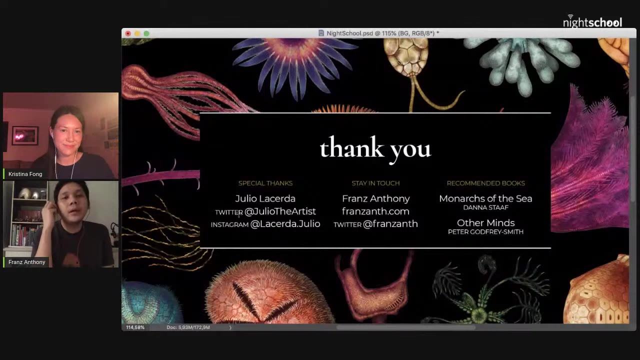 This is really interesting and fun to see. No problem, This creature come to life. Yeah, Yeah, Thank you for having me. Yeah, And I would like to thank my friend Julio for lending me his images. You can follow him on his social media here. 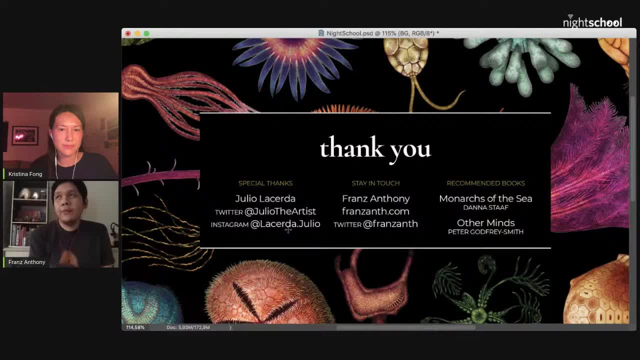 I showed the links on the screen And if you would like to read more about the history of cephalopods, cephalopods have been around for over 400 million years, So they have a much longer history than dinosaurs, So I recommend you to read Dynastaff's Monarchs of the Sea. 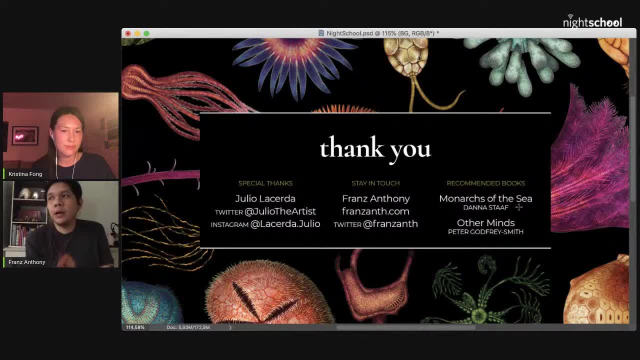 And if you want to read more about their behavior and so on, there's a book called Other Minds. that's really really good. I just finished it- Awesome. Well, thank you so much. Check out all those links And I'm going to say goodbye to Franz and bring Lynn back on the screen. 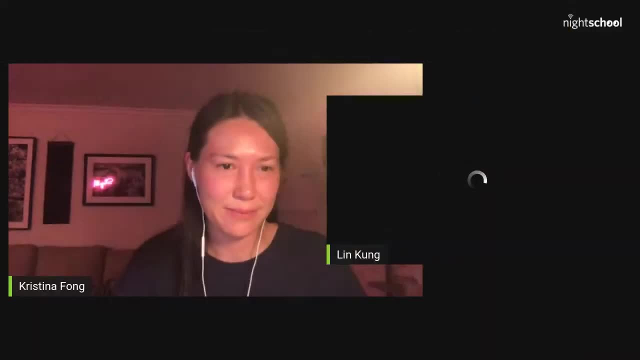 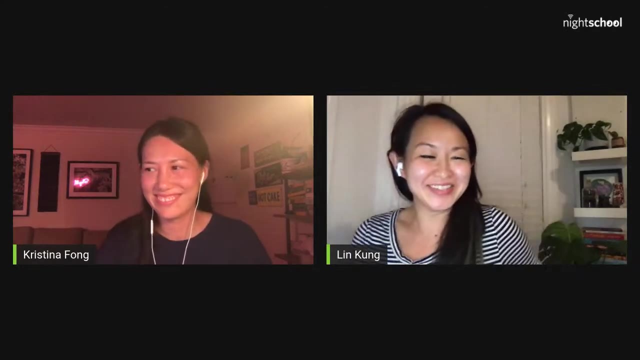 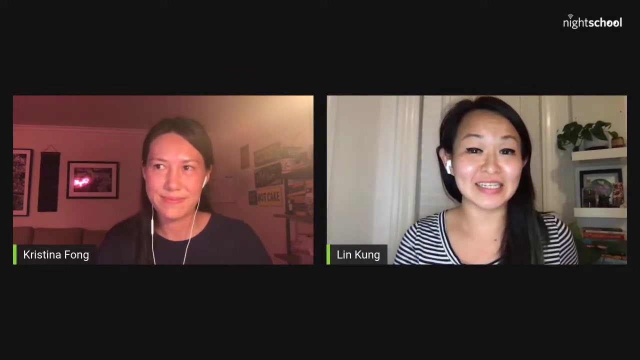 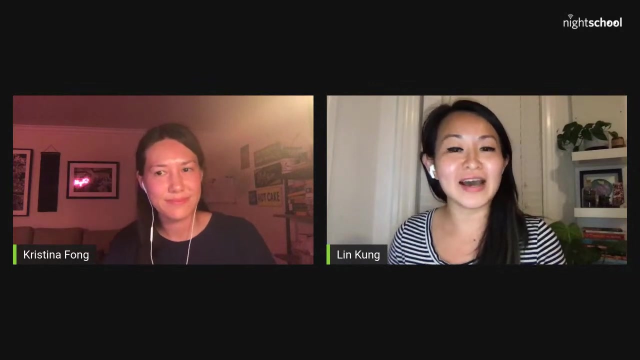 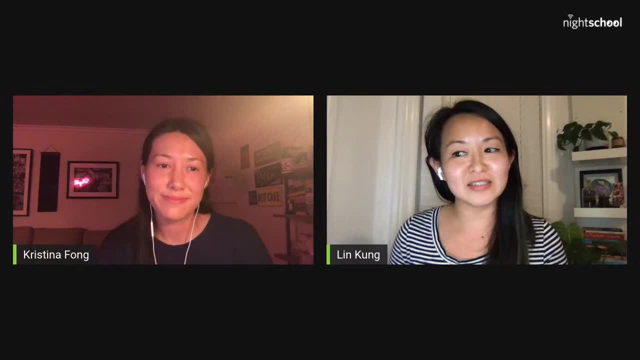 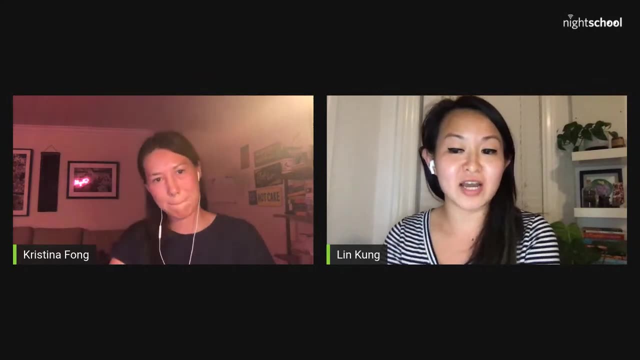 Next week it's our Halloween special. Get ready for a night of science, death and drag. We're talking alligator carcasses and zombie worms, Jumping spiders, Sookie. tales from a blackwater photographer who will take over hosting Moody's. 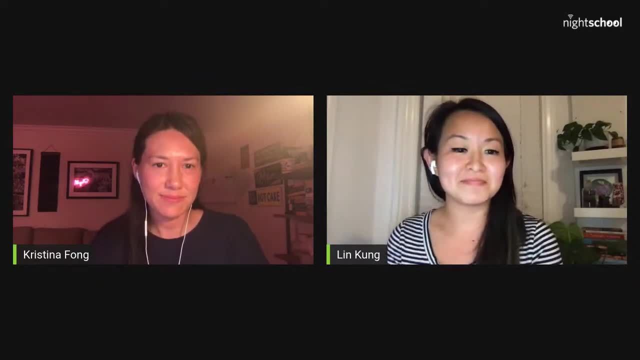 with some terrifyingly entertaining performances. And, in case you haven't heard already, the Academy is actually reopening to the public tomorrow. It's been seven months And we just wanted to thank you so much to all the people who are tuning in for the first time. 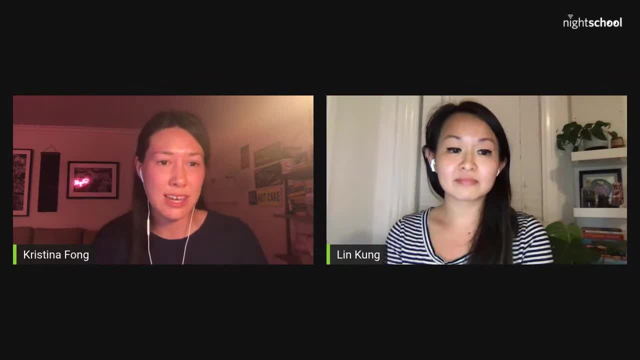 for the members, the donors, for supporting us all this time. We're so. we wouldn't be getting to tomorrow without you. Nightlife is not returning just yet, but we will definitely let you know as soon as we do. We're eager to see you. 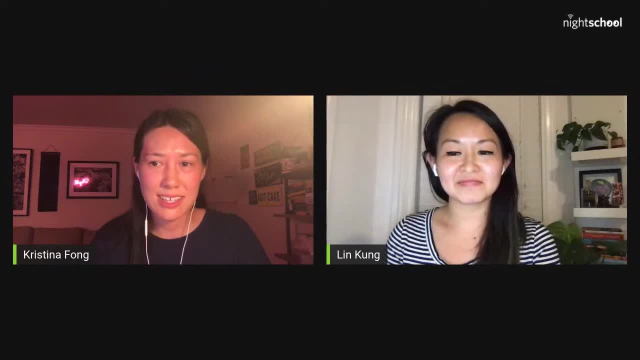 Until then, thank you so much and have a good night. Good night.